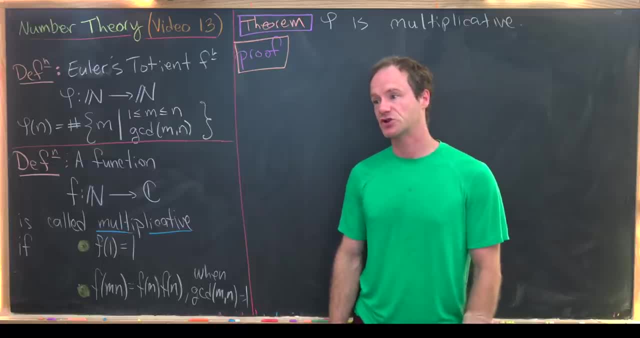 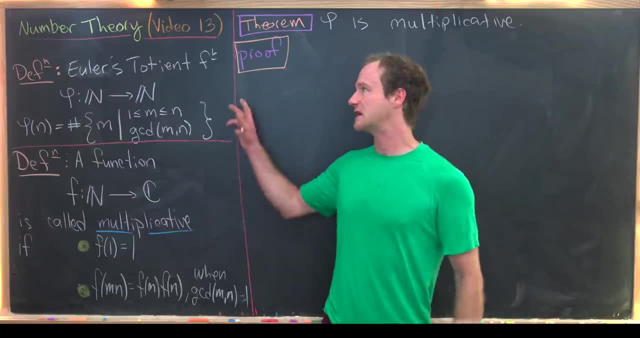 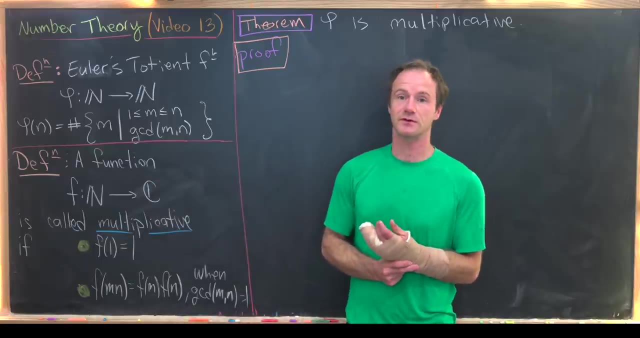 prove some things about Euler's totient function and come up with a nice strategy for finding values of this function. Okay, so let's begin by recalling that Euler's totient function, phi, goes from natural numbers to natural numbers and it's defined by: phi of n is equal to the number. 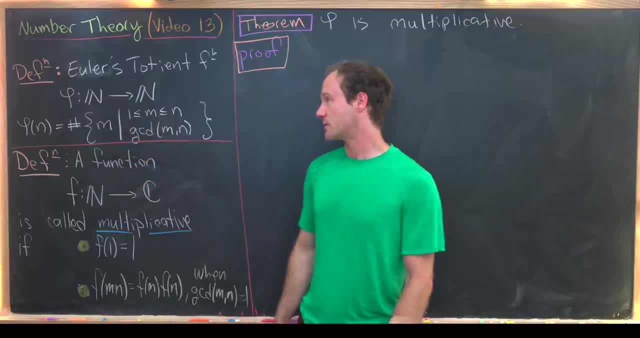 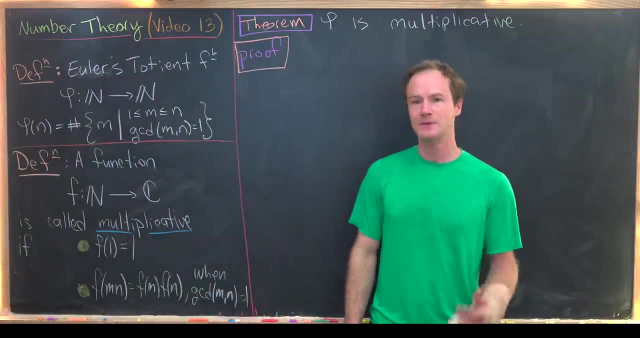 of elements in the following set. So these are natural numbers between 1 and n that are relatively prime. Okay, so we did several examples in the last video of evaluating Euler's totient function at some numbers, and we'll do some more at the end of this video once we have a nice formula for this. 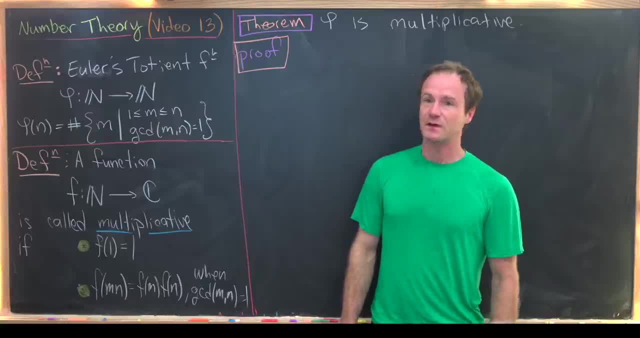 function. Okay, so the first thing that we want to prove is that phi is indeed something called a multiplicative function. But let's look at the definition of that first. A function f- from natural numbers to complex numbers- is equal to the number of elements in the following set. 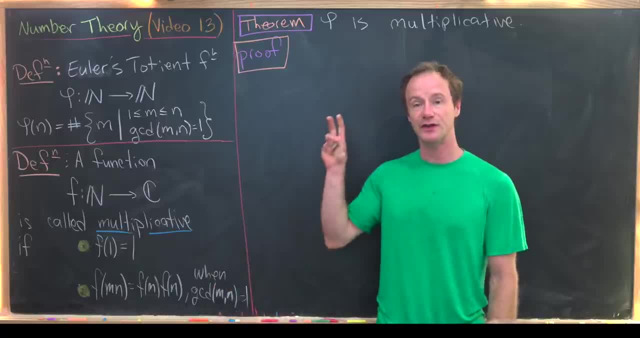 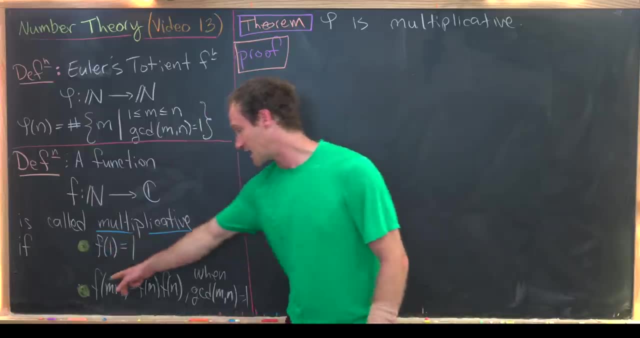 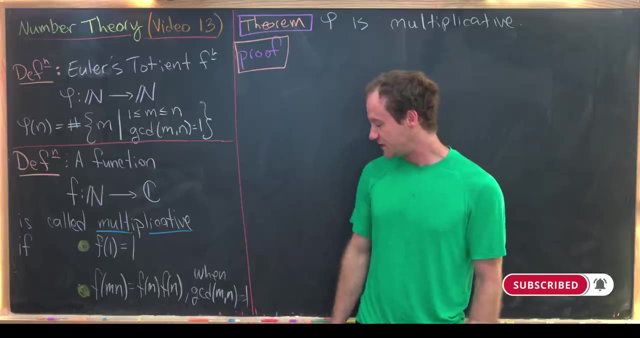 The first is that f evaluated at 1 is 1, and the second is that f evaluated at m times n is equal to f of m times f of n when the gcd of m and n is 1.. So if the gcd is not 1, then all bets are off. 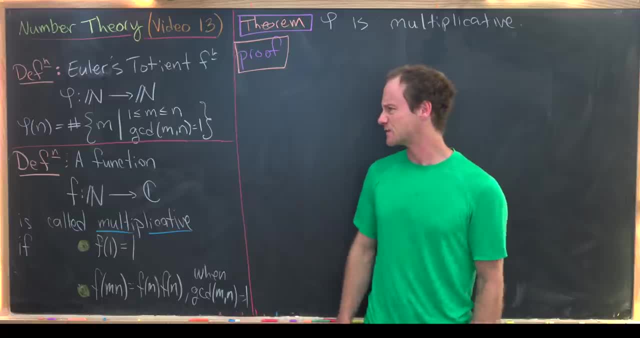 You may not have this property, And I think this is like some sort of number theoretic definition of a multiplicative function. If you know something about abstract algebra, ring theory or something like that, then this may seem like a little bit more restrictive. But let's just 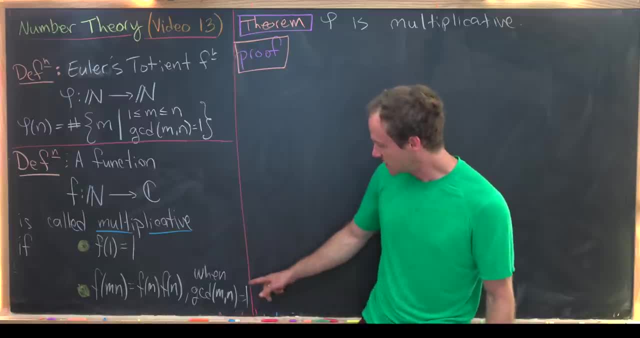 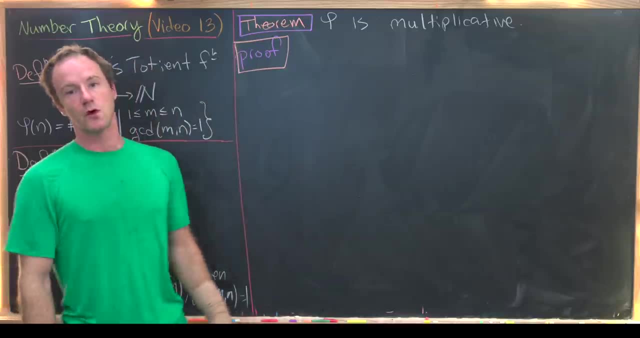 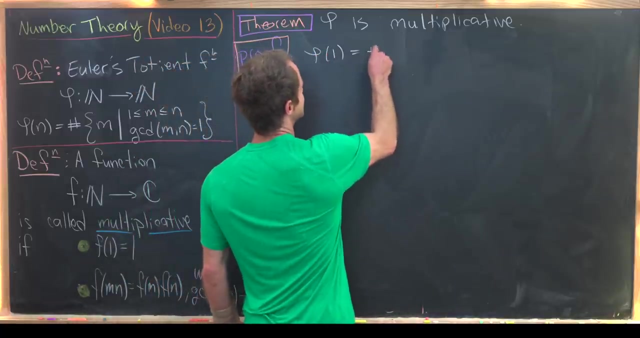 keep the context of this being a number theory class. So we need this second condition here. That's important, Okay. so let's get going on this proof. We'll start by proving that the first condition holds, but that's pretty easy. Notice that phi of 1 is the number of elements in the 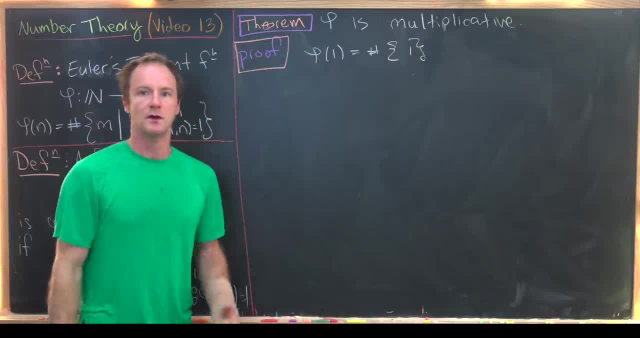 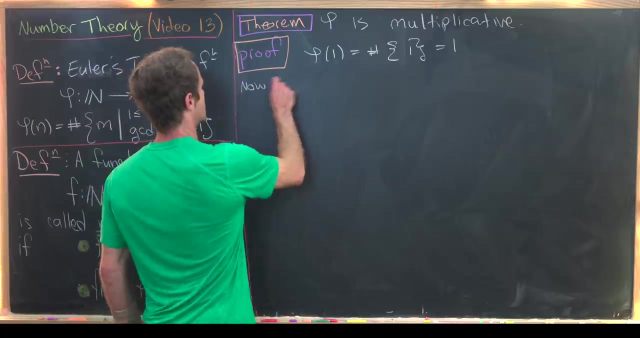 set containing just 1.. Well, why is that? Well, 1 is the only number between 1 and 1 that has gcd of 1 with 1.. So we're pretty good to go there. This is equal to 1.. Okay, so now we want to suppose that. 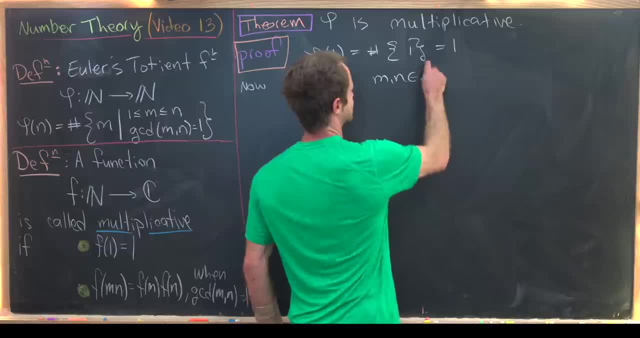 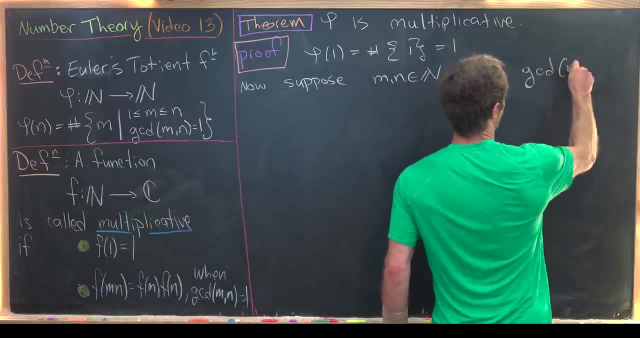 we've got a pair of relatively prime natural numbers, So I'll call them m and n. And, like I said, they're relatively prime, So I'll call them m and n. And, like I said, they're relatively prime, So I'll call them m and n. And, like I said, they're relatively prime, So I'll call them. 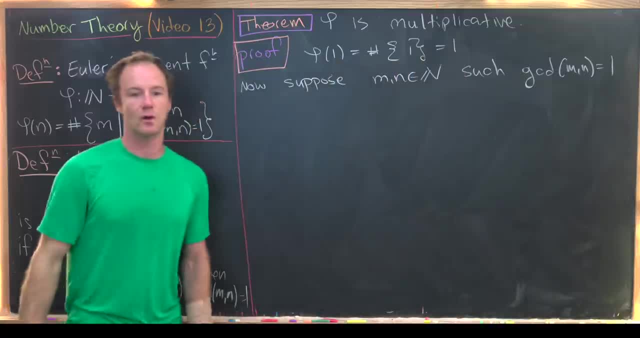 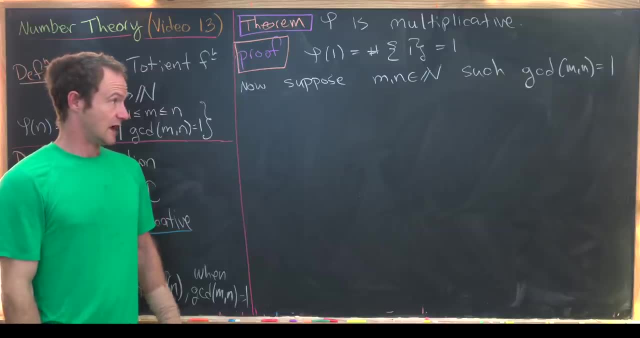 prime, Or in other words their gcd is equal to 1.. And now let's recall: in the last video we had the notion of a reduced residue system And we're going to want to use that notion for these two numbers, m and n. So let's bring two reduced residue systems into existence. 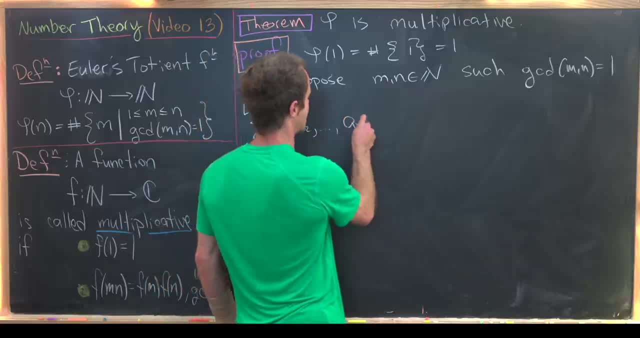 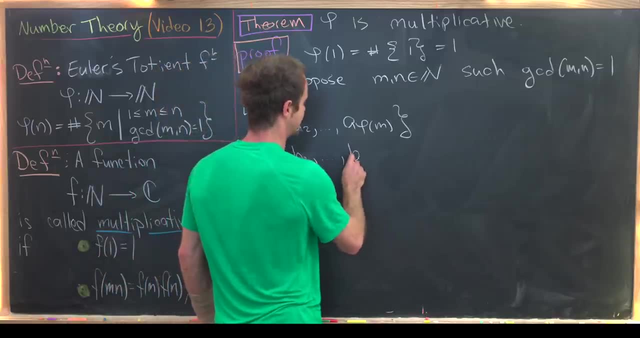 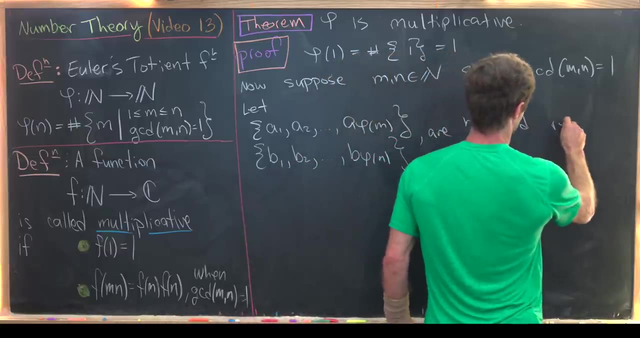 So a1, a2, all the way up to a phi of m, And then b1, b2, all the way up to a phi of m, And then b1, b2, all the way up to b phi of n. So these are reduced residue systems. 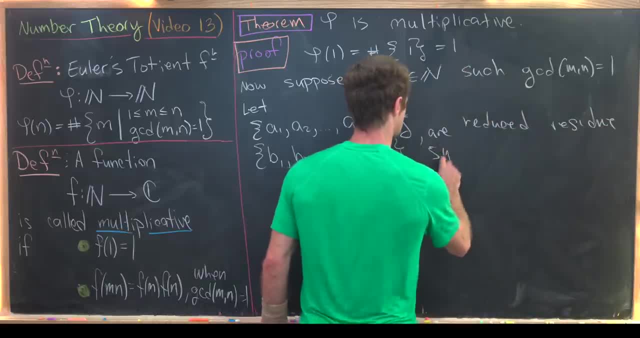 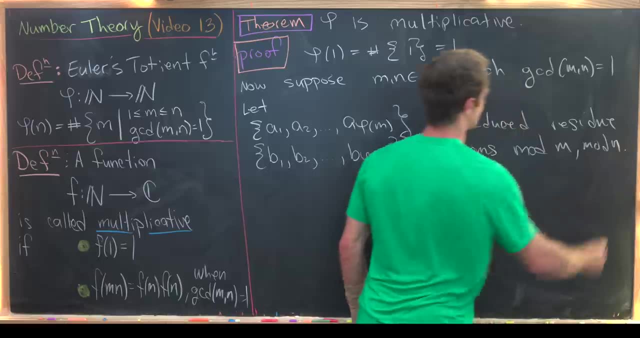 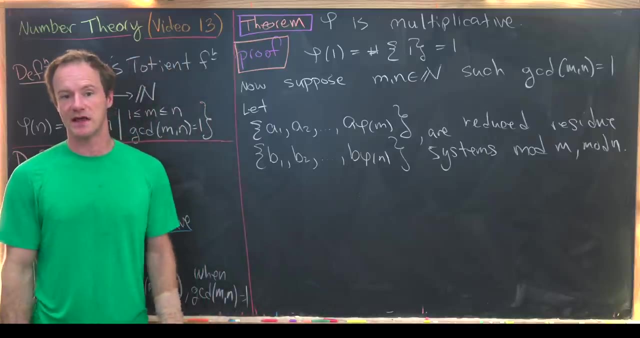 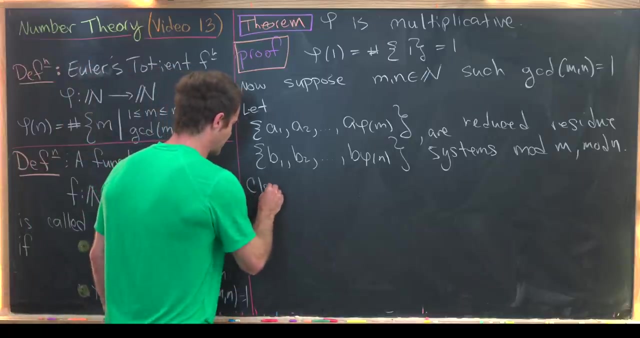 mod m or mod n, kind of as the context dictates. So obviously, this first one is going to be a reduced residue system, mod m, And this second one is a reduced residue system modulo n. And now we're going to prove the following claim, And this following claim will actually: 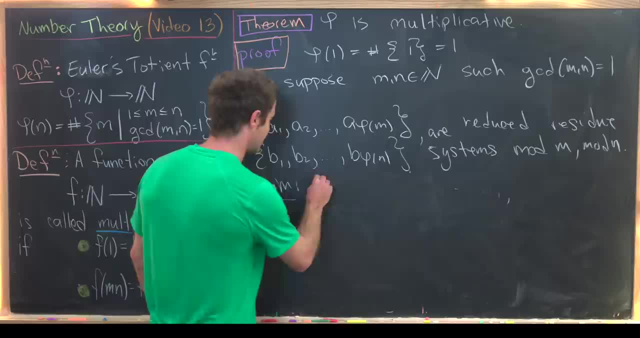 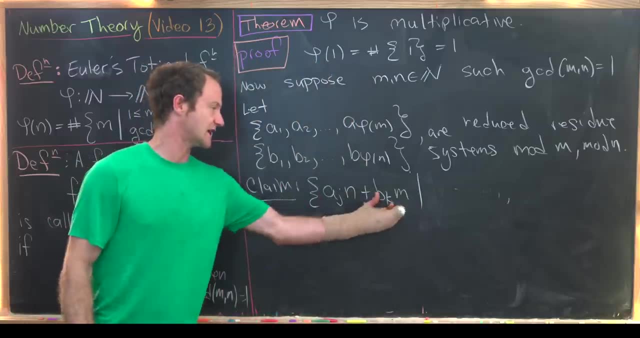 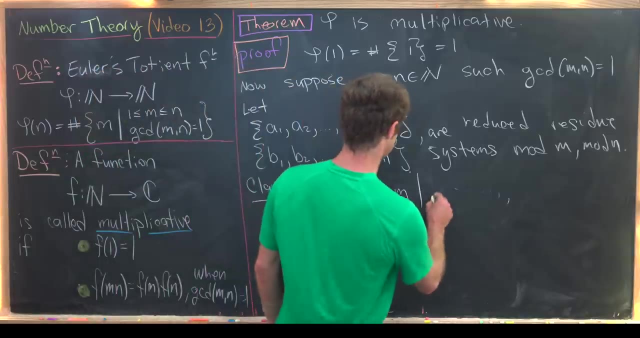 pretty much finish this proof off. So the set of linear combinations a, j, n plus b, k, m, as j and k run over the appropriate indexing sets, so we get everything from these two sets. So let's see, That means j must go between 1 and. 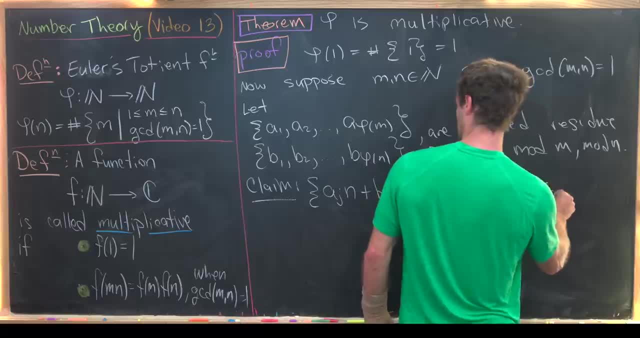 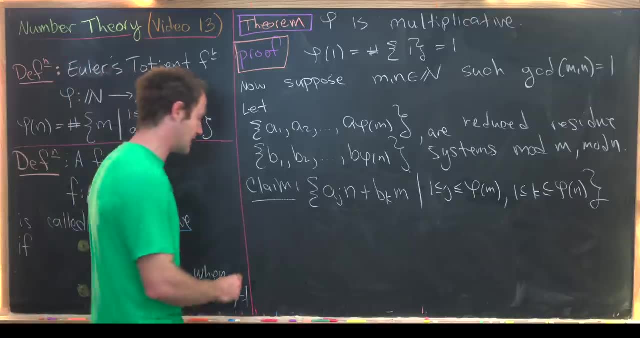 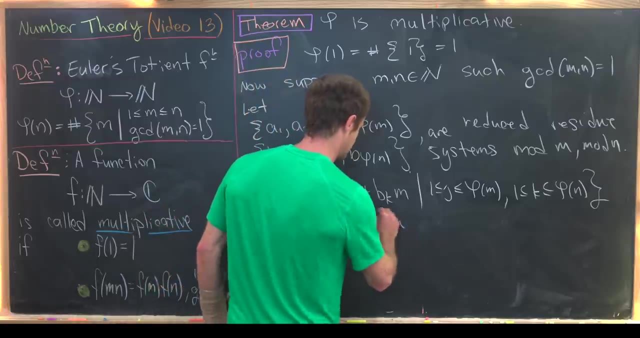 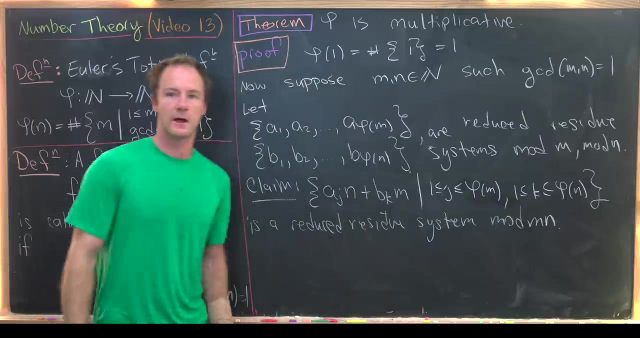 phi of m And then k must go between 1 and phi of n. So this is the set that we're looking for, And our claim is that that is a reduced residue system. modulo m- n. Okay, Well, let's see, maybe how this would help. So this is a reduced residue system. 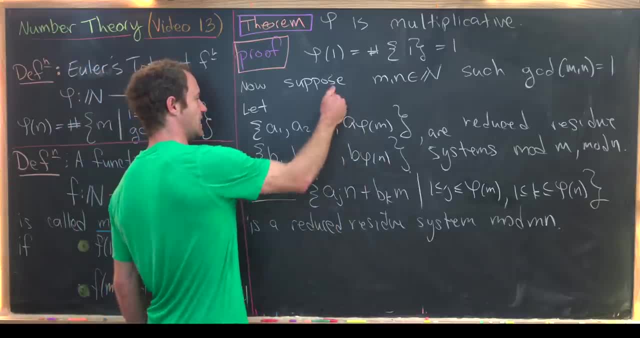 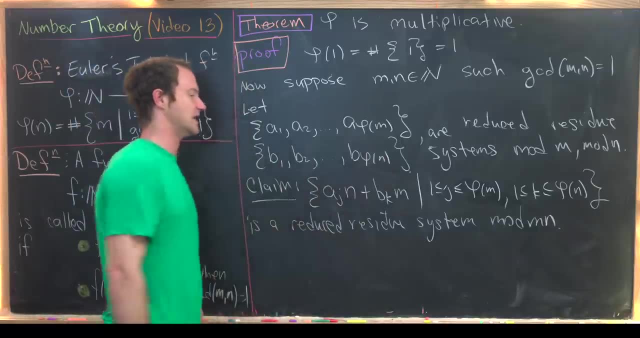 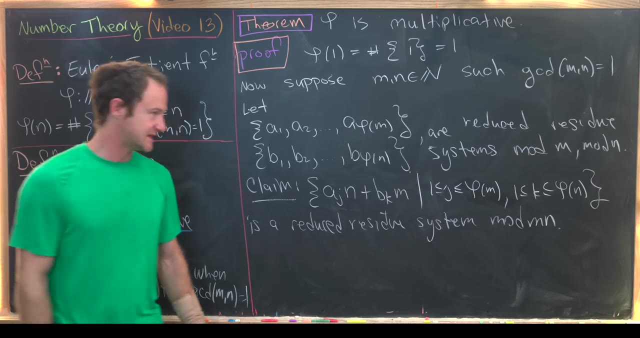 modulo m, And how many elements are in there. Well, there are phi of m elements in there. This is a reduced residue system. modulo n: There are phi of n elements in here, But then, by the construction of this set, this set contains phi of m times, phi of n elements. 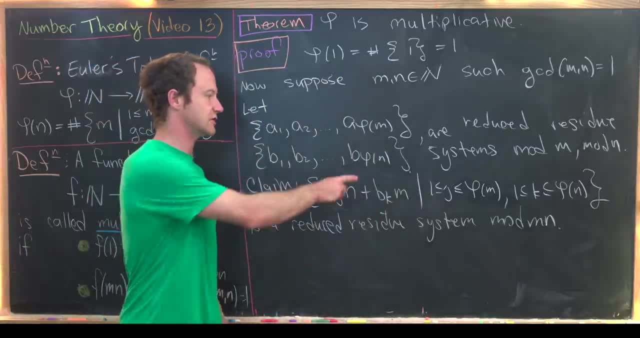 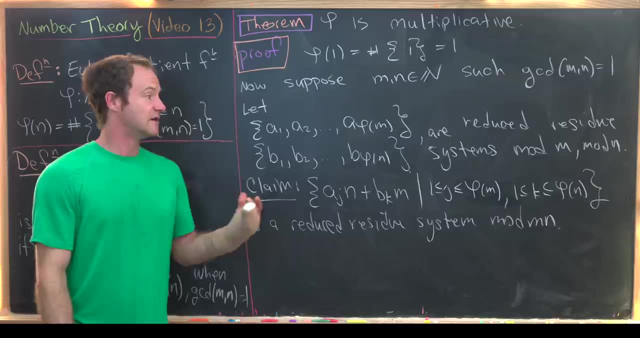 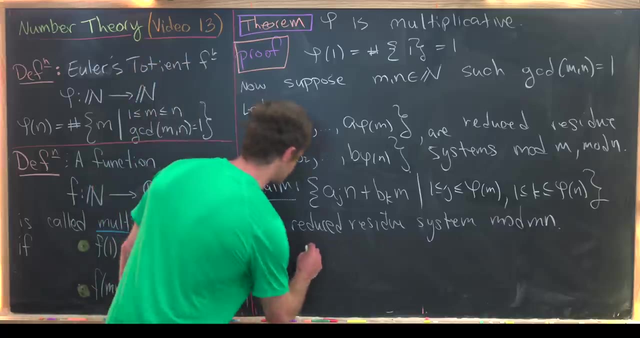 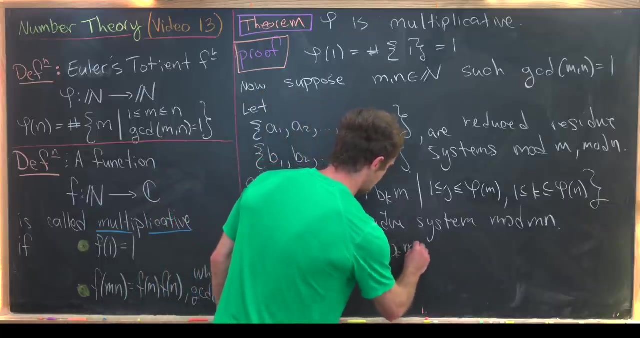 So if we can prove that it's a reduced residue system modulo m n, then that means phi of m? n is the size of this set, which is phi of m times phi of n, And then we're good to go. Okay, so we'll start the proof of this claim with a couple of observations. So, first off, the GCD of a j n plus b k m with the number m is the same thing as the GCD of a? j n with m. 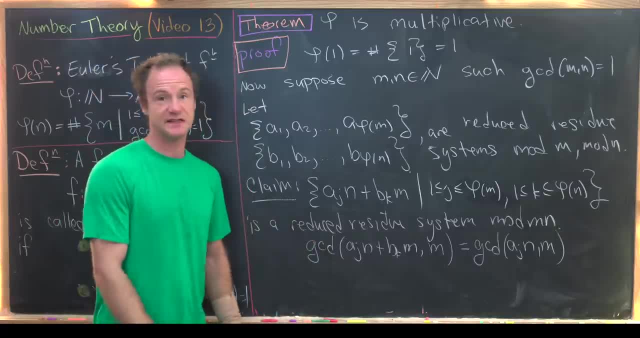 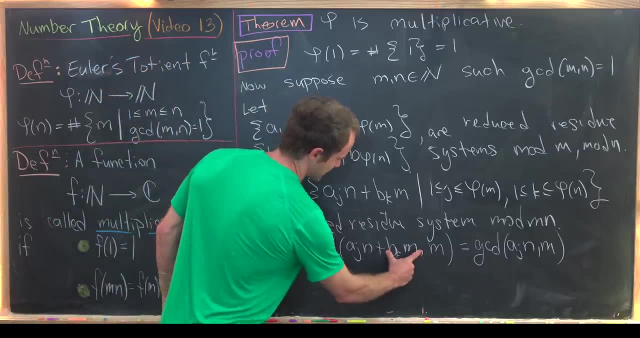 So why is that? Well, that's from one of the properties of the GCD that we proved several videos ago when we were looking at the Euclidean algorithm. So notice, here we've got a multiple of m. If we take this multiple of m away, then all we're left with 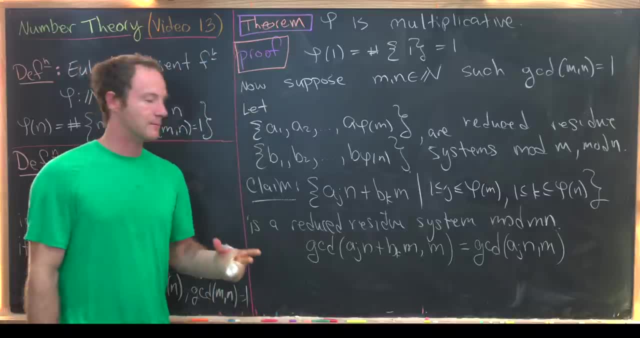 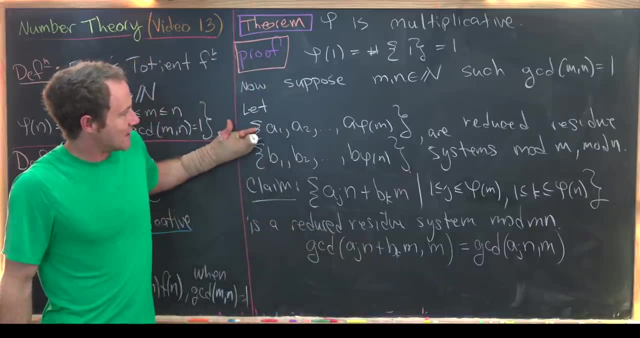 is the GCD of this number and this number. But next let's notice that a, j is relatively primed to m, given that it's an element of this reduced residue system. n is relatively primed to m, given that it's an element of this reduced residue system. 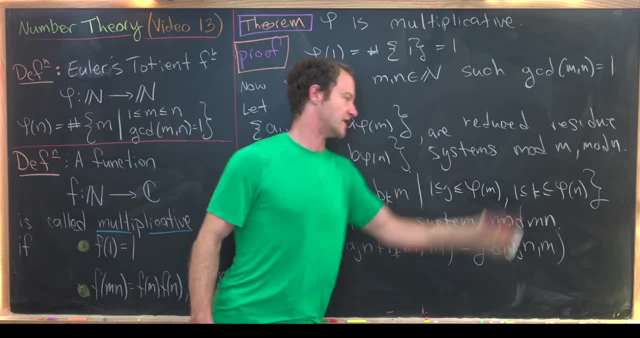 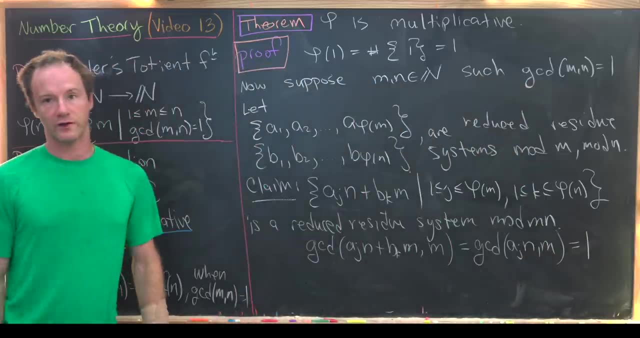 n is relatively primed to m, given that it's an element of this reduced residue system That's by our given up here. That means the product is relatively primed. So that means we've got a GCD of one right here, But now we can symmetrically play this game having an n here. 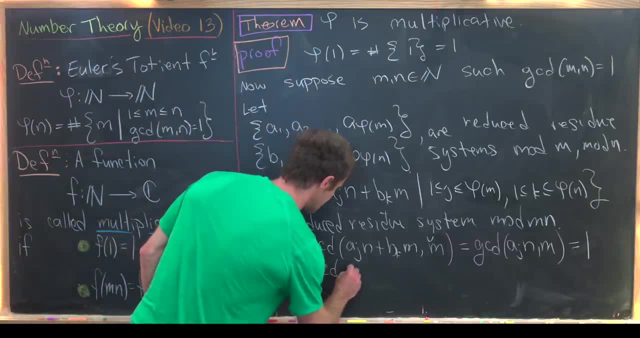 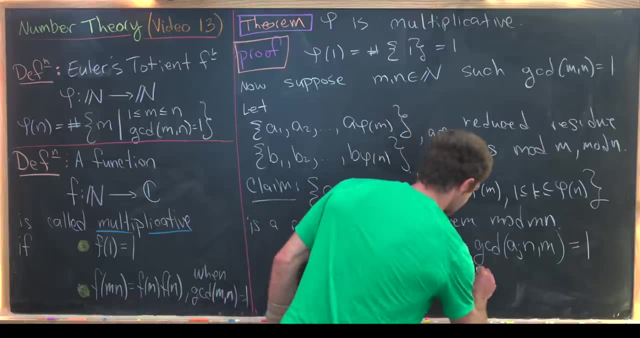 instead of an m here. So we've got the GCD of a j n plus b k m with n is the same thing as the GCD of b k m. So we've got the GCD of a j n plus b k m with n is the same thing as the GCD of b k m with n is the same thing as the GCD of b k m. 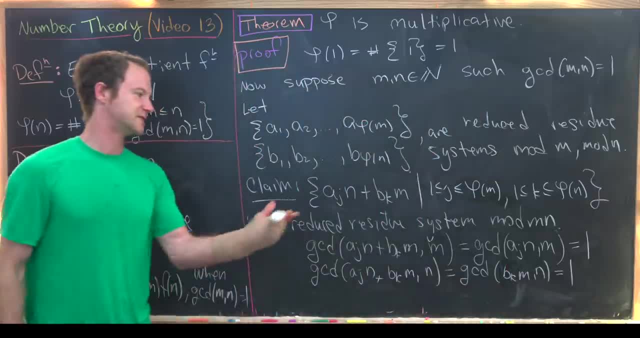 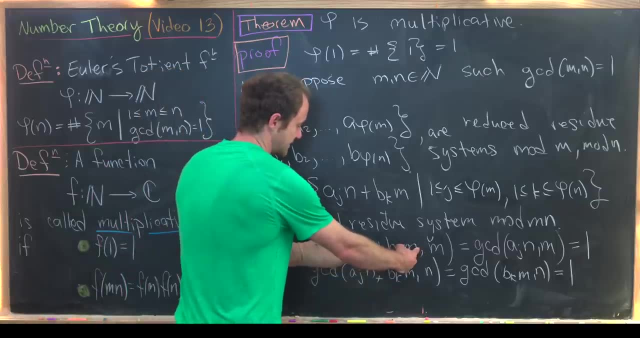 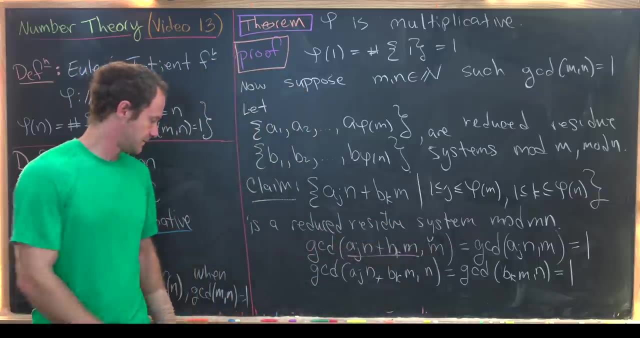 again kind of symmetrically for the same reason. But now let's look at what we've got. So we've got the GCD of this number right here, which may be- i'll underline in pink with the number m is one, and then this number that i'll underline in purple. 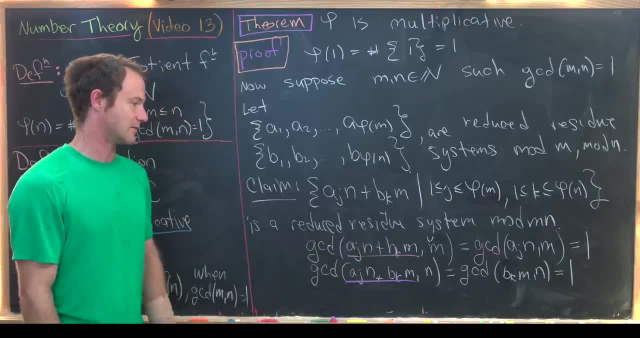 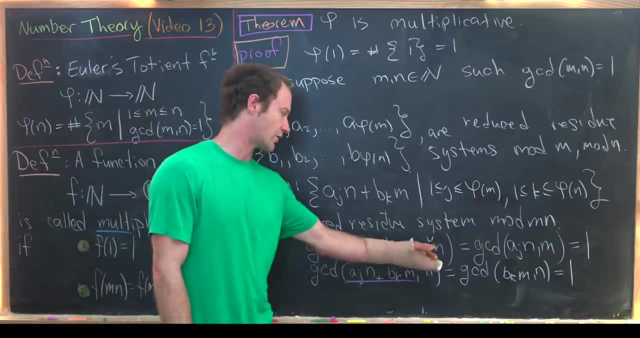 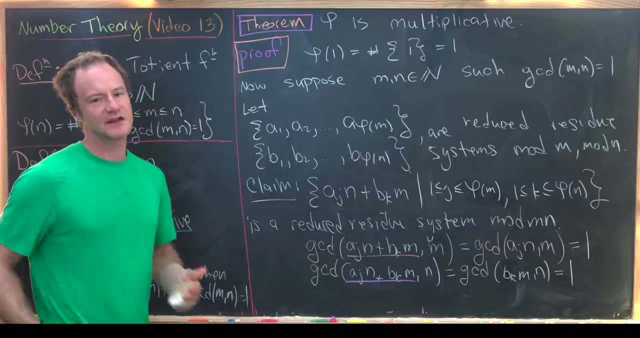 which is the same as the number in pink, has a GCD of n with one, But it's the same thing as the number in pink. those two pairs are both relatively prime to M and N, then they are relatively prime to the product of M and N. So, again, that's one of the properties of the GCD that we proved. 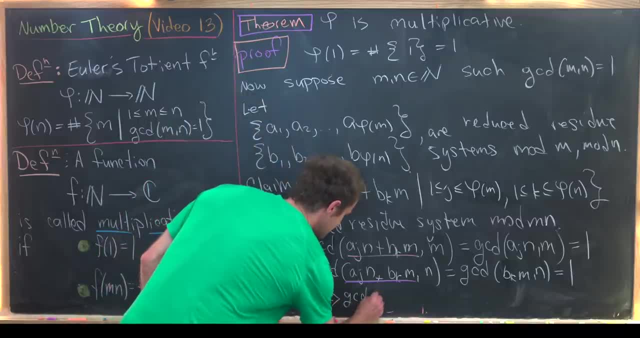 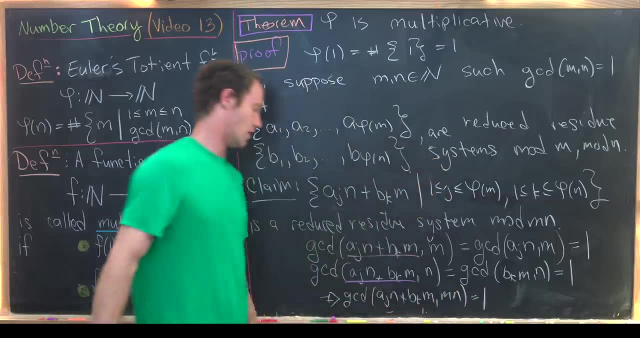 early on. So notice that means that we have the GCD of A, J, N plus B, K, M with M, N is equal to 1. And that's one of the properties we need for this set to be a reduced residue. 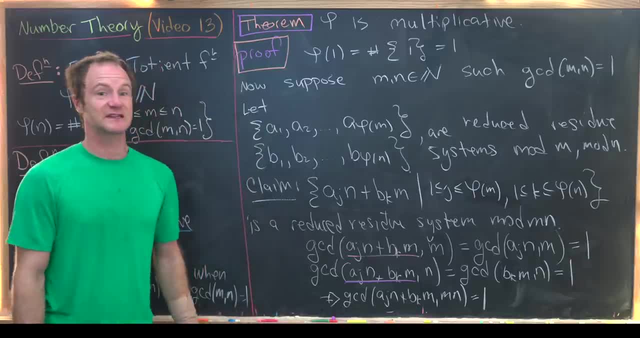 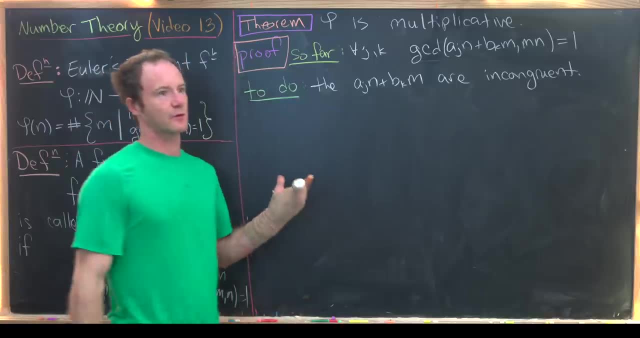 system. Okay, so let's maybe summarize what we've got at the top and then we'll move on to the next step. Okay, so where are we along the path of this proof? We started with a reduced residue system, mod M, and another one, mod N, and we constructed this would-be. 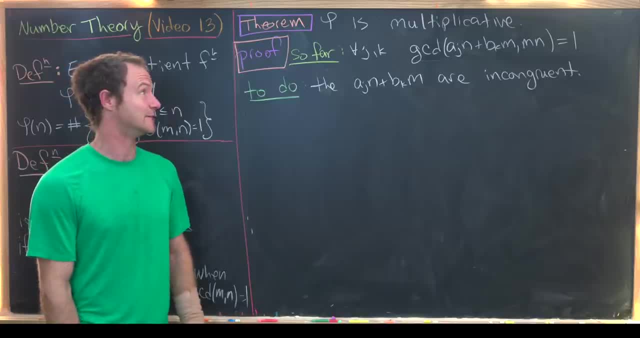 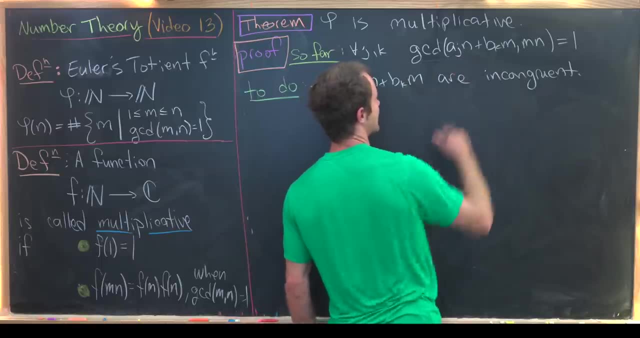 reduced residue system. module of the product M times N. So so far we've shown that this GCD of A, J N plus B K M with M N is equal to 1.. So so far we've shown that this GCD of A, J N plus B K M with M N is equal to. 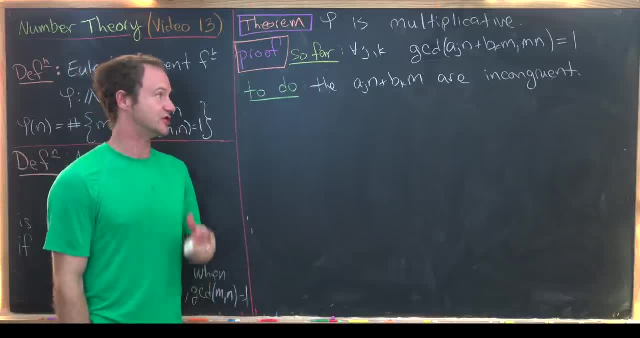 So so far we've shown that this GCD of A, J, N plus B, K, M with M, N is equal to 1. So the GCD requirement of being a reduced residue system is good to go. Now we just have to. 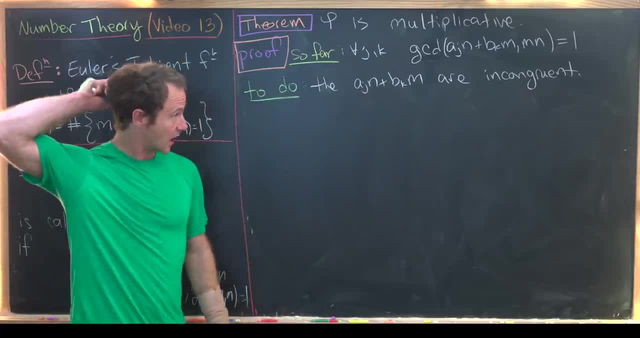 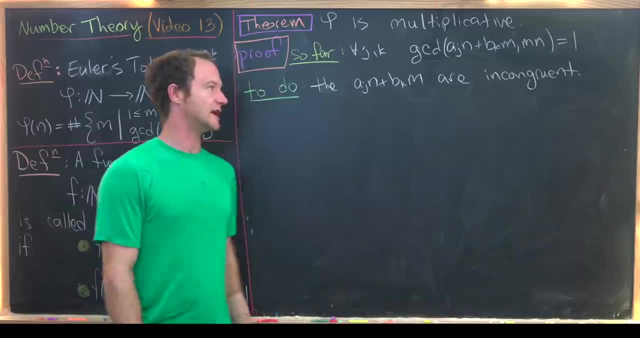 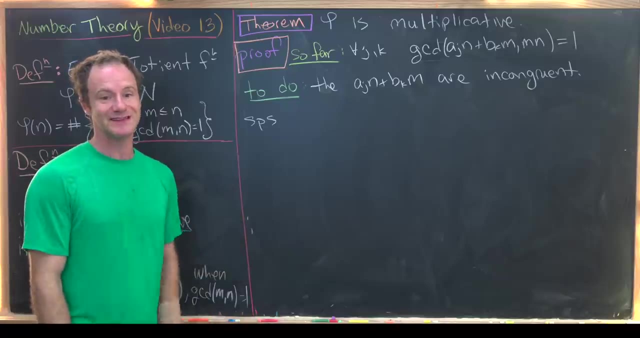 show that all of those things making up that set are incongruent- and we have enough of them. So let's do this part first. We want to show that all of these are incongruent, modulo M, N. So let's start by supposing that we've two, got two of these that are 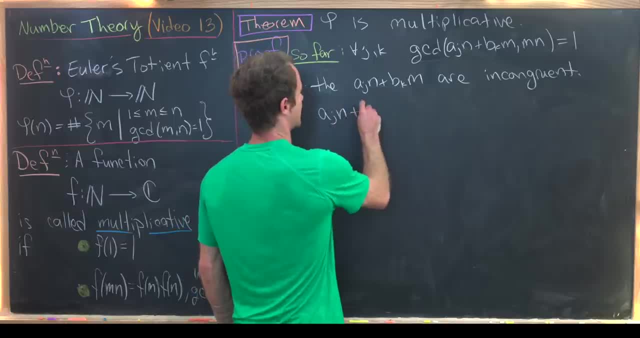 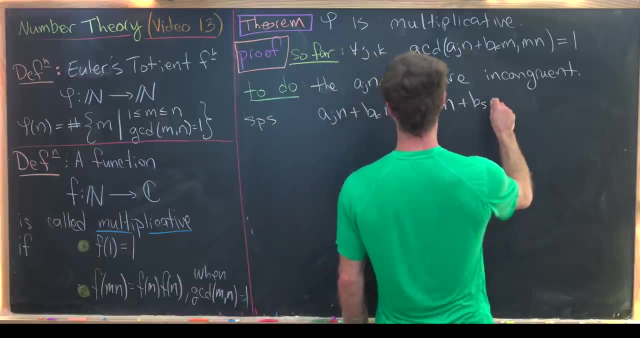 congruent. So I'll say A, J, N plus B K M is congruent. So let's start by supposing that these are congruent to A, R, N plus B S, M, and this is occurring modulo M N like. 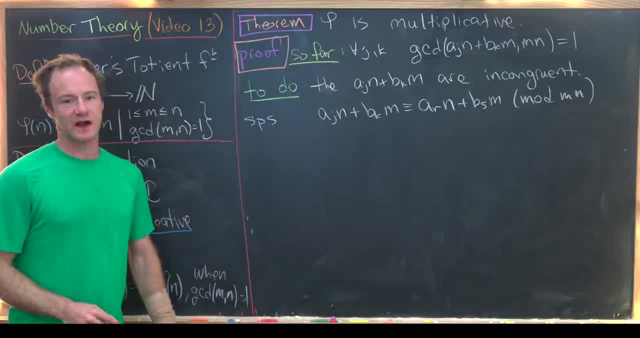 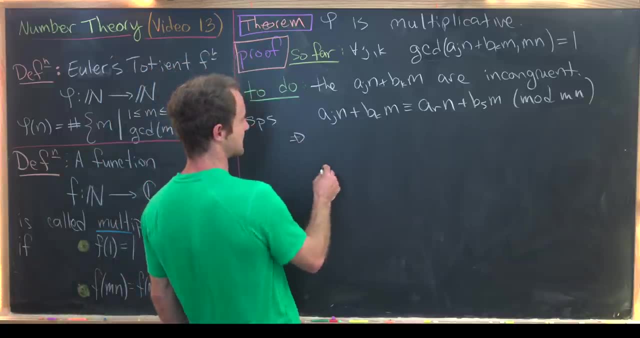 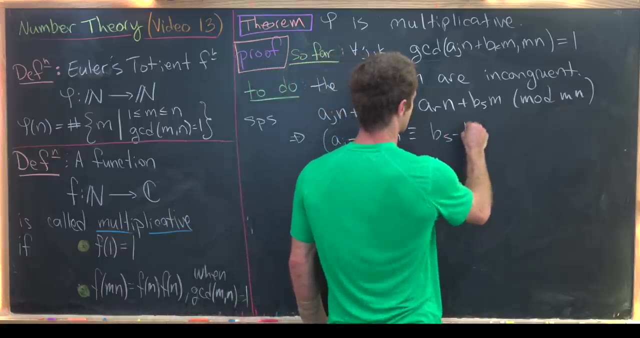 that Okay. well, let's move some things around. So we've got a multiple of N on one side and a multiple of M on the other side, So that's going to give us something like A J minus A R times. N is congruent to B? S minus B K M, So that's going to give us 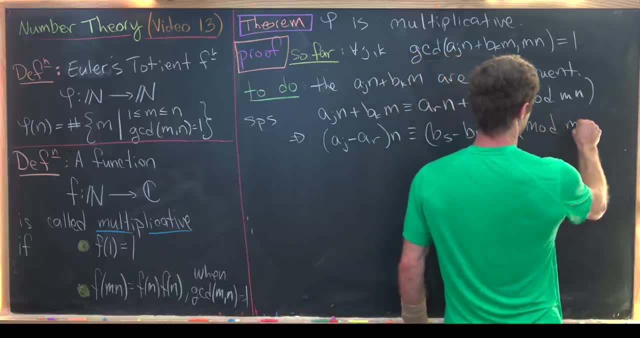 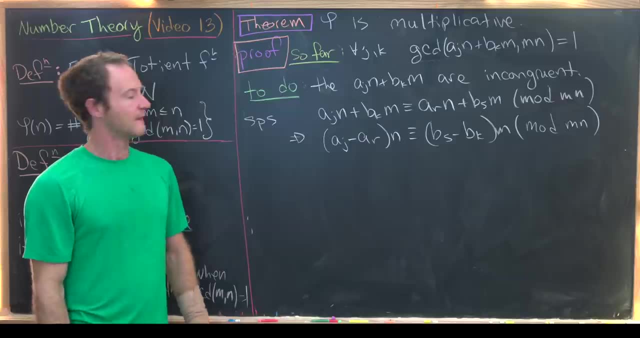 something like A J times M, and that again is all happening. mod M, N. So that's just moving this A R over and that B K over. Okay, but let's see what we've got. The left-hand: 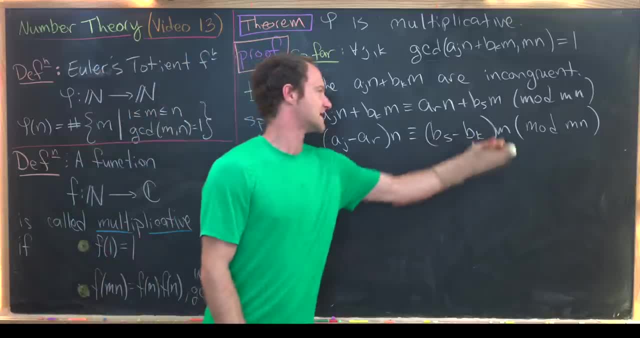 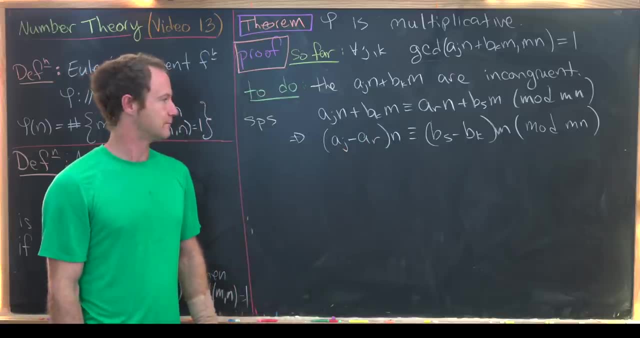 side is a multiple of N. The right-hand side is a multiple of M, But N and M are relatively prime. but that tells us that the multiple of M is a multiple of M. So that's going to give us something like A J minus A R, So we've got a multiple of M. that's occurring. 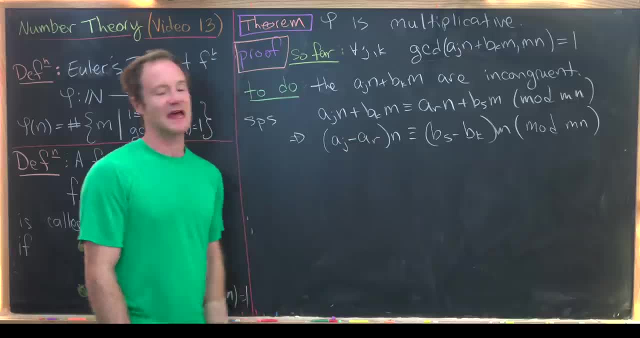 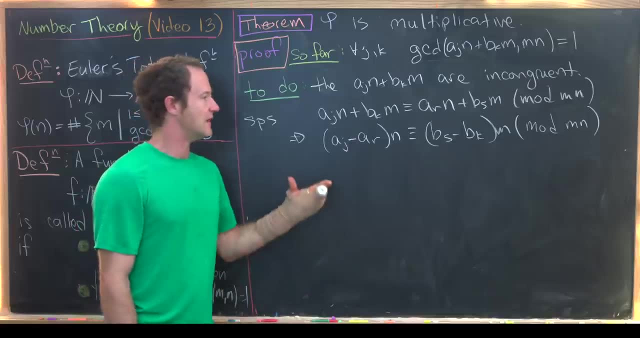 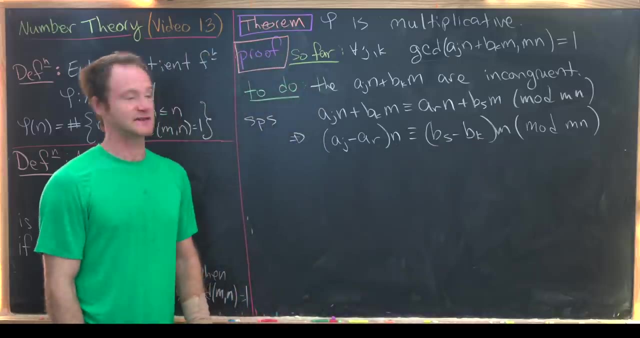 on the left-hand side must be wrapped up in this: A J minus A R, because since the right-hand side's a multiple of M, so is the left-hand side. And then, furthermore, the multiple of N that occurs on the right-hand side is wrapped up in this B S minus B K, Again because 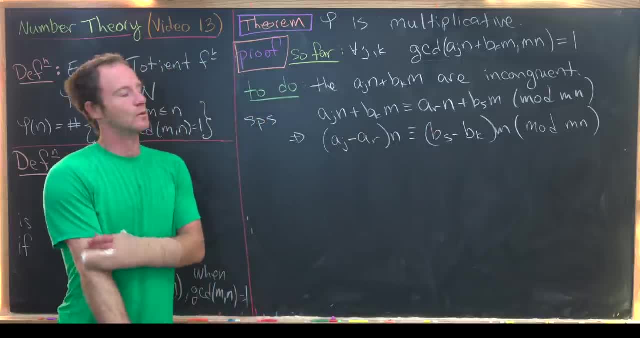 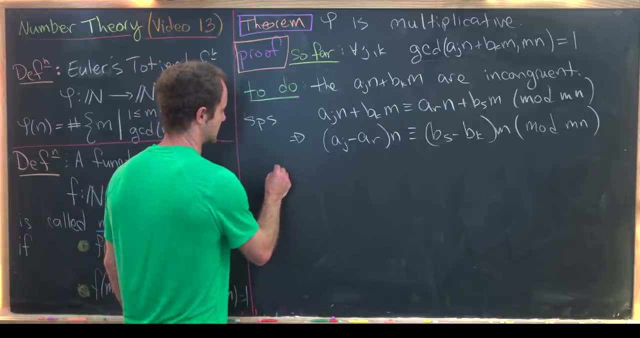 the left-hand side's a multiple of N, so is the right-hand side. We're only able to do that because these two numbers are relatively prime. Okay, So let's summarize that split as follows: We have A J minus A. R is congruent to zero. 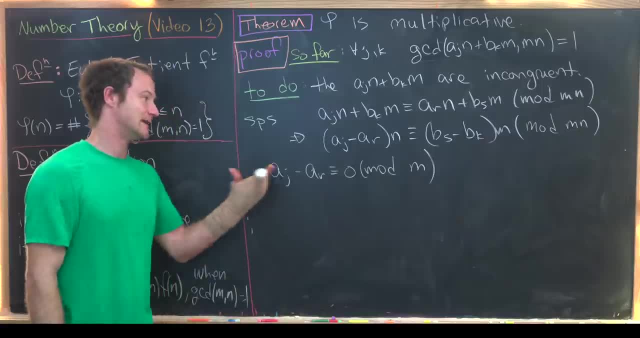 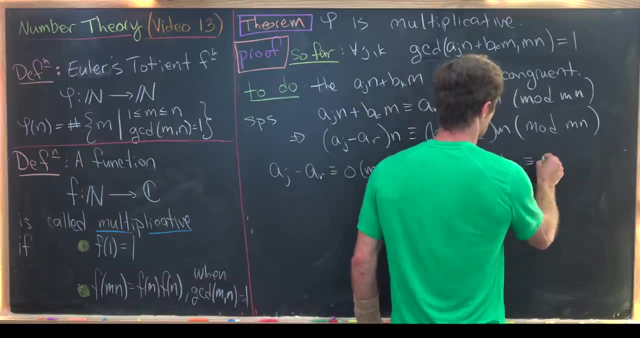 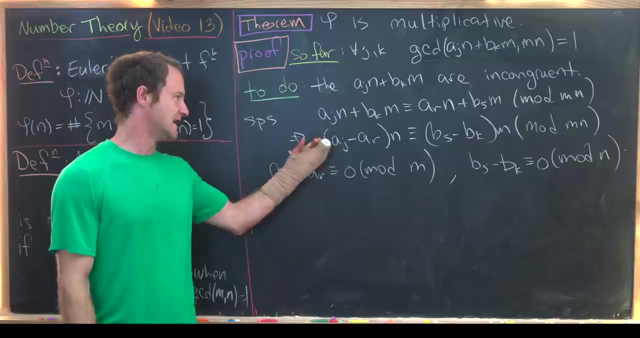 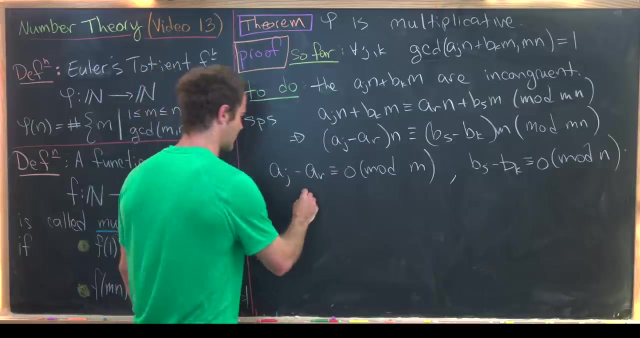 modulo M. Like I said, it's a multiple of M, And then likewise B S minus B K is congruent to zero mod N. Okay, So that appropriately summarizes that discussion that I said in words. Okay, But now we can move this stuff around a little bit. We get A. J is congruent to A R modulo. 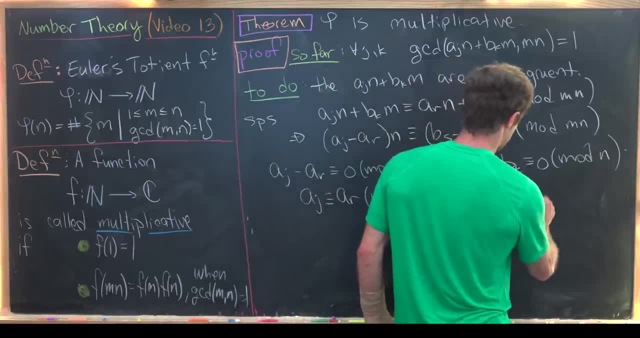 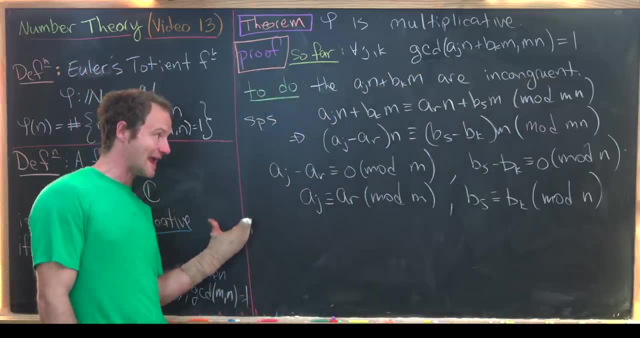 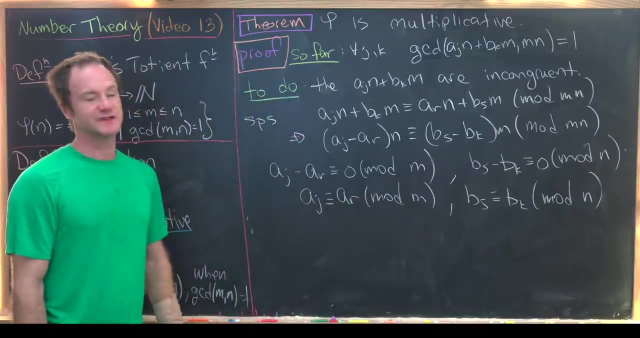 M And then B S is congruent to B K modulo N. But now let's recall: since the A's form a reduced residue system, mod M and the B's form a reduced residue system, modulo N, then that means they are either: 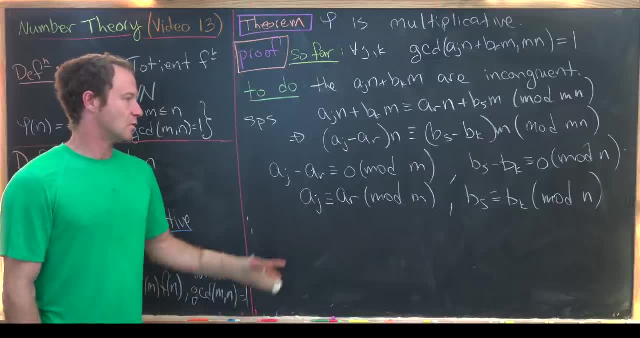 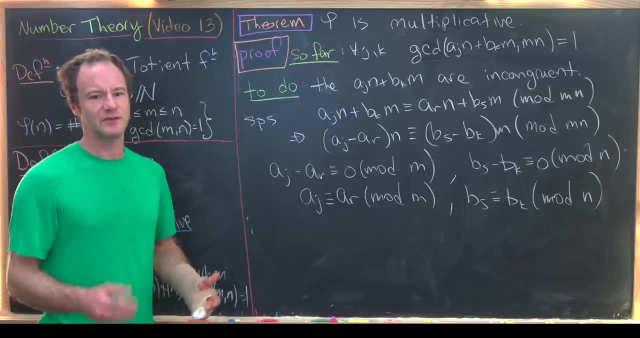 Well, since these things are congruent, then they must be equal. That's part of it being a reduced residue system instead of, maybe, just a residue system. Okay, So that tells us that J is equal to R, or maybe A J is equal to A R, But really. 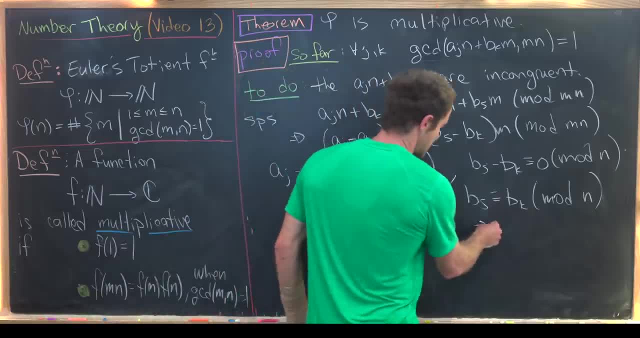 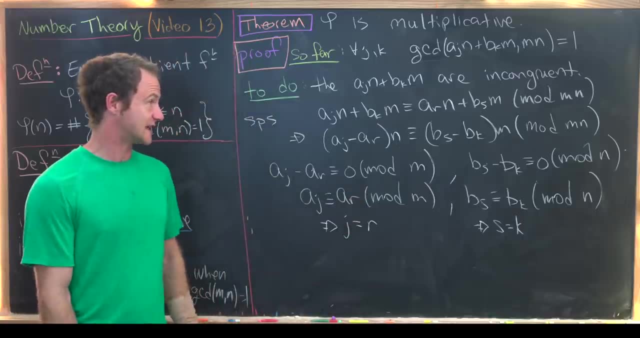 the indices being equal is enough. And then this down here implies that S is equal to K. But now, if J is equal to R and S is equal to K, then that means that A J is equal to A R. Okay, 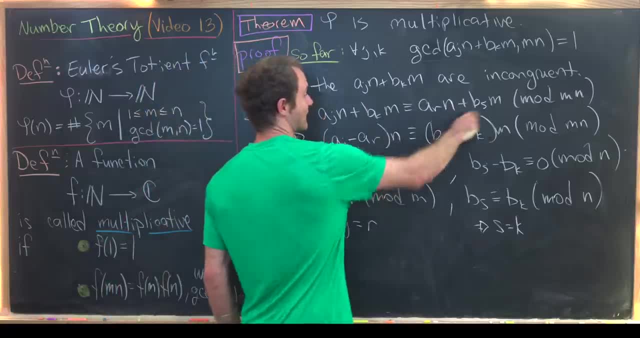 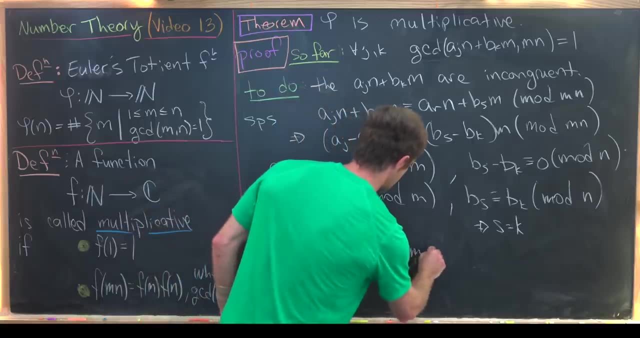 So if we have a reduced residue system, mod K, then that means we don't just have congruence up here, but we have equality up here. So we've got A, J, N plus B, K. M is equal to. 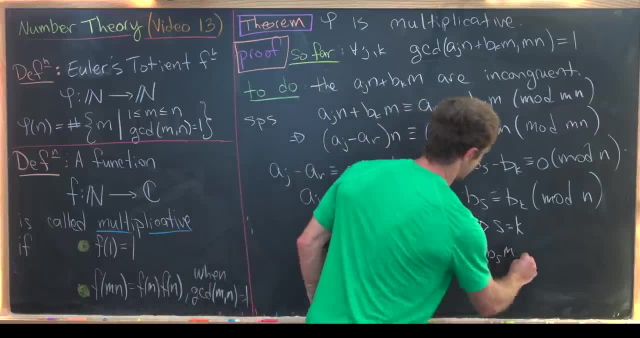 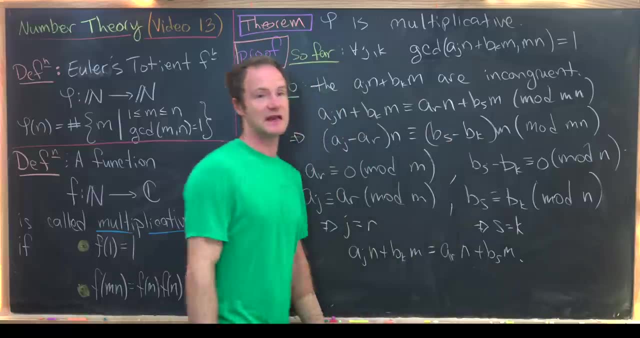 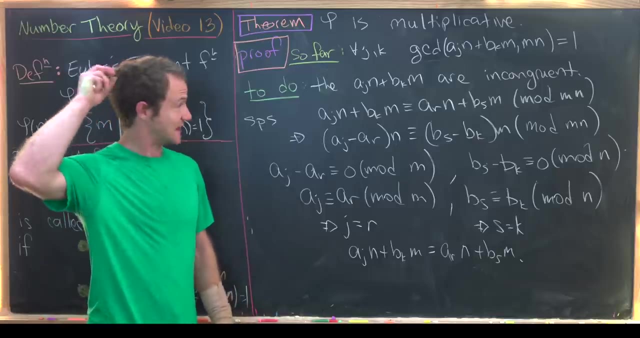 A, R, N plus B, S, M. Okay, So let's back up and summarize So this fact that the GCD of this object with M and N is equal to 1, that means one condition of the reduced residue system is satisfied. 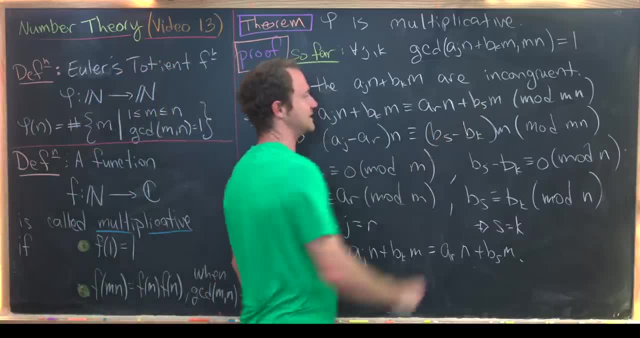 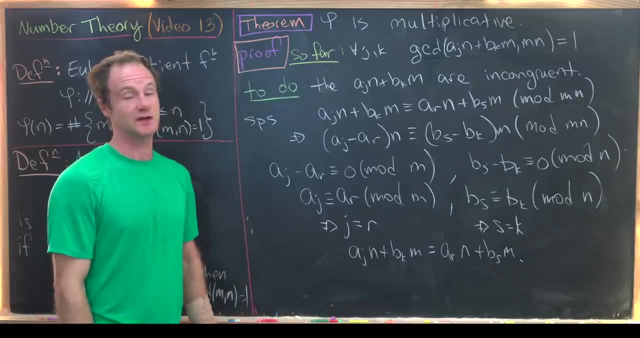 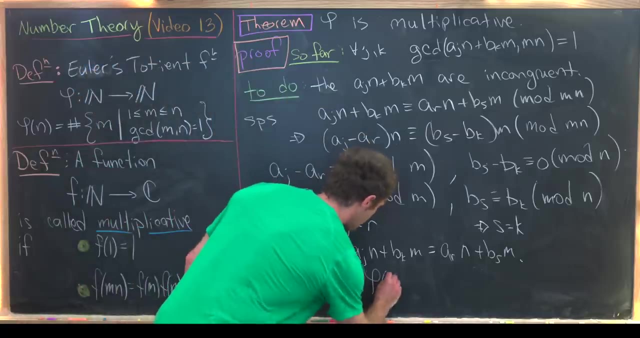 Okay, satisfied. The fact that the only way for these to be congruent, mod mn is for them to be equal, is another part of the reduced residue system to be satisfied. But that actually doesn't finish the proof of this. That only gives us an inequality. So so far we see that phi of mn. 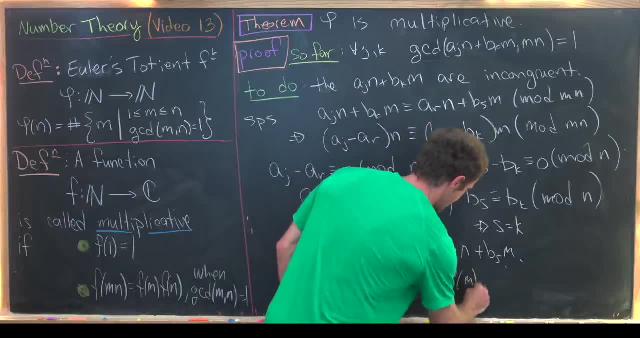 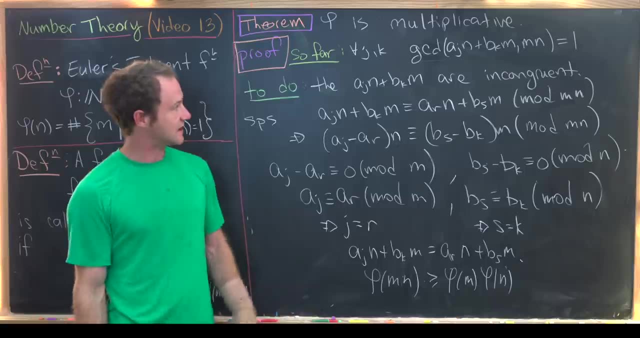 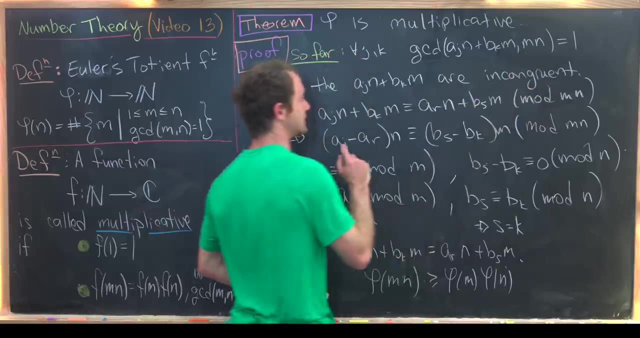 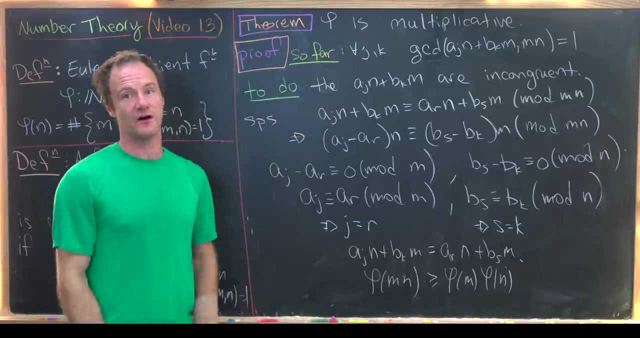 is bigger than or equal to phi of m times phi of m. So let's recall that our set of phi of m times phi of n numbers were made up of numbers of this form. So we showed that we have the GCB requirement, and congruence implies equality, but we haven't yet showed that we have enough of the 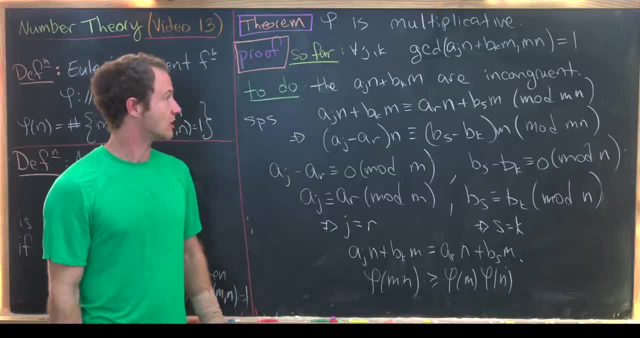 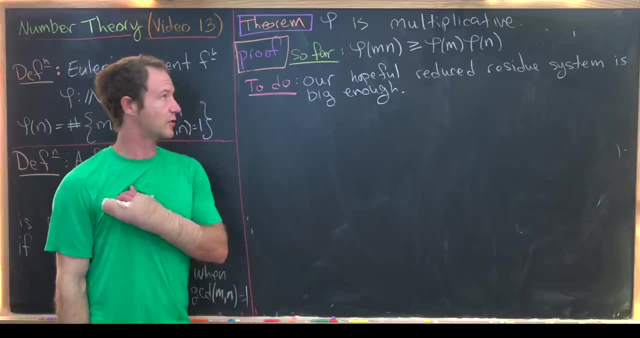 elements in that set. So that's the last thing that we need to show, But we don't have room for that. So let's get rid of that and then we'll do that. proof, Okay. So so far we've proved that if 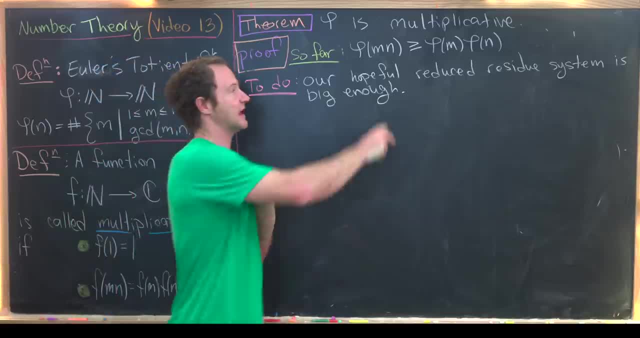 we've got relatively prime natural numbers n and n, that phi of mn is bigger than or equal to phi of mn. So that's the last thing that we need to show: phi of mn is bigger than or equal to phi of m times phi of n, And that involved constructing. 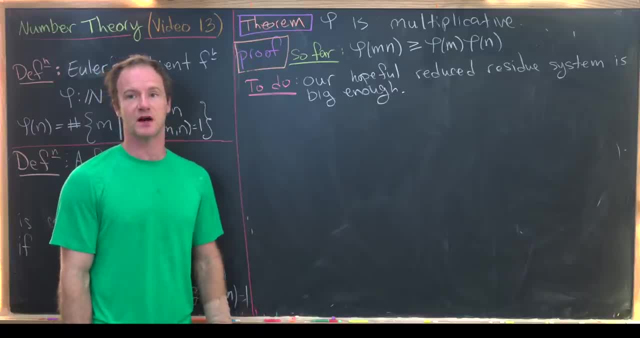 what is a would-be reduced residue system modulo mn out of reduced residue systems modulo m and n, And what is left to do is show that our hopeful reduced residue system is big enough. So in some ways we've shown it is not too big already. Now we want to show that it's big. 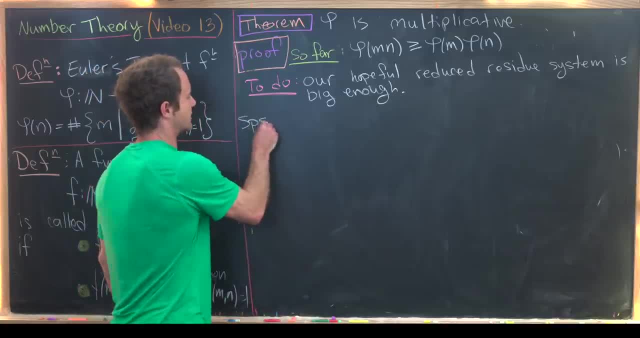 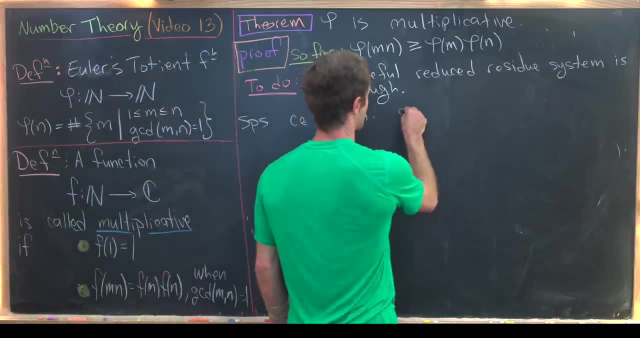 enough, Okay, So let's see how we can do that. So we're going to bring a new integer into the world. We'll call that c, So let's suppose c is an integer such that the gcd of c with m times n. 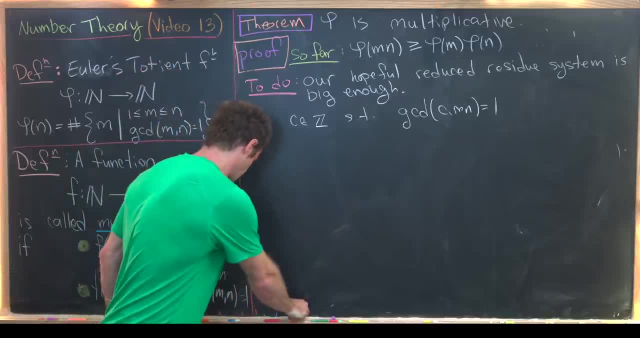 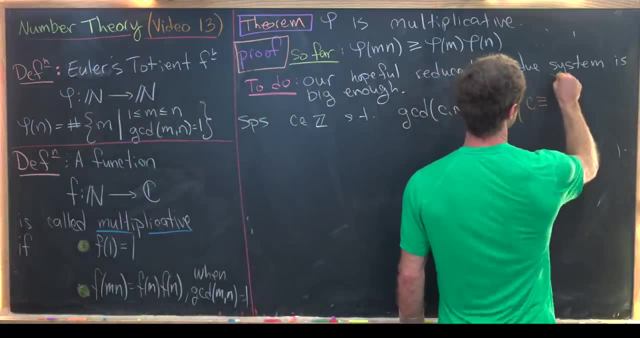 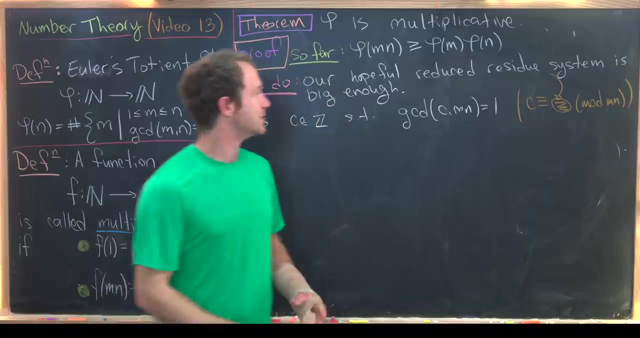 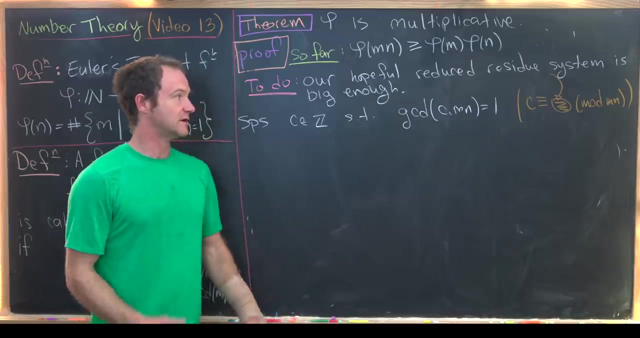 is equal to 1.. So, keeping in mind where we want to go, what we hope is that c is congruent to something from our would-be reduced residue system modulo mn, Because, remember, our hopeful reduced residue system should have all possible residues that are relatively primed to mn, including this random. 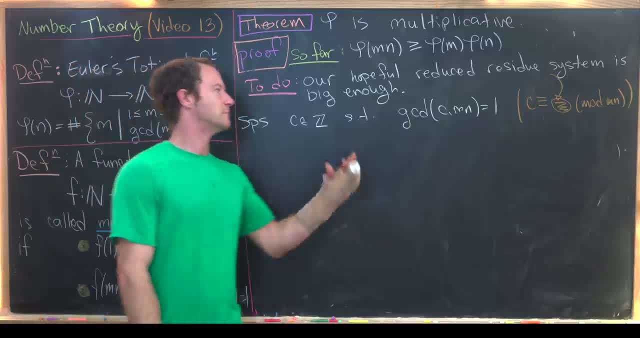 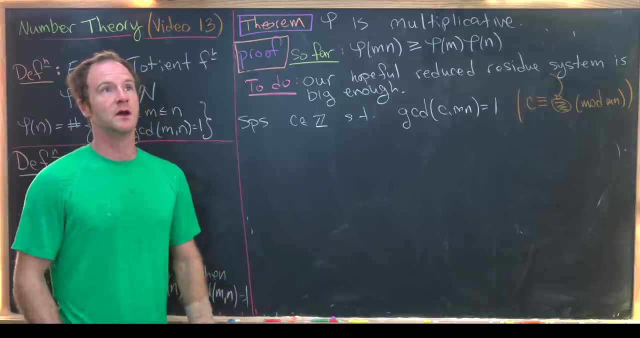 one c that we just picked. Okay, But what should you do if you see that the gcd of c with mn is equal to 1?? Well, you should maybe implore something called Baizu's identity, which we do all the time. So now we want to use the fact that m and n are equal to 1.. So we're going to. 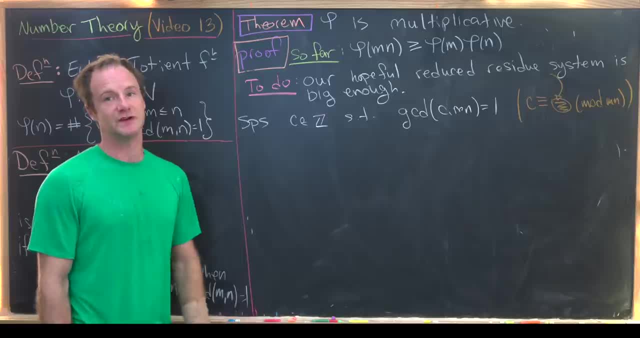 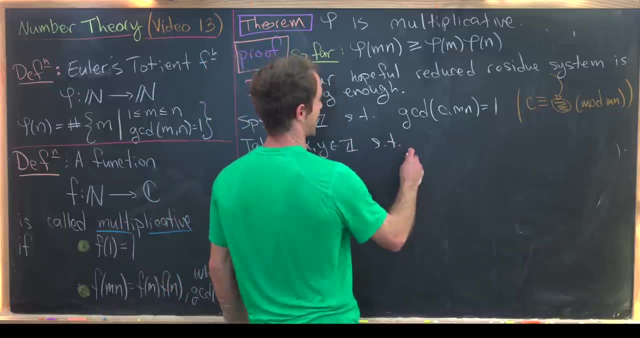 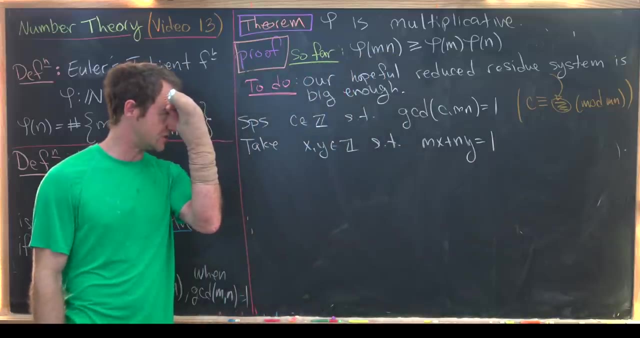 are relatively prime, And so let's use Baizu's identity. So, in other words, let's take integers x and y, such that mx plus ny is equal to 1. And again, that's possible because the gcd of m with 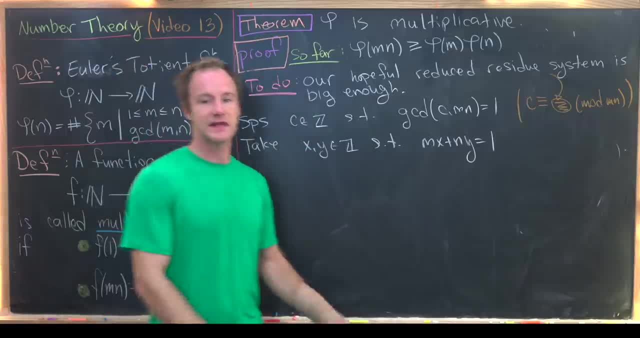 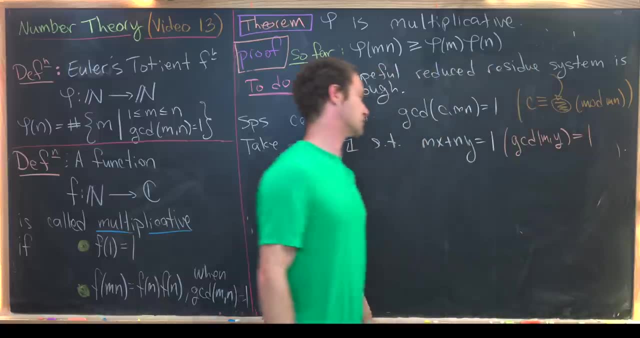 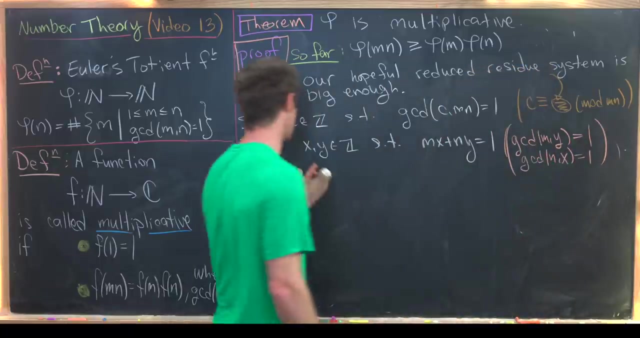 n is equal to 1.. But now let's notice that this means that the gcd of m and y is also equal to 1.. Because we've got a linear combination of m and y that creates 1.. And likewise the gcd of n with x is also equal to 1.. So, even though x and y were kind of brought into existence, 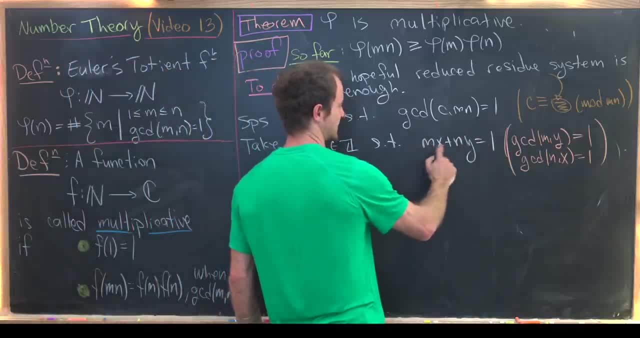 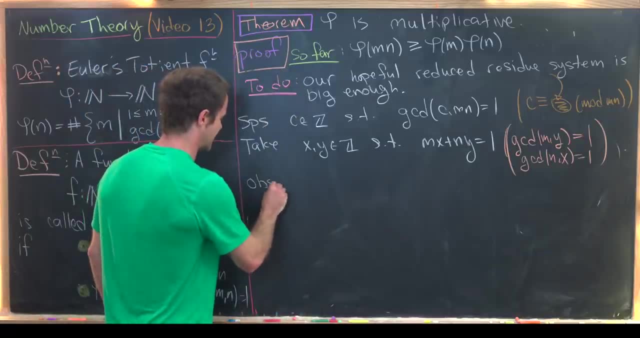 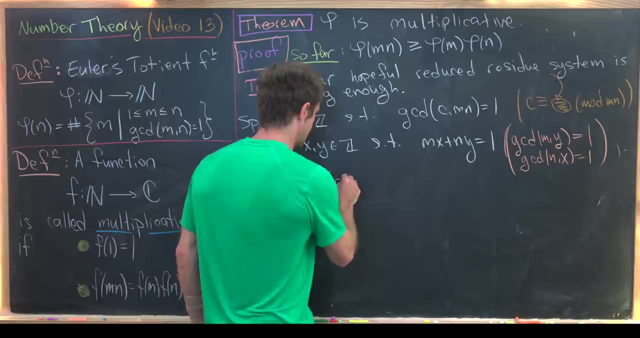 to create this, which uses the structure of m and n. we get this extra stuff kind of for free, Okay. So now let's look at the following observation which will be helpful, And that is: let the gcd of cy with m is equal to 1.. And then likewise, kind of in parallel, 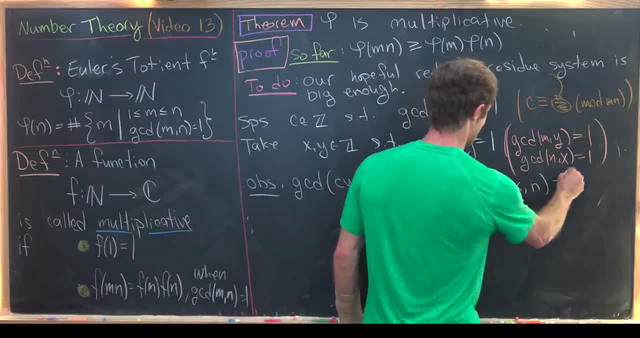 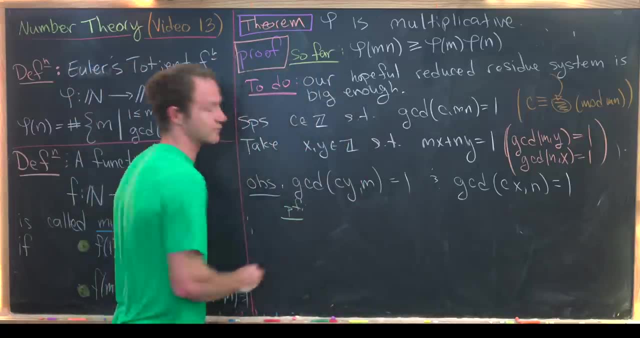 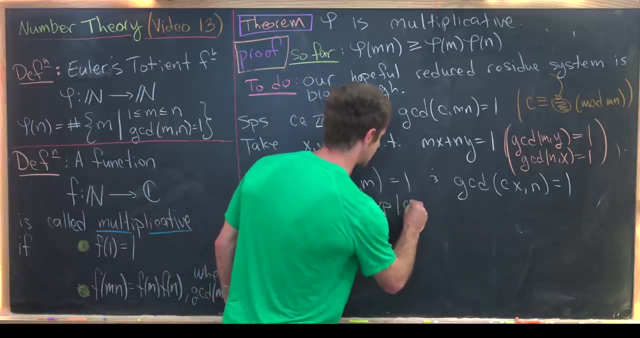 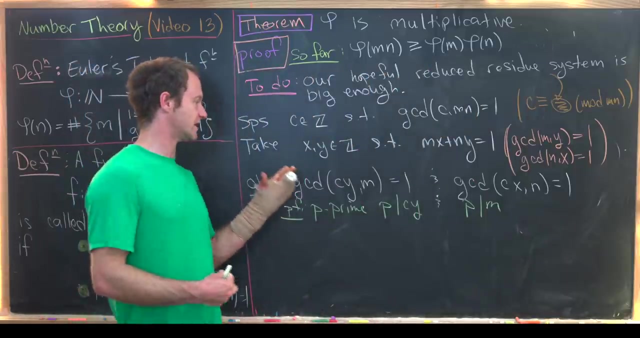 the gcd of cx with n is also equal to 1.. Okay, So let's run through the little proof of this observation really quickly. So let's suppose p is some prime and p divides c times y times c, Or p divides n and p divides m. In essence, what we're doing here is starting. 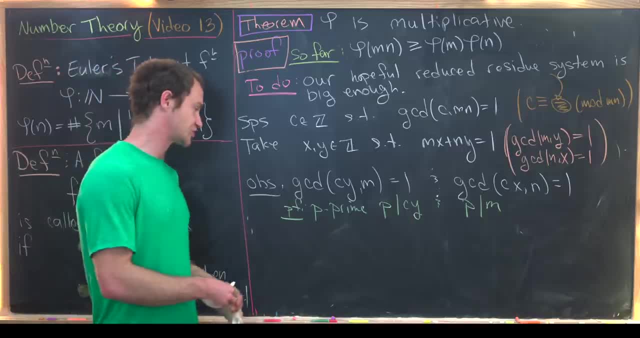 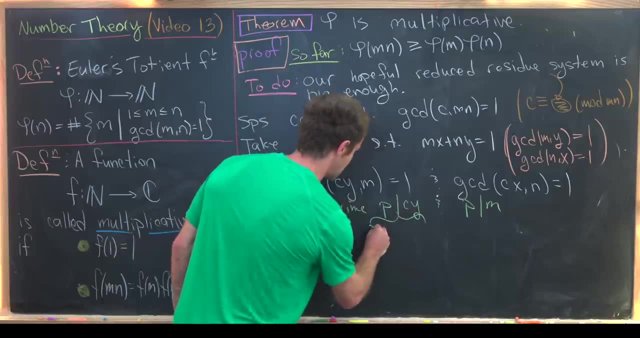 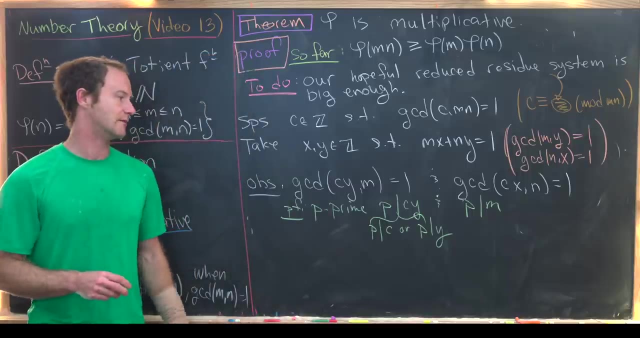 by assuming the gcd is not 1 and searching for a contradiction. Okay, So from here we can say that this means p divides c or p divides y. That's just a standard fact about prime numbers and when prime numbers divide products. Okay. So now let's see how we can break it down into a solution我們的 product dividen um into products. Now that we've extracted, the出来 is the number of variables that make D and Y the n per in D divided by c. So we can actually find the n that makes D divided by c times, p divided, z divided by C. What we're trying to do is just to growing up different pior video that we're doing our project into new formulas So we can set up exactly this example these times. 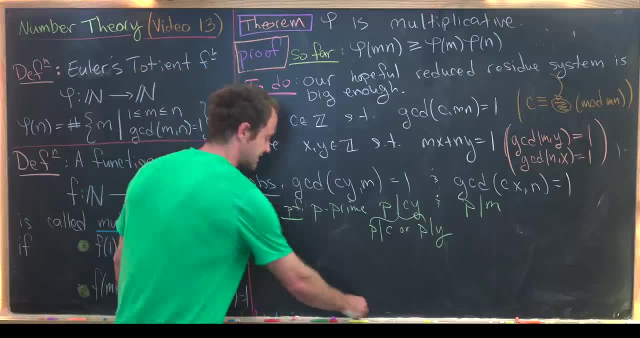 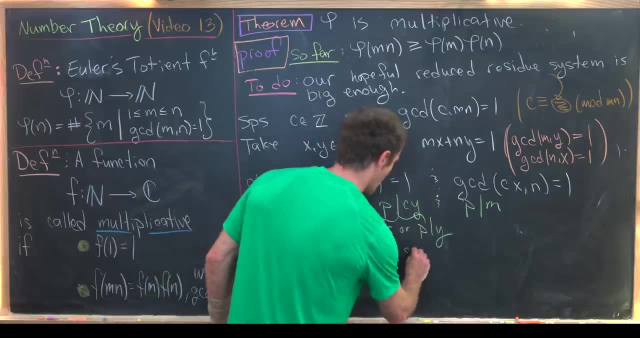 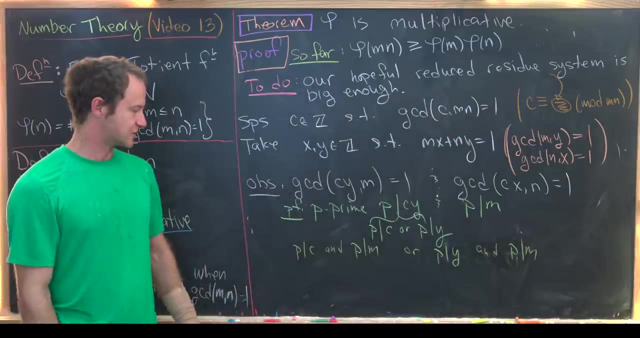 let's see how we can work off of both of these. So this splits into two cases: p divides c and p divides m, or p divides y and p divides m. But now we can do a bit of a trick If p divides m. 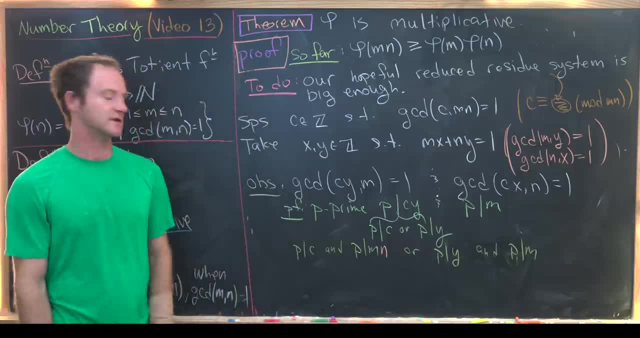 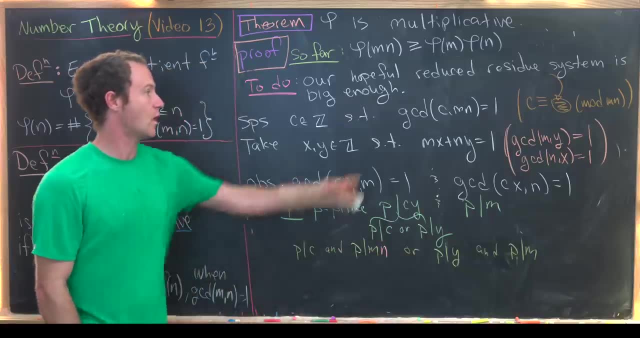 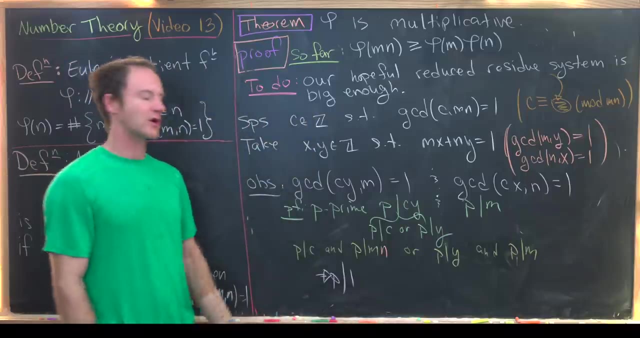 then p most definitely divides m in just by multiplying by n. Okay, but now we know the gcd of c with mn is equal to one. that's our assumption way up here. So this tells us that p divides one, but there are no primes that divide one. So that leads us to a contradiction. 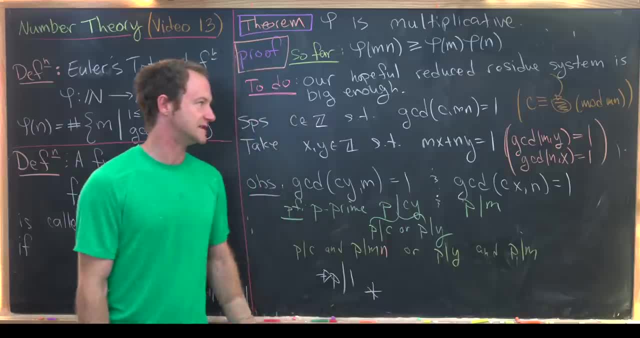 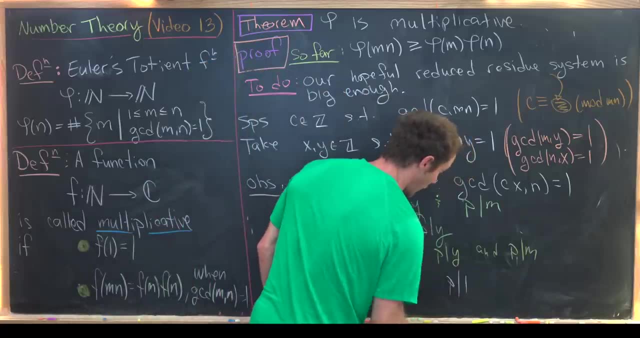 Now we move over here and we see that p divides y and p divides m, But this says that the gcd of m and y is equal to one, but that means p divides one. But again that's a contradiction because there are no primes that divide one. So that means 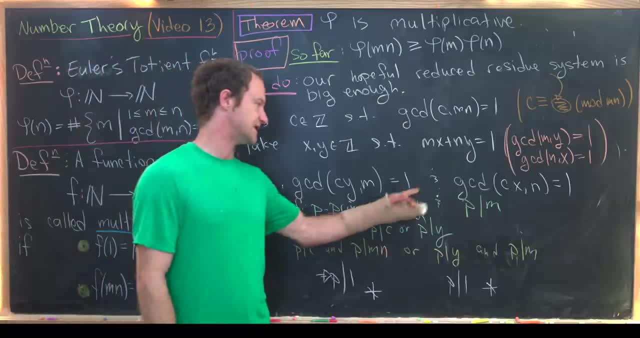 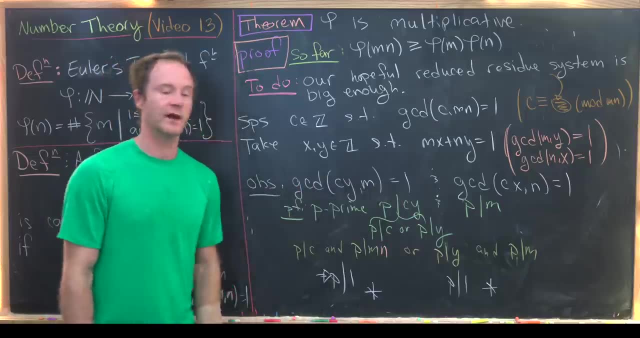 there are really no primes that divide both CY and CM, but the only way for that to be the case is for this GCD of CY with M to be 1.. And then symmetrically, we have the GCD of CX with N is. 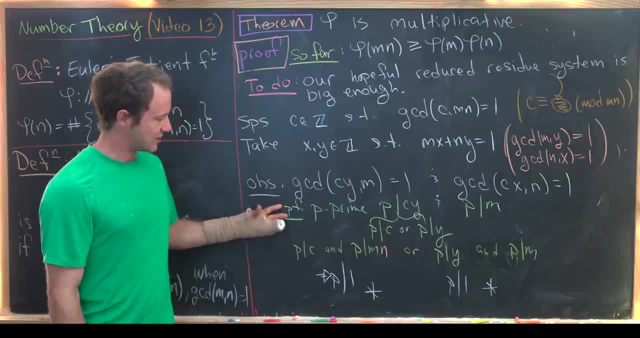 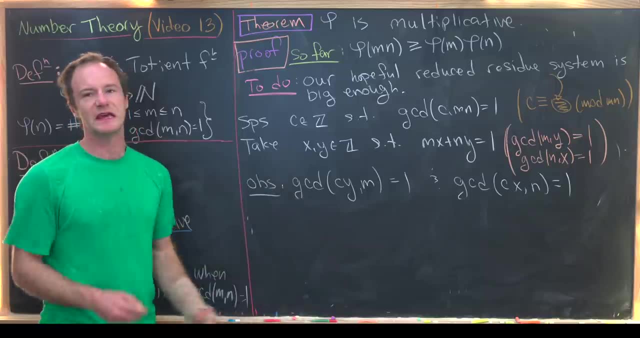 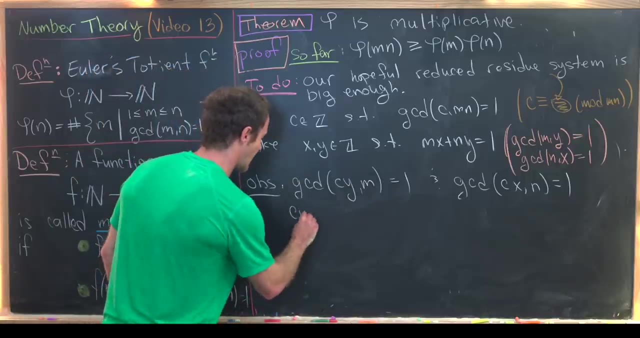 also 1.. Okay, so let's leave this observation up, but we'll get rid of this proof and then finish this off. Okay, we just got done arguing this observation. This is going to be key to finishing this off. So since the GCD of CY with M is 1, then that means that CY is congruent to 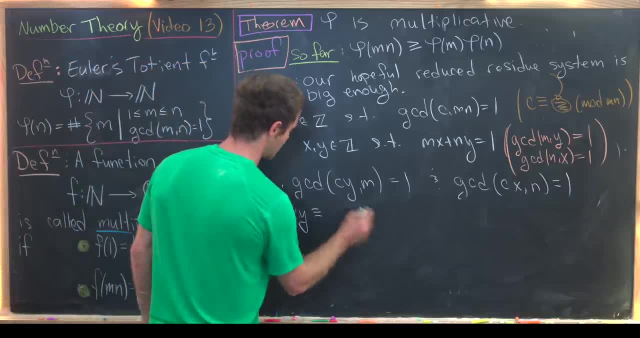 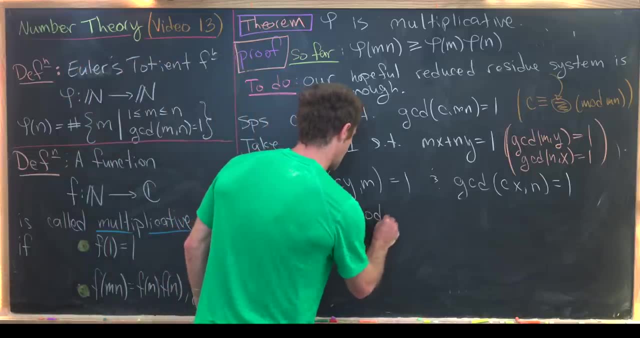 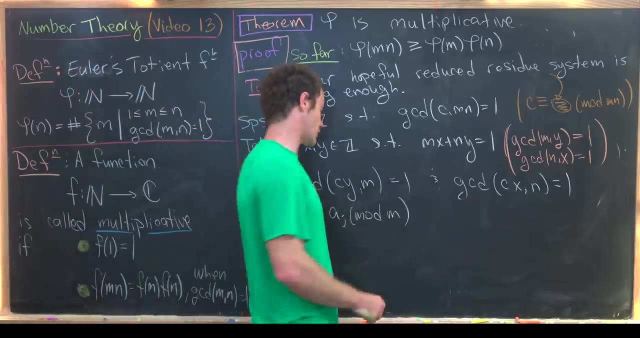 one of the elements from the reduced residue system of M, And so remember those were of the form A sub something. So we'll say A sub J mod M, And remember that J is going to go between 1 and phi of M. And then, similarly, this over here says that CX is congruent to B. sub M. So we'll say that CX is congruent to B sub M, And then similarly, this over here says that CX is congruent to B sub M, And then similarly, this over here says that CX is congruent to B sub M. 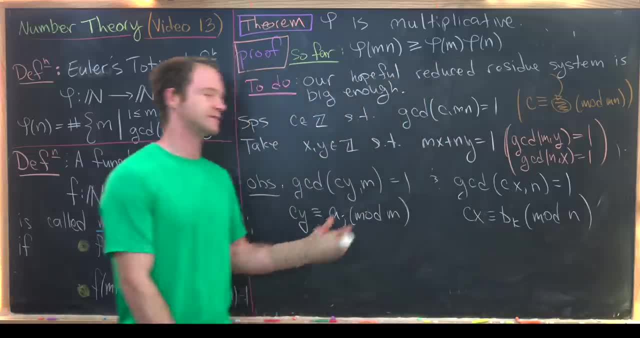 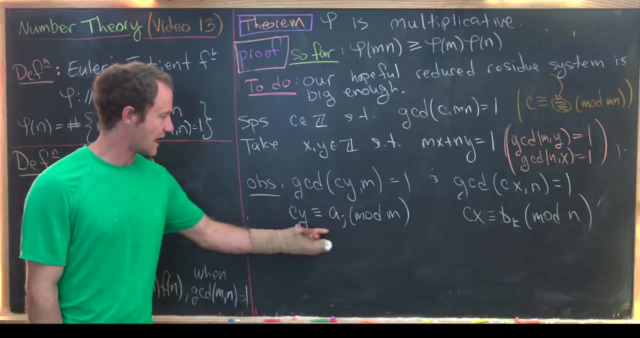 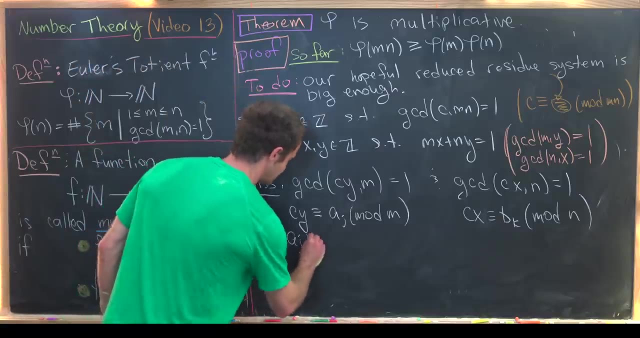 And then, similarly, this over here says that CX is congruent to B sub K modulo N Again, because we've got this reduced residue system And now we're actually ready to start finishing it off. So let's multiply both sides of this congruence by N And notice that that tells us that AJ times N is. 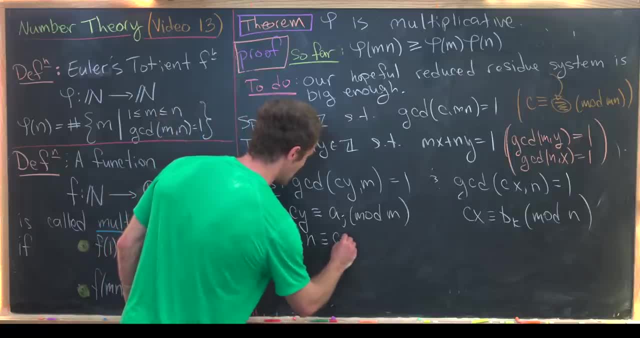 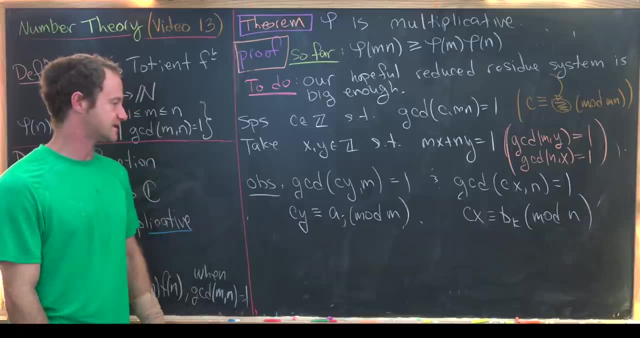 congruent to. let's see what we've got: CY times N modulo M. Now we've got all of the pieces in place to start finishing this off. So let's take this congruence which followed from our observation and multiply it by N. 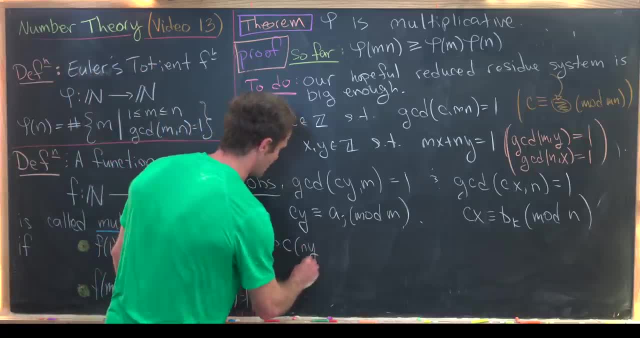 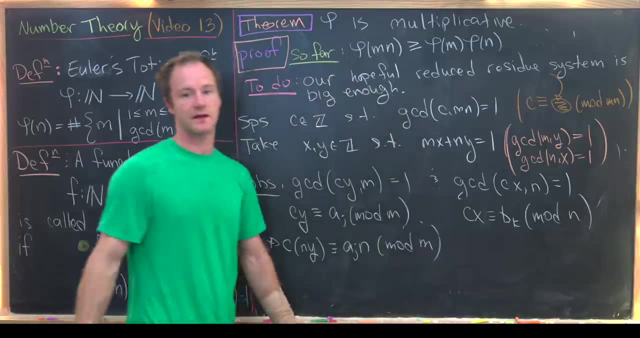 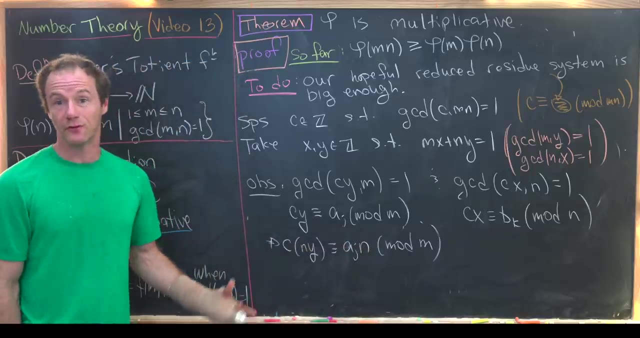 So notice that that is going to give us C times. NY is congruent to AJ times. N modulo M, Like that. And then from here we can freely add a multiple of M to the right hand side, And that doesn't change anything because M is congruent. 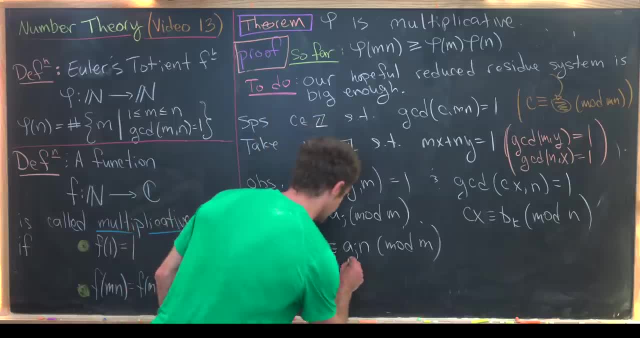 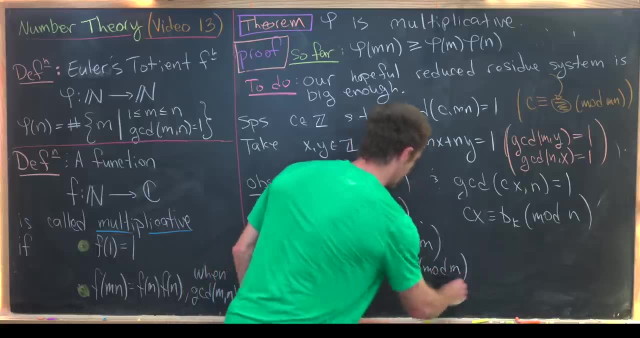 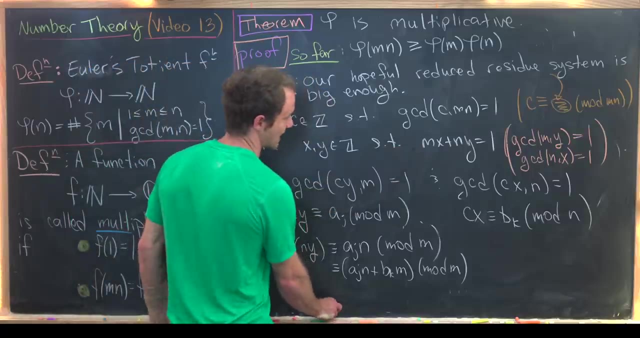 to 0 mod M. So notice, this is going to be congruent to AJN plus BKM mod M. Again, we just multiplied this fancy version of 0.. But now let's look back up at this equation right here and reduce this equation modulo M. 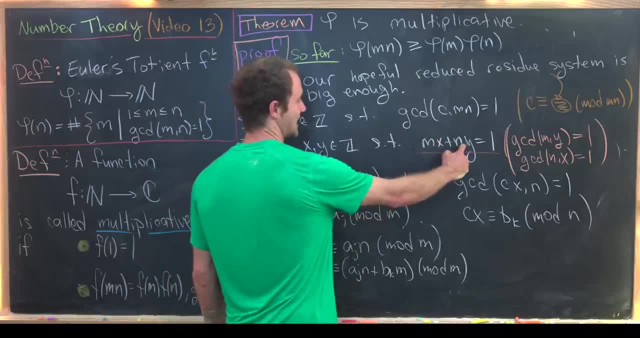 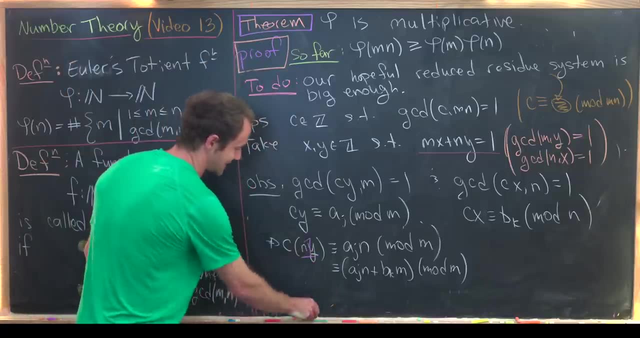 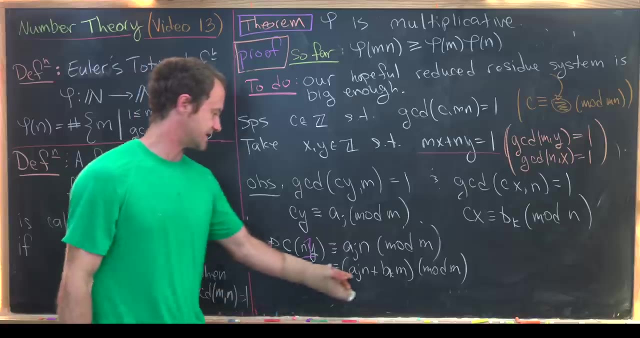 So this bit will go to 0 and we'll have N times Y is congruent to 1 mod M. So that means this: N times Y multiplies down just to the number 1,. well, mod M and we're left with C is congruent to this AJN plus BKM mod M. 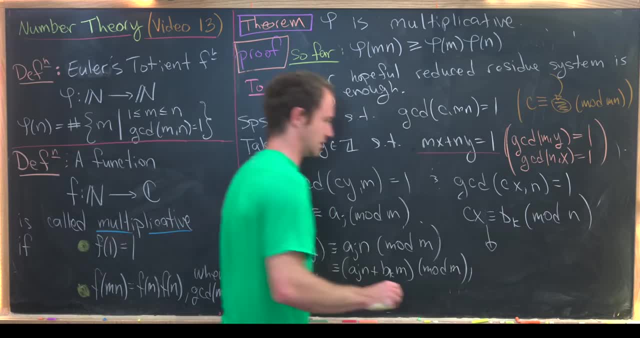 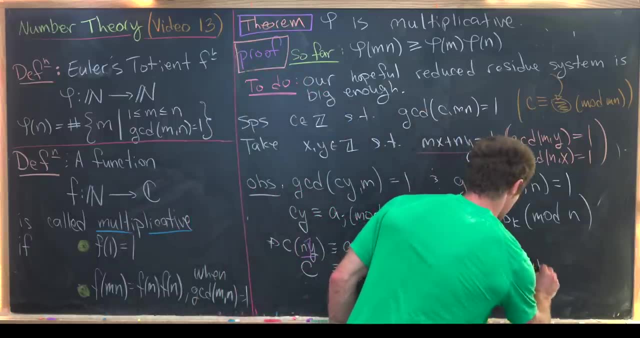 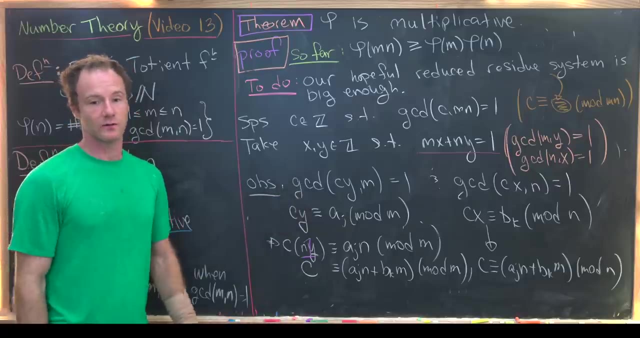 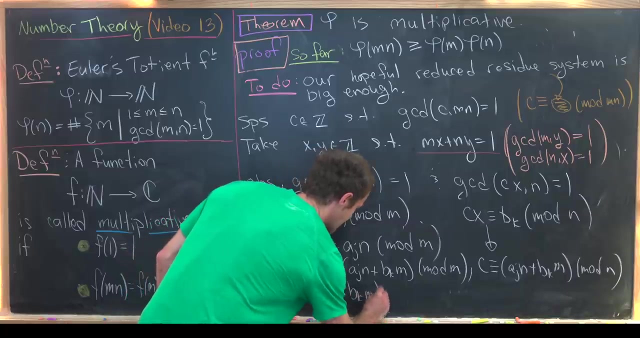 And then, through a very similar or in some ways a parallel argument, we get: C is congruent to the same thing, AJN plus BKM mod N. But since M and N are relatively prime, that tells us that C is congruent to AJN plus BKM mod M N. 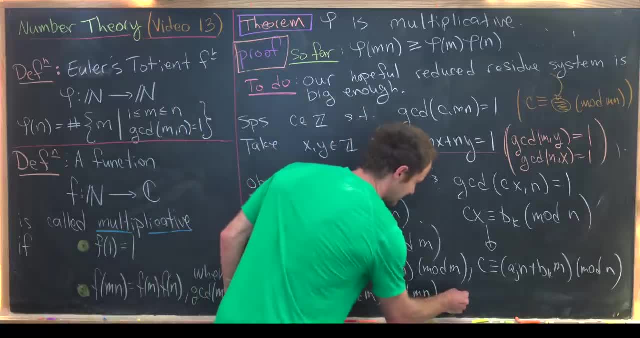 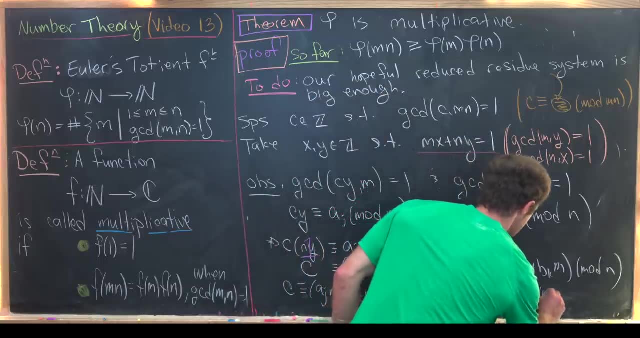 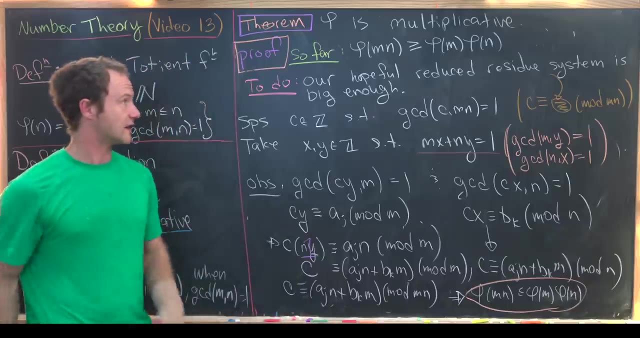 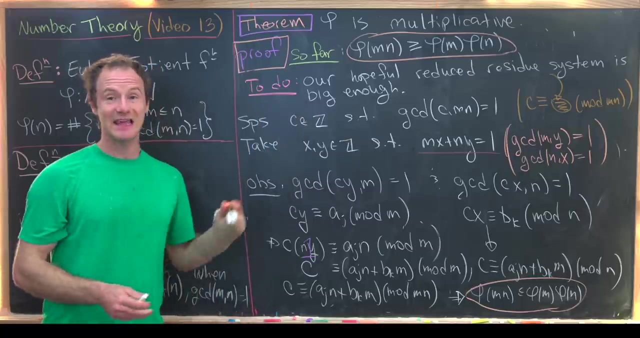 But that tells us our reduced residue system is in fact big enough. So in other words, we have. But now, combining this inequality which I've just circled down there, together with our inequality from the first half of the proof, we see that phi of mn is equal to phi of m times phi of n, which is exactly what we needed to show. 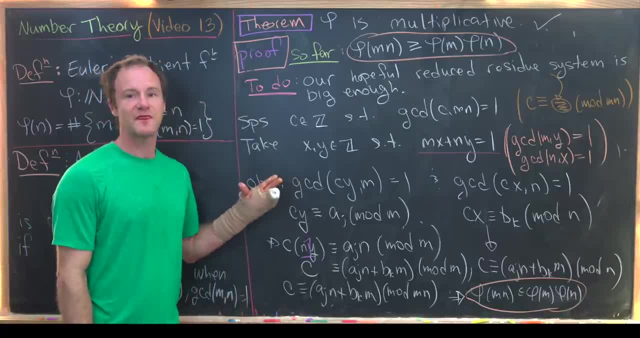 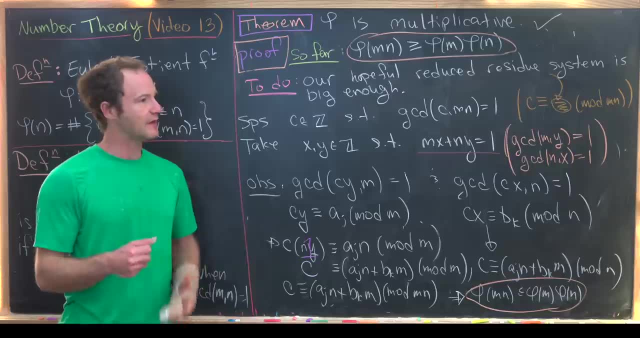 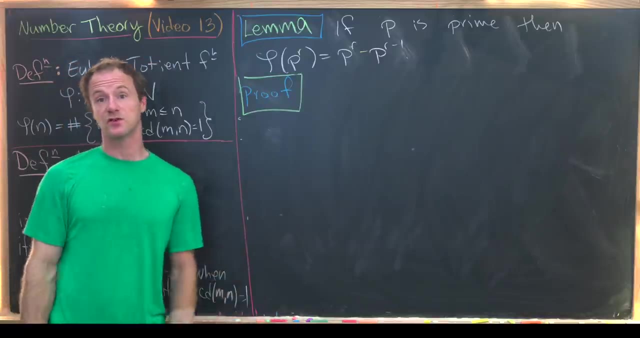 for phi to be multiplicative. Okay, so now that we've got this in place, we need to prove a limit involving the value of phi at a power of a prime, and then we're pretty much good to have a formula for our function phi. Okay, we just got done proving that our function phi Euler's totient. 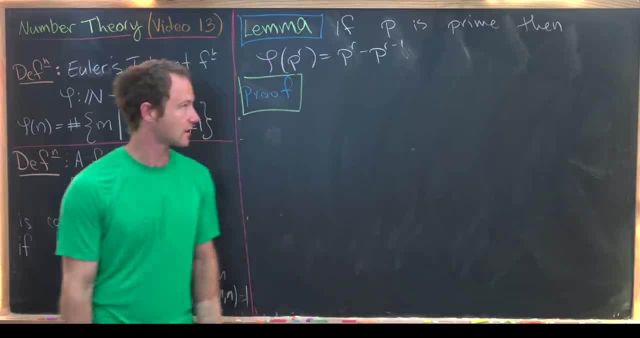 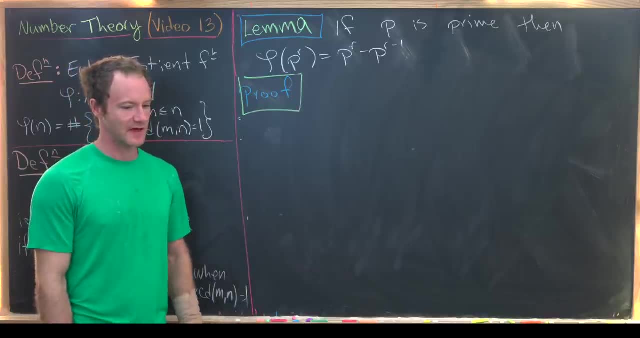 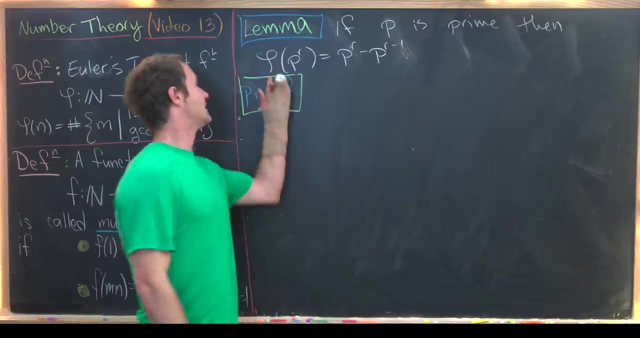 function is indeed multiplicative by this definition down here. Now we want to see the value of phi at a power of a prime. That'll give us a nice calculational method for calculating phi at some like randomly given number. Okay, so if p is prime, then phi of p to the r is equal to p to. 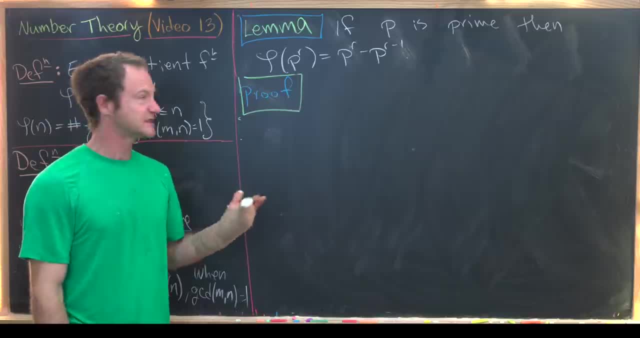 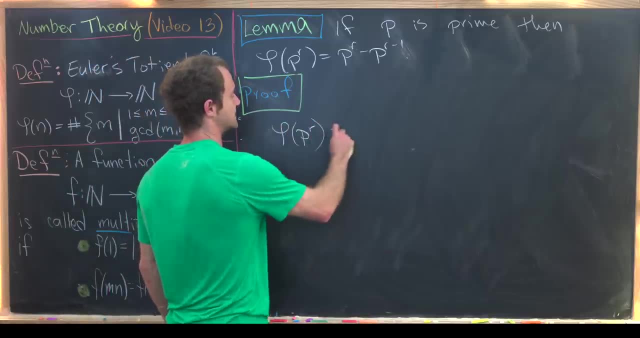 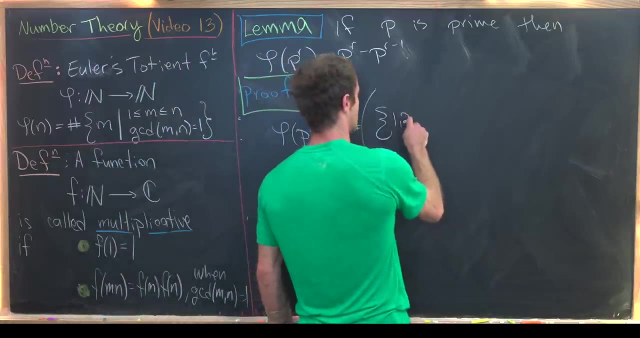 the r minus p to the r minus one. And this proof is a lot shorter than what we just saw. And we can start by noticing that phi of p to the r is equal to the number of elements in the difference of the following sets: So one, two. 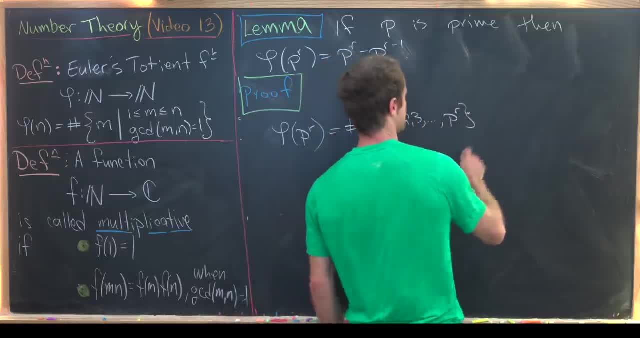 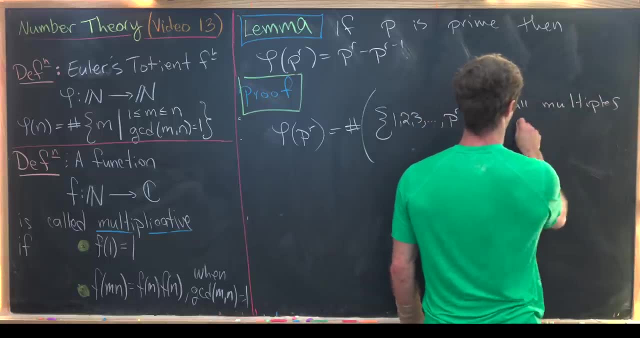 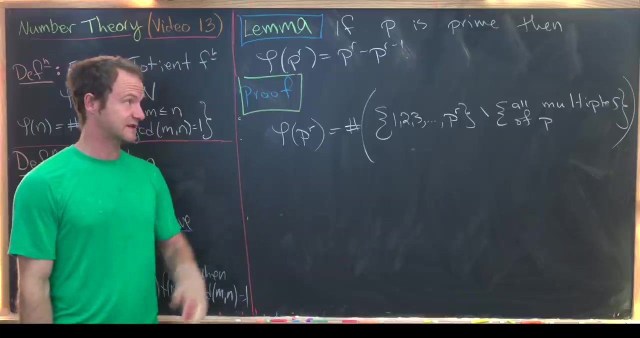 three all the way up to p to the r, minus all multiples of p. Well, recall that we want to count up all of the numbers that are relatively prime to p to the r, but the only thing that's not a relatively prime to p to the r are multiples of p. So that's kind of how. 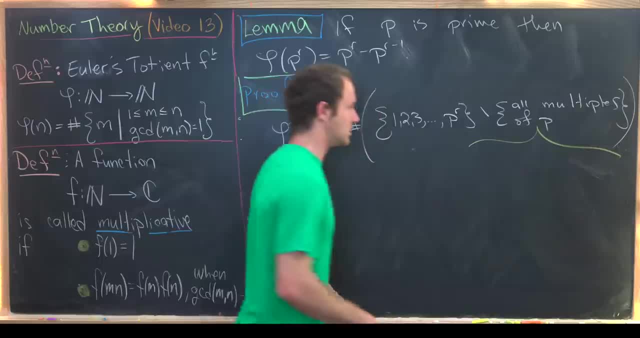 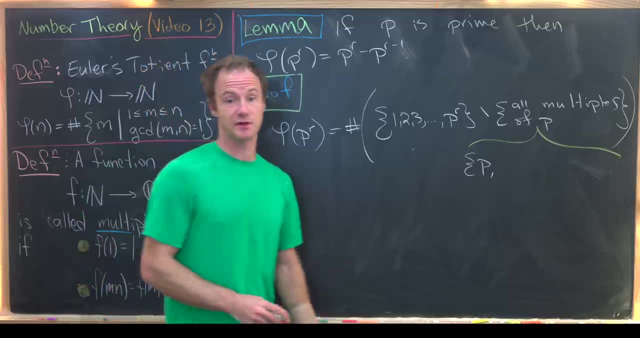 that settles out. So now let's count up all multiples of p. That shouldn't be too hard. So notice, we've got one times p. That's most definitely a multiple of p. We've got two times p, three times p, all the way up to. 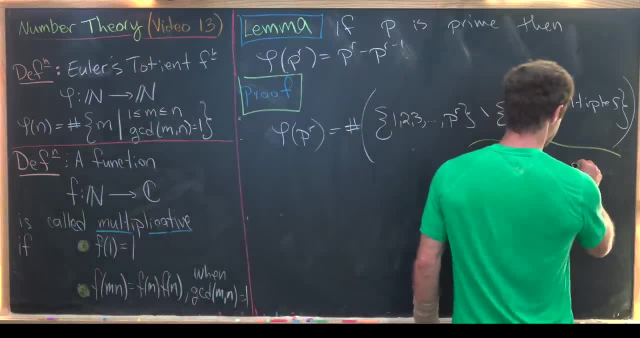 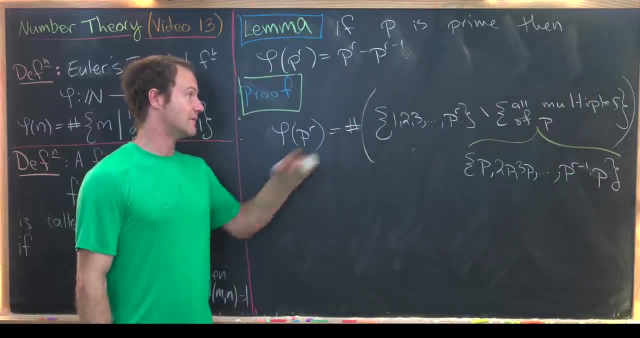 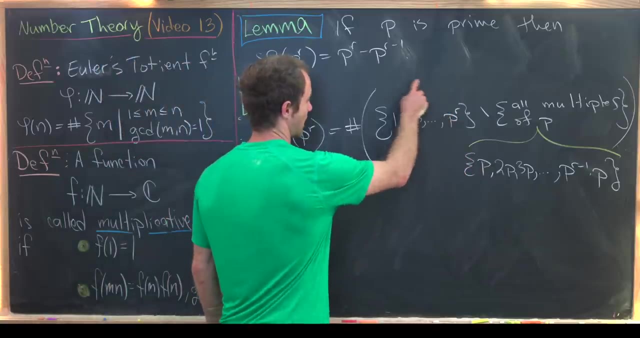 two. The last multiple of p will be p to the r minus one times p. So now we're good to go. We need to find the number of elements in this set minus this set, which is a subset of the original set. So here we have. there are obviously p to the r elements. 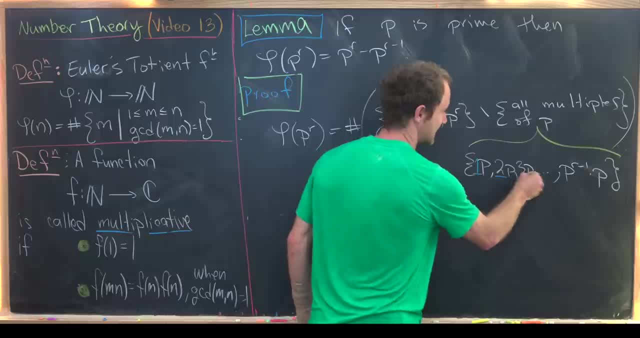 in this first set, And then the elements of the second set can be counted by the coefficients of p, by the coefficients of p. So there are p to the r elements in this número 2 set and then the 1st piece in the La Re eller Bq. dumplings. So if these are also a part of the set, we are able to calculate a derivative coefficient or an infinite transformation for each set of elements of p. Зions can also be calculated automatically by determining the expressions of the elements. So what we do here is we try to find the elements of theRAY candidate to be dari alien to the right. 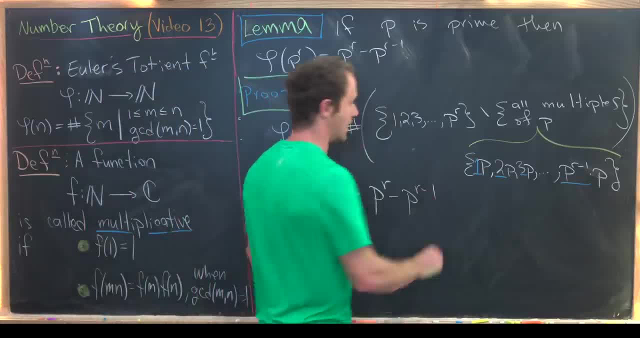 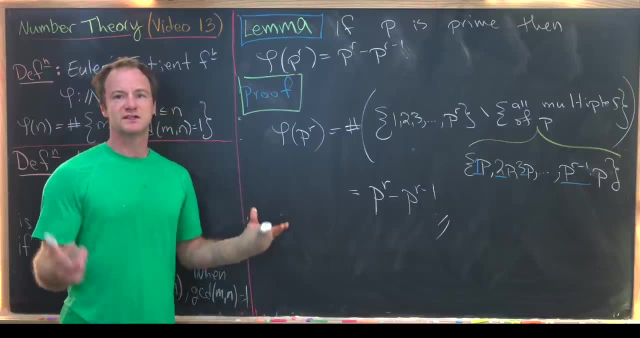 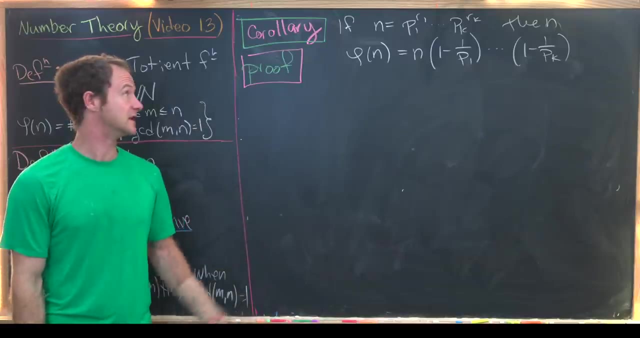 so there are p to the r minus 1 elements in that second set, and that finishes the proof of this lemma. okay, so now let's smash that last theorem and this lemma together into a nice formula for phi. okay, so this is the punch line of this video, and that is the following corollary. so if we've 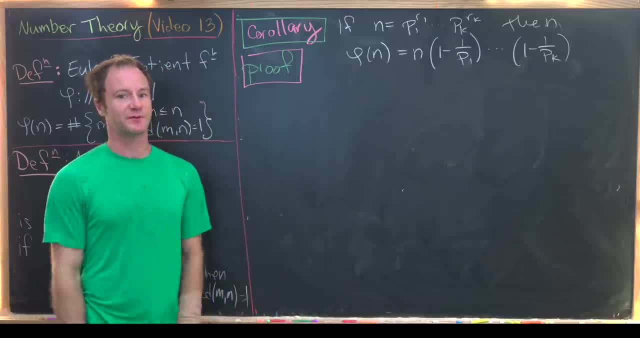 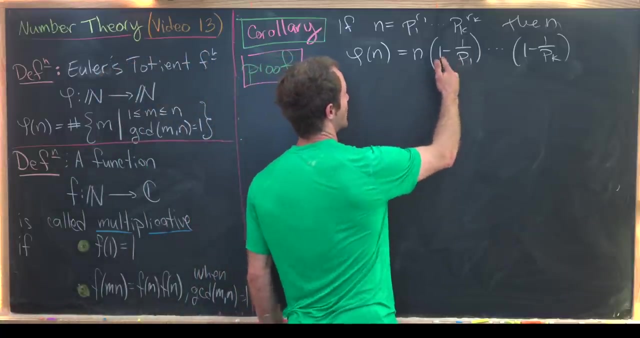 got a prime factorization of n, which we know is possible by the fundamental theorem of arithmetic, and that prime factorization is p 1 to the r 1, all the way up to p k, to the r k, where all of the p's are distinct primes. then phi, evaluated at n, is n times 1 minus 1 over p. 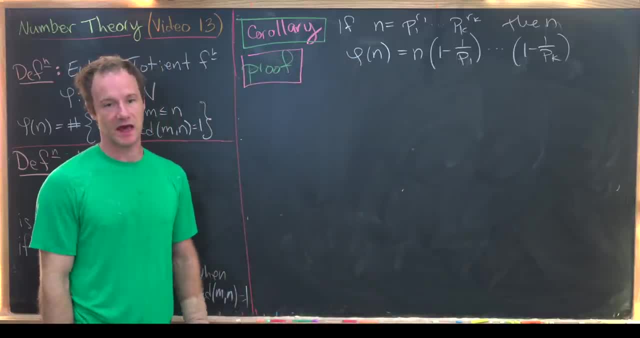 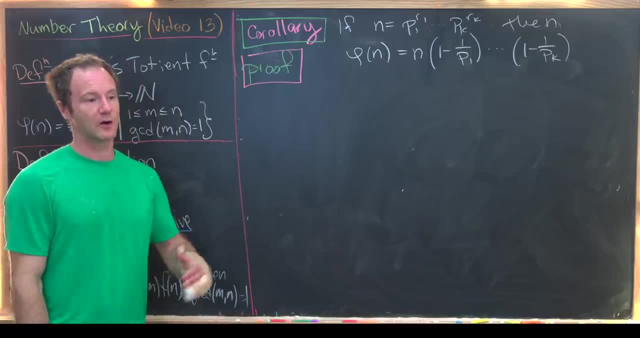 all the way down to 1 minus 1 over p k. okay, so let's see the proof of this, which is actually fairly calculational and quick now that we've got our previous theorem and that corollary. so let's notice that phi of n. 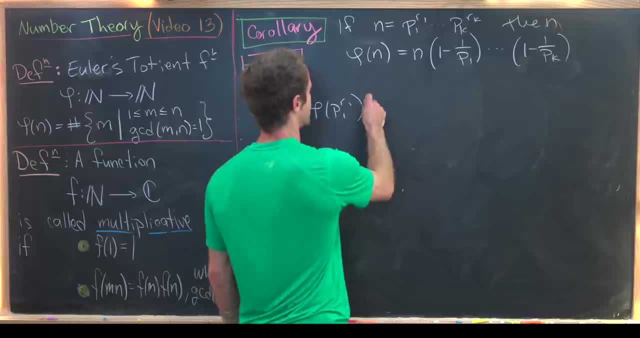 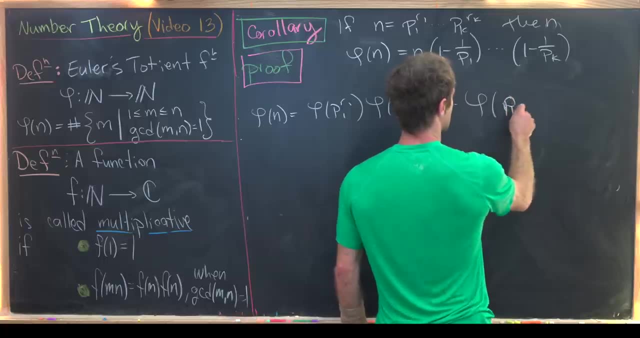 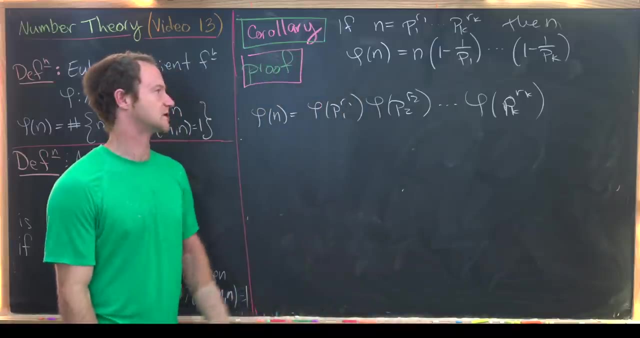 that's lights up, can first be written as: phi of p1 to the r1, times phi of p2 to the r2, all the way up to phi, of pk to the rk, And that's by the multiplicativity of our function phi. All of those primes are: 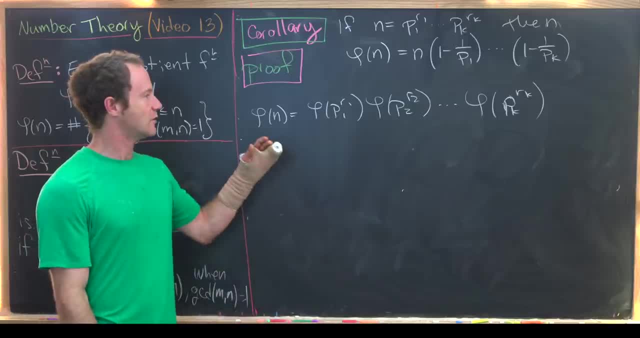 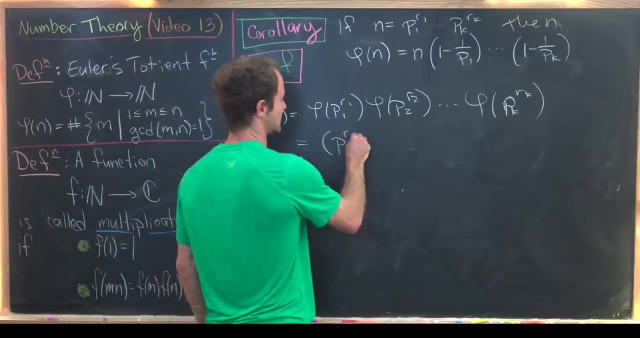 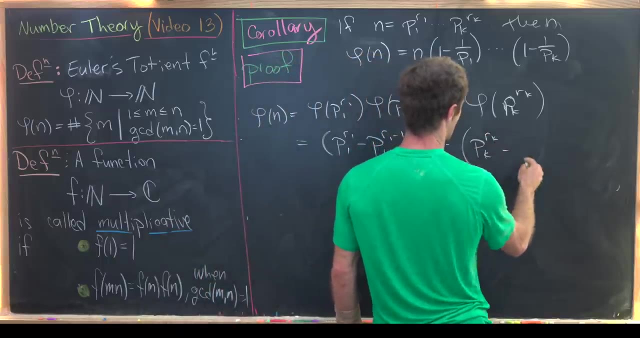 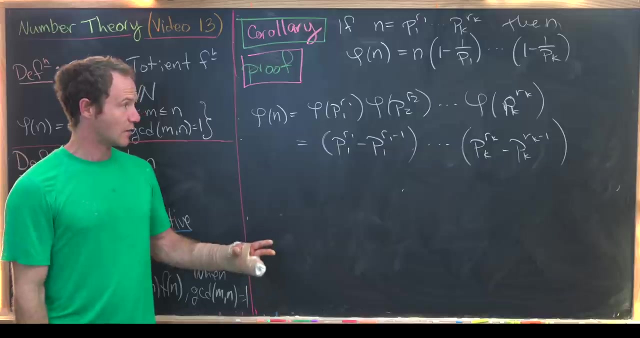 clearly relatively prime to each other. Now we can apply our prime power formula to each of these. So notice this guy right here- will be p1 to the r1 minus p1 to the r1 minus 1, all the way up to pk to the rk minus pk to the rk minus 1.. Again, that's by our previous lemma. Now what I'll do. 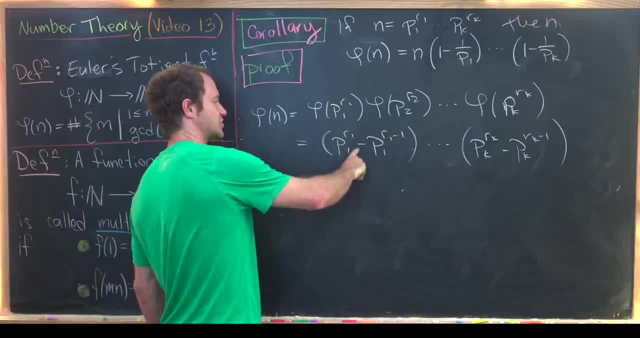 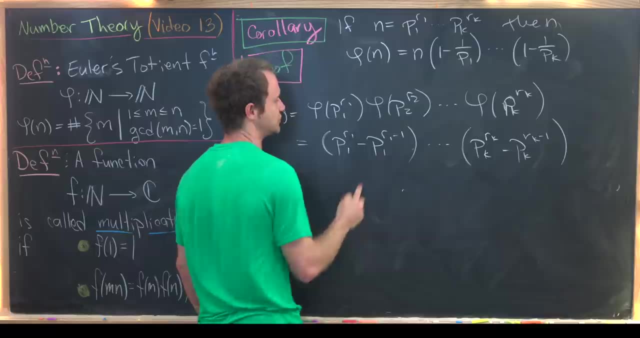 is factor, the first term out of each of these binomials. So I'll factor a p1 to the r1 out of this one, a p2 to the r2 out of this one and finally a p2 to the r1 out of this one, And 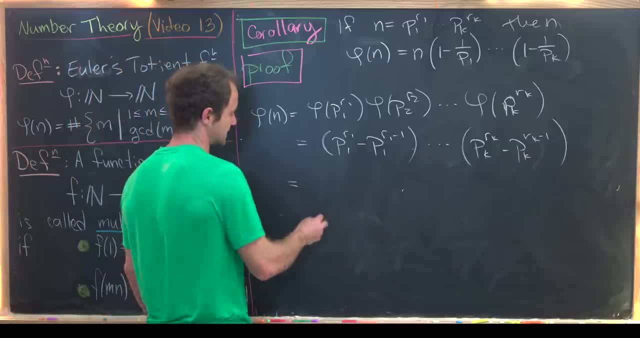 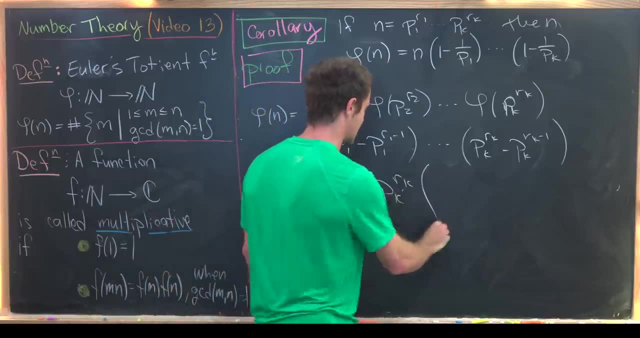 pk to the rk out of the last one. That's going to leave me with a p1 to the r1, p2 to the r2, all the way up to pk to the rk. in front of the whole thing. Then let's see what's left over. 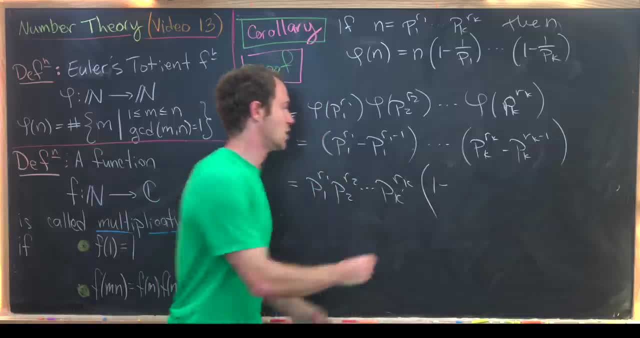 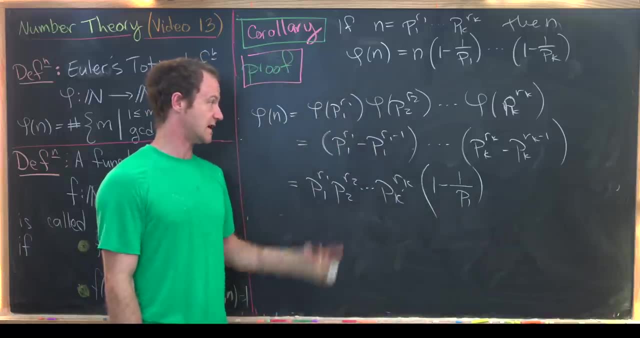 So here we'll be left with 1 minus 1 over p1.. Well, why is it 1 over p1? Because we have one less power of p1 here than we factored out, And then the next term will be 1 minus 1 over p2,. 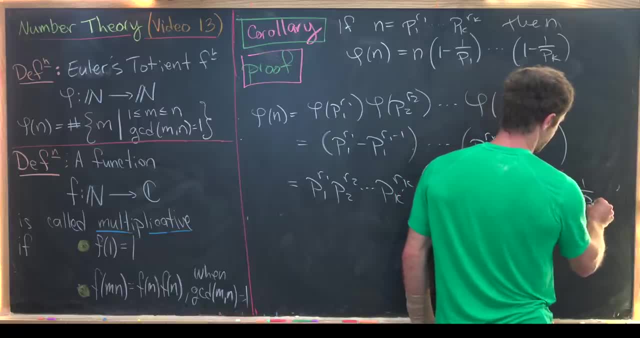 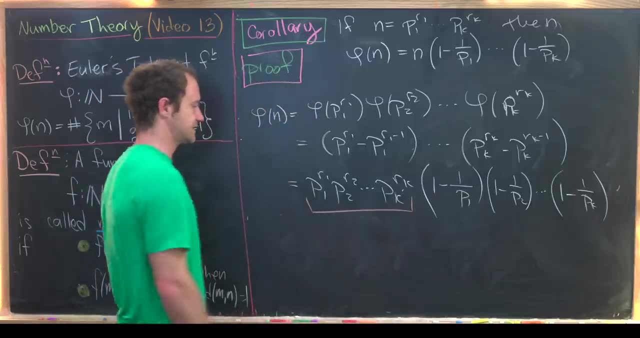 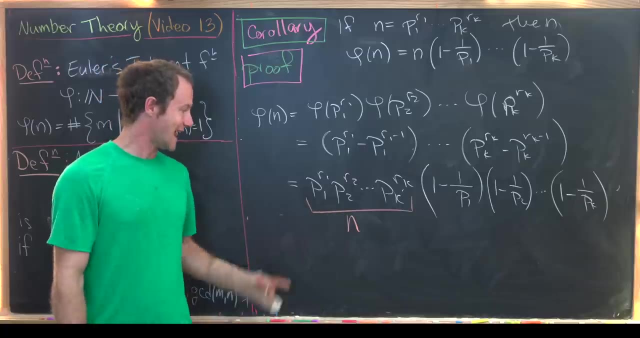 all the way up. The last term will be 1 over 1 minus pk, like that. But now we're in luck because- notice, these numbers represent exactly the factorization of our number n. So we can just smash all those together to get n And we've got n times that product over there, which is exactly. 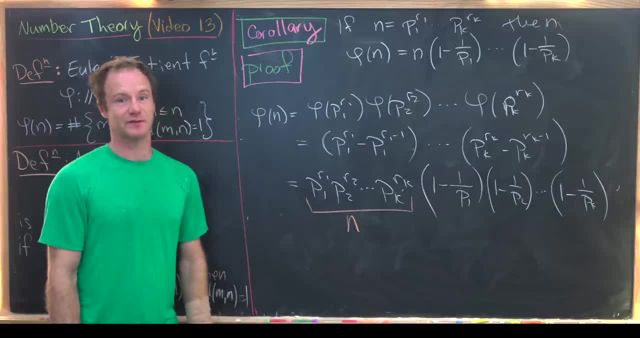 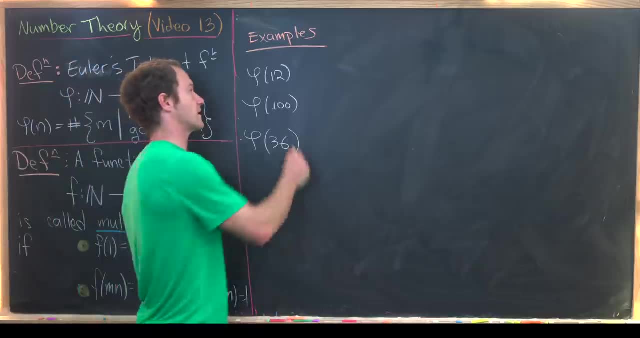 what we wanted to show. Okay, so now let's do some examples. Okay, so let's do some fairly quick examples. So let's first calculate the number of times that we've got. So let's do some fairly quick examples. So let's first calculate phi of 12 using our formula. So we know that this is 12. 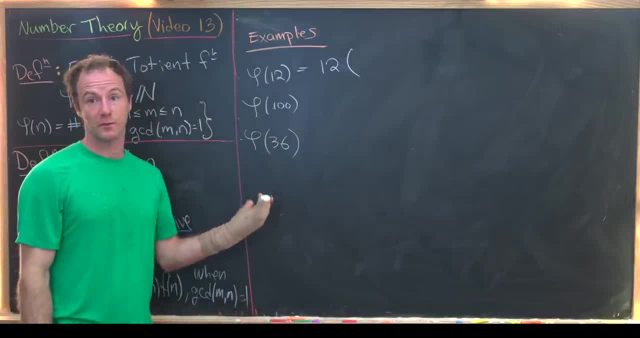 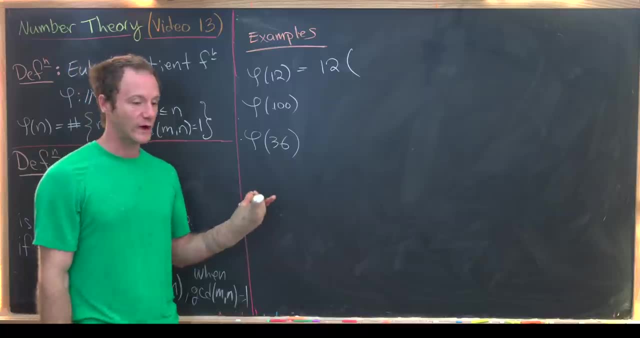 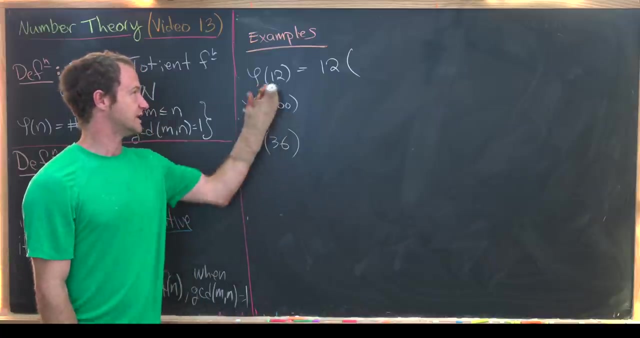 times 1 minus 1 over the primes that divide into 12.. Notice, we don't even really need to know the prime factorization. We only really need to know which primes divide into this. We don't need their exponents by that trick of the formula that we saw before. So we know 12 is divisible by 2 and 3.. 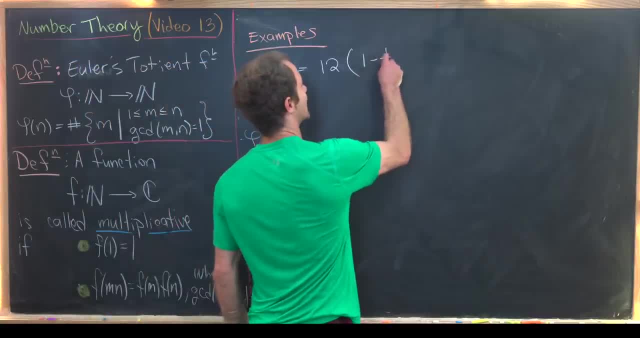 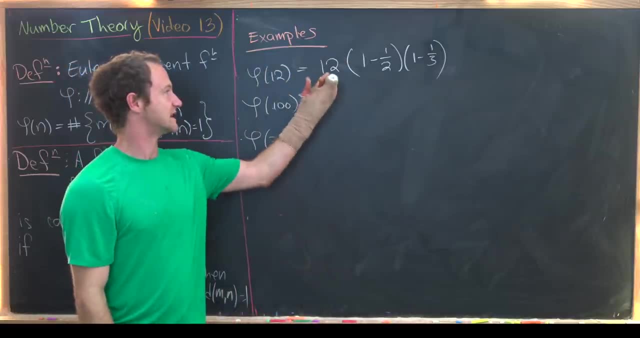 Those are the only primes that divide into it. So this should be 1 minus half and then 1 minus 1.. So we know that this is 12 times 1 minus 1 over the primes that divide into 12.. And we were right. We shouldn't really have pi minus third like that. But notice that's going to. 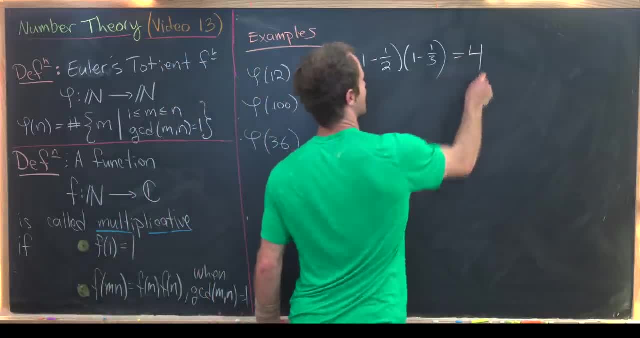 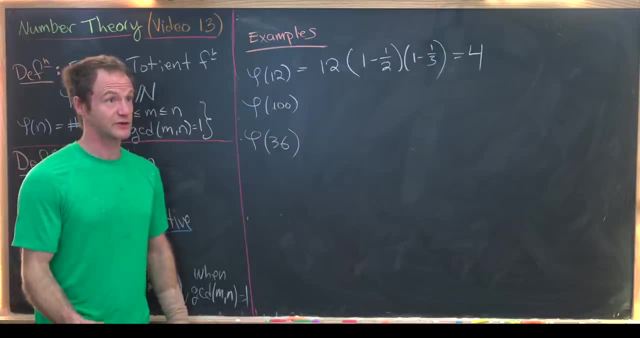 give us 12 times half times 2 thirds. I'll let you guys multiply that out and see that you get the number 4, which checks out, because the only numbers between 1 and 12 that are relatively prime to 12 are 1, let's see 5,, 7, and 11.. Okay, so now let's do phi of 100.. We'll get 100.. 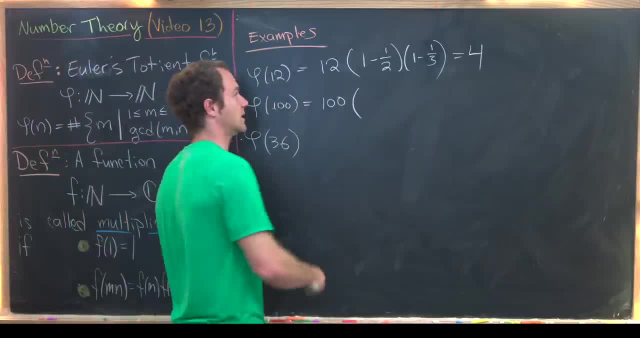 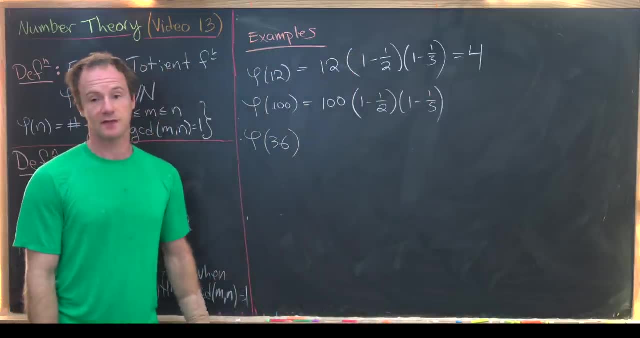 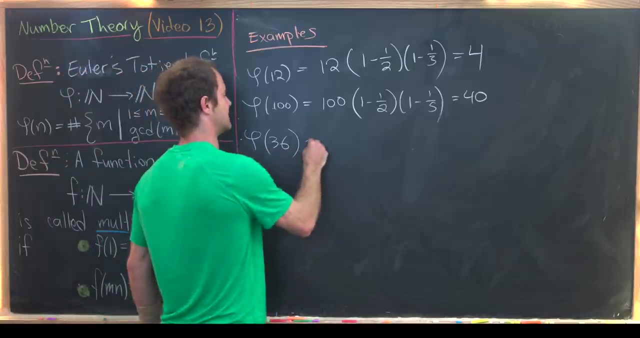 And then 2 and 5 are the only primes that divide into 100. So got 1 minus half and then 1 minus fifth. So again, that's a fairly elementary arithmetic problem and you'll see that we get the number 40. Then, finally, phi of 36, that's going to be equal to 36: 1 minus. 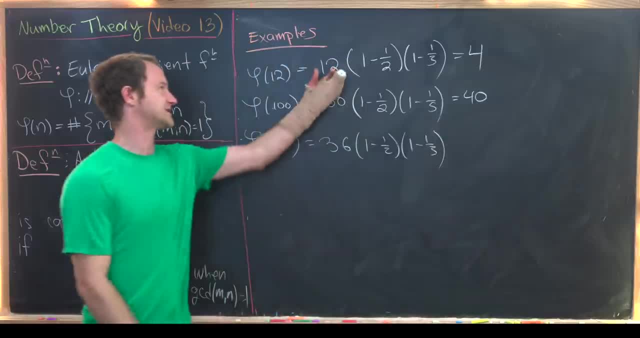 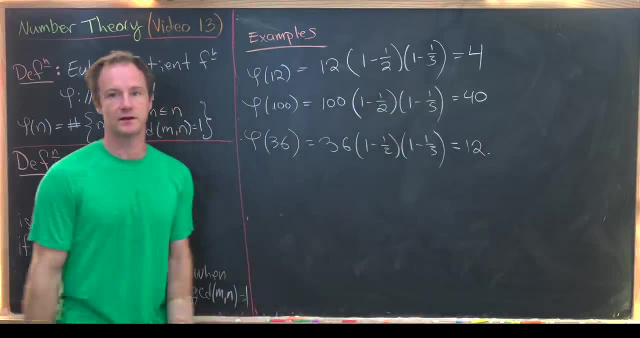 half and 1 minus third, pretty much for the same reason as we had up here. Those are the only primes that divide into that and that gives us the number 12 in the end. Okay, so let's do one more example before we present some warm-up problems. Okay, so now we're going to do a little. 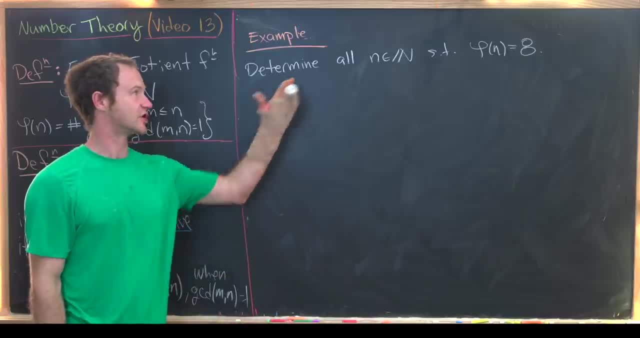 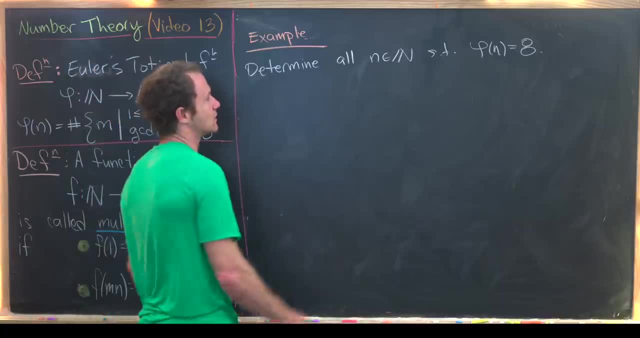 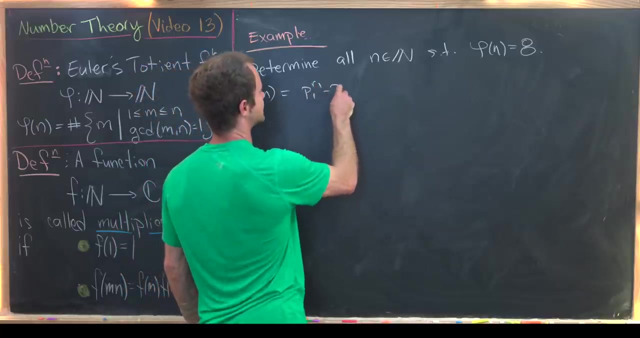 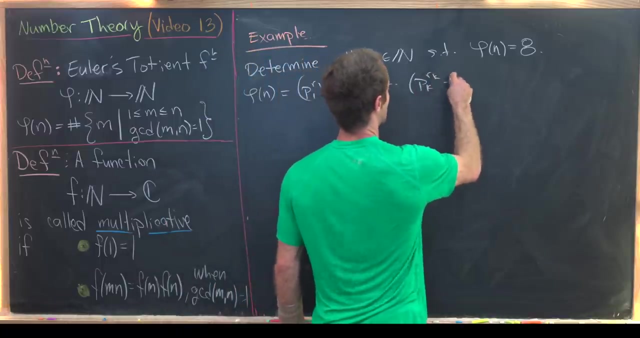 bit bigger of an example. So our goal is to determine all natural numbers, n, such that phi of n equals the number 8.. Okay so let's first recall that our phi of n will give us p1 to the r1 minus p1 to the r1 minus 1, all the way up to pk to the rk minus. 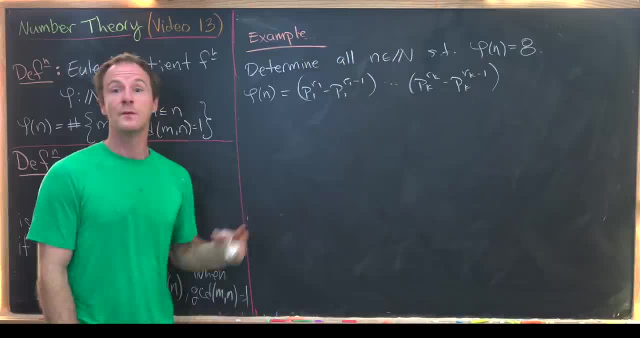 p1 to the r1 minus 1.. So we're going to do one more example before we present some warm-up problems: pk to the rk minus 1.. But now, instead of factoring this the way we did in the proof of our lemma, 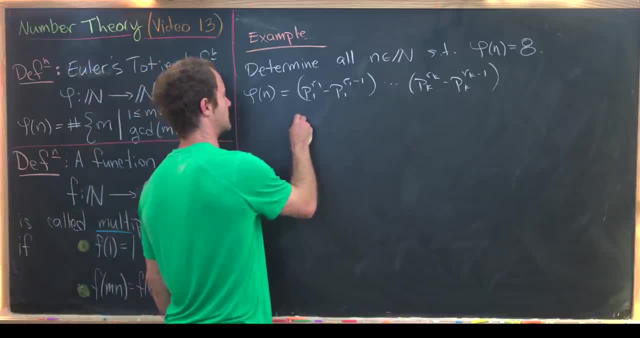 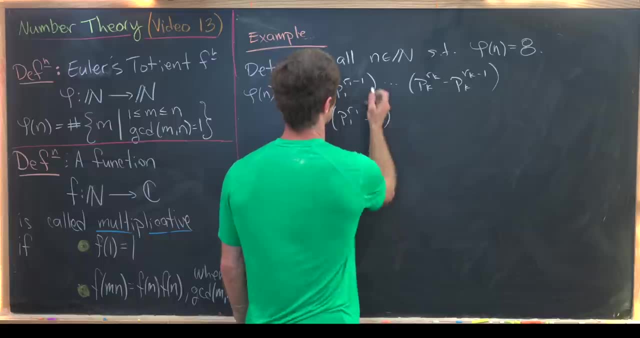 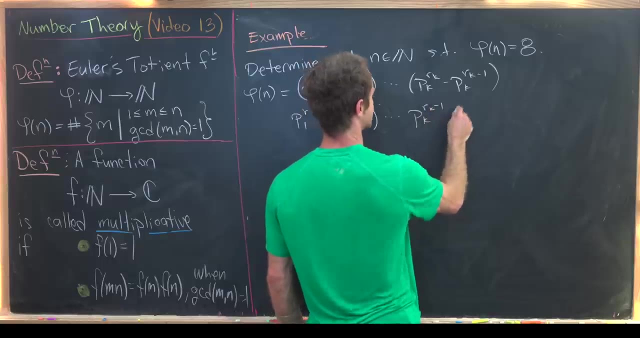 let's factor it a little bit differently. Let's factor this term out. So we've got p1 to the r1 minus 1 times p1, r1 minus times p1 minus 1, all the way up to pk to the rk minus 1 times pk minus 1.. 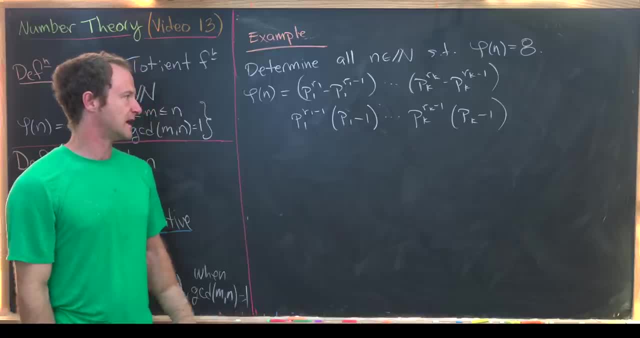 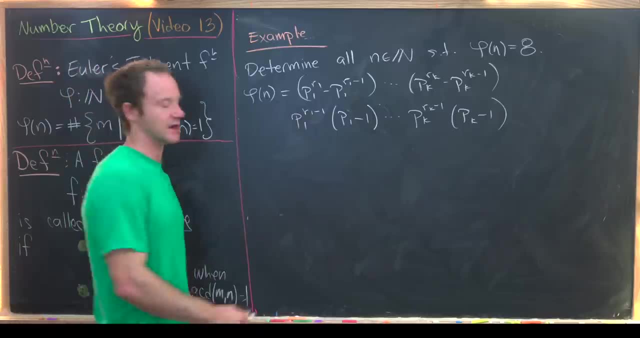 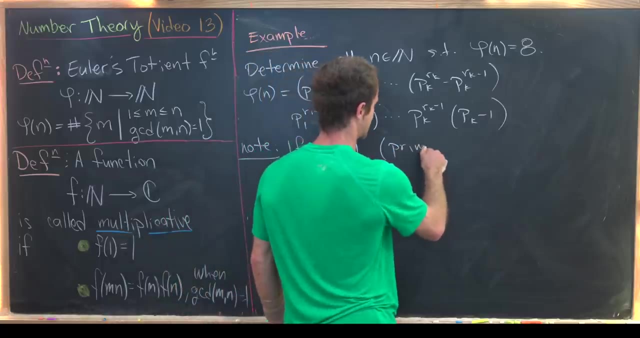 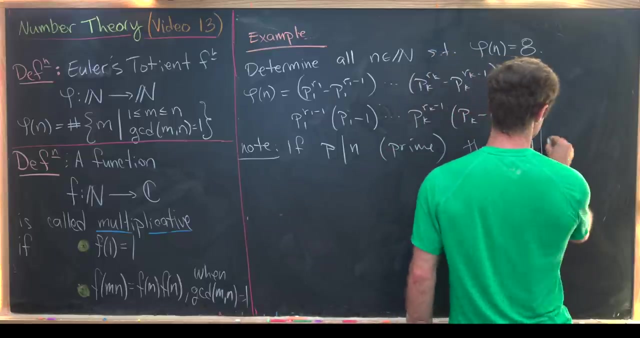 So the important takeaway here is that 1- less than all of the primes dividing n must divide phi of n. So maybe we'll put that as a note. So if p divides n and I should say p is a prime, then p minus 1 divides phi of n. Okay, but now we can look at some 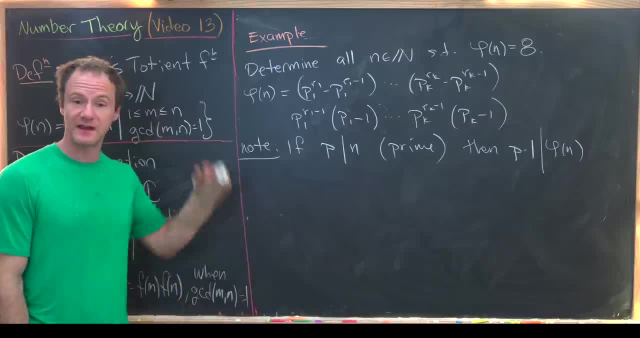 different ways of dividing phi of n. So we can look at some different ways of dividing phi of n. So we can look at some different ways of dividing phi of n. So we can look at some different divisors of 8.. Remember, our goal is for phi of n to be 8.. So if p minus 1 divides phi of n, 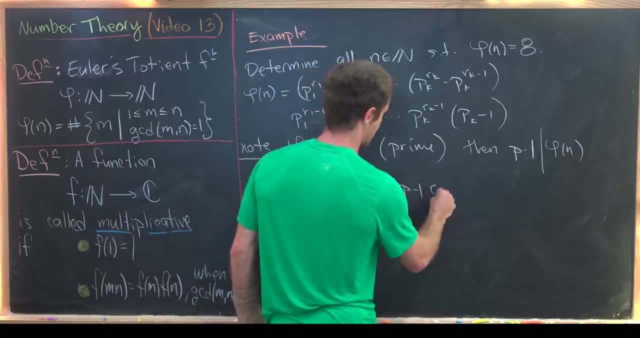 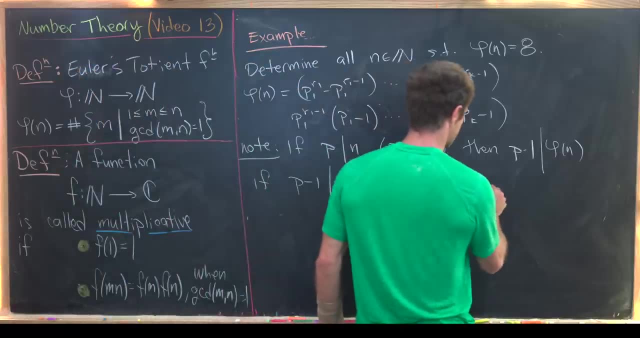 which is 8,. then that means p minus 1 comes from a fairly small set. There are only so many divisors of 8. So it comes from the set 1,, 2,, 4,, 8.. Again, those are all the divisors of 8.. But that tells. 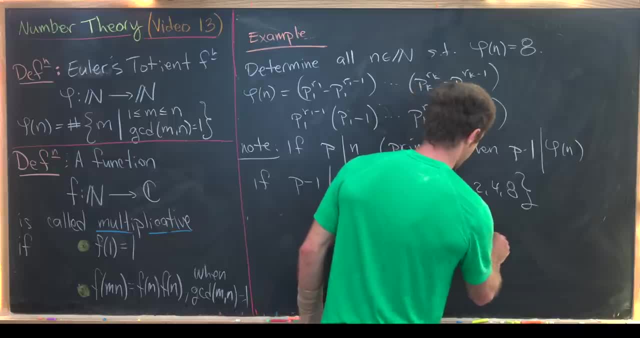 us that p comes from the set 2,, 3,, 5,, 6,, 7,, 8,, 9,, 10,, 11,, 12,, 13,, 14,, 15,, 16,, 17,, 18,, 19,, 20,, 21,. 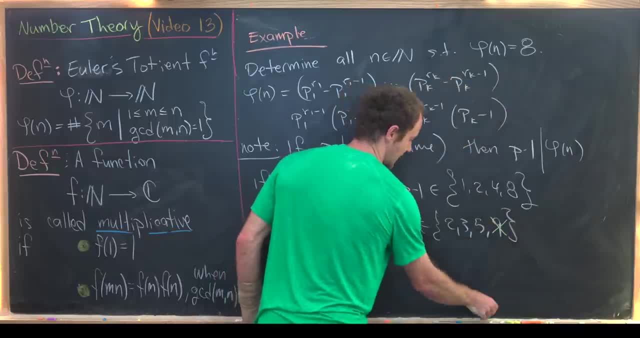 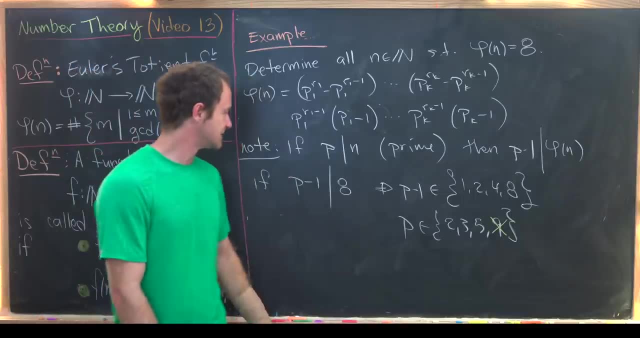 22,, 23,, 24,, 25,, 27,, 28,, 29,, 30. So if we divide phi of n by 2, then we get phi of n. So we can look at some different ways of dividing phi of n. Okay, so what does that tell us? That tells us that the 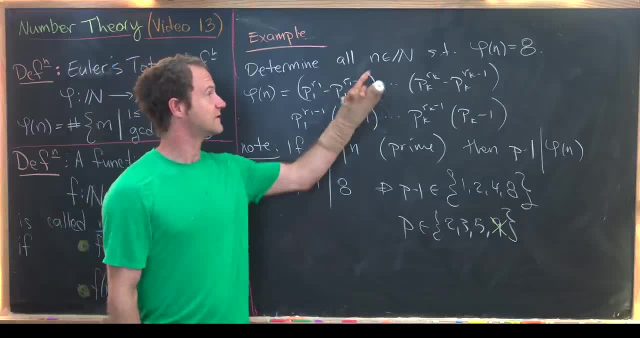 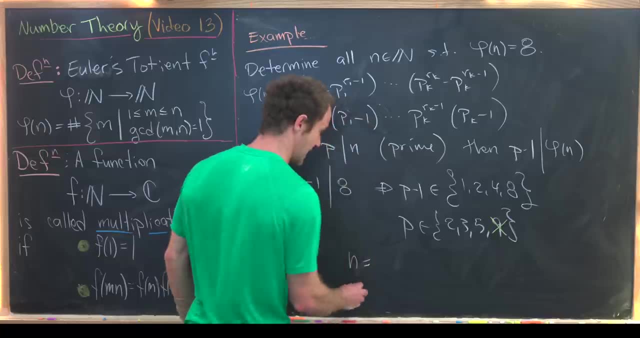 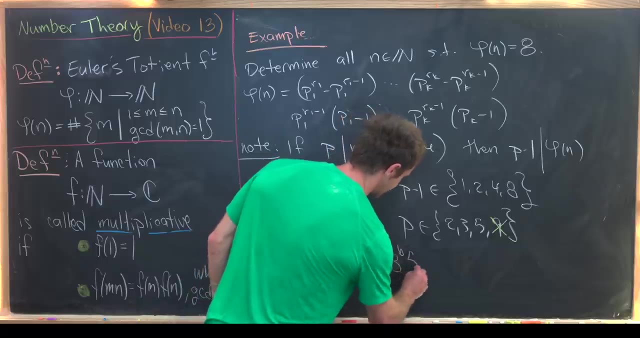 prime factorization of n that will achieve phi of n equals 8, only includes the numbers 2, 3, and 5.. In other words, our number n looks like 2 to the a times. let's see 3 to the b times 5. 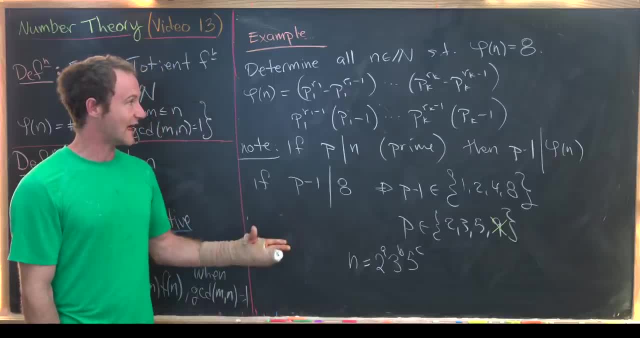 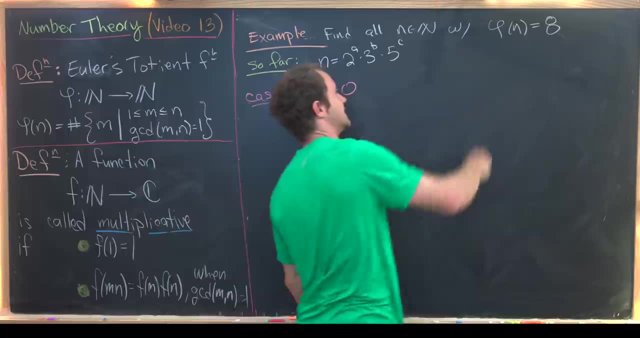 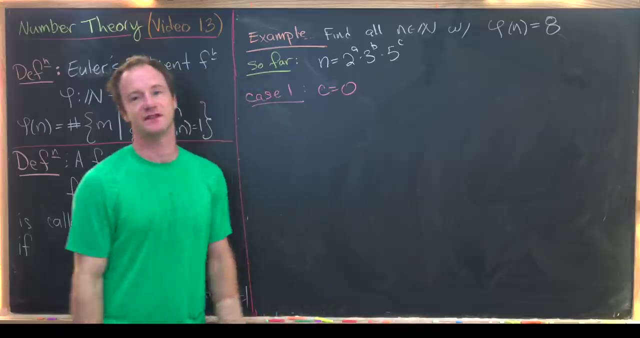 to the c. Okay, so now that we've figured that out, let's maybe bring that data to the top and then we'll move on. Okay, so our goal is to find all natural numbers in such that phi of n is equal to 8.. So far we've argued that n has to be the form 2 to the a, 3 to the b, 5 to the c, 2,, 3,. 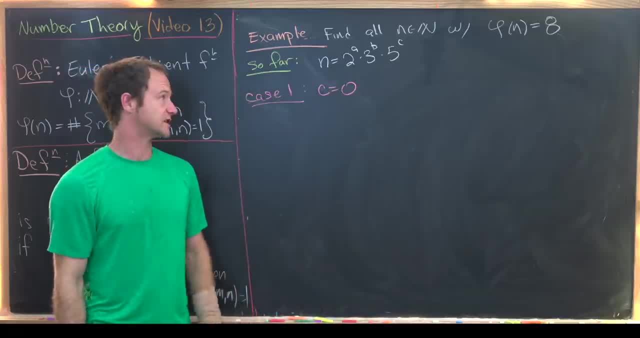 and 5 are the only possible prime factors of n. And now from here to the end. an end is not super fun, It's just a bunch of casework. But I want to point out that a lot of times math problems end up with a portion of the solution which is not fun, And maybe I shouldn't say not fun, but maybe. 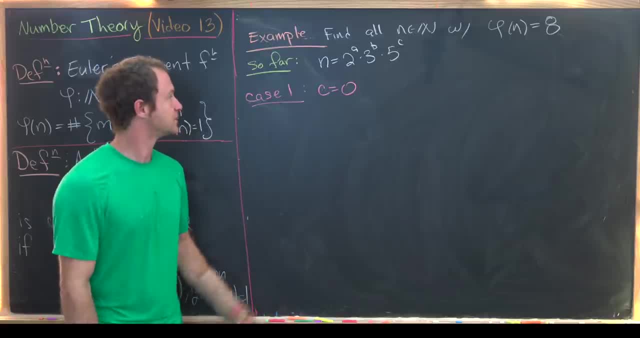 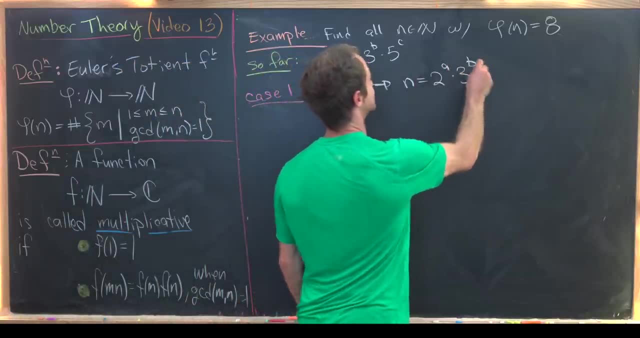 just a little bit tedious, And that's just part of the game. So our first case is that c is equal to 0. So, in other words, n is equal to 2 to the a times 3 to the b. Now, like I said, we're going to 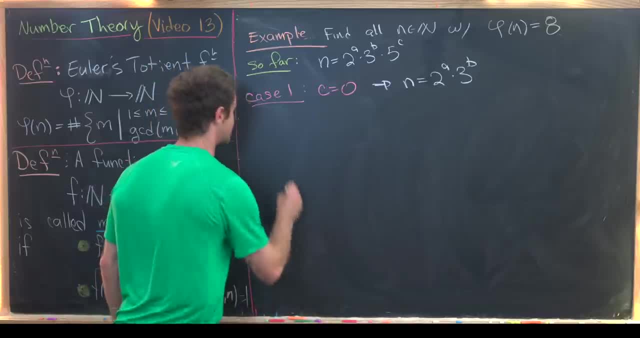 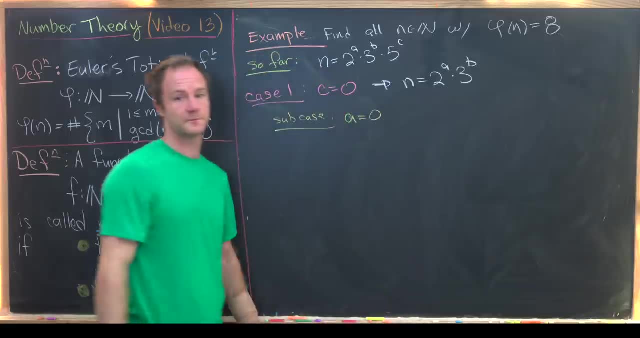 do casework, including the solution. So we're going to do casework including the solution. So we're going to do casework including the solution. So we're going to do casework including subcases. So let's do our first subcase, which will be: a equals 0.. So notice, if a is equal to 0,. 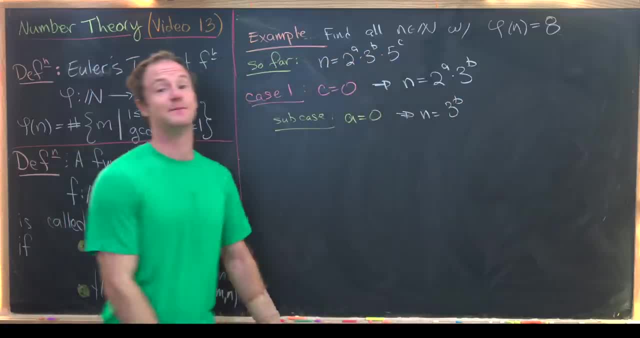 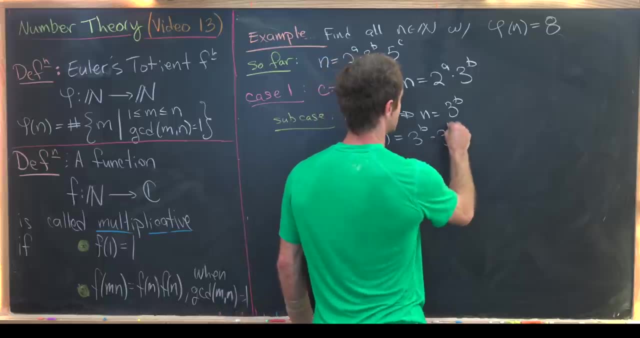 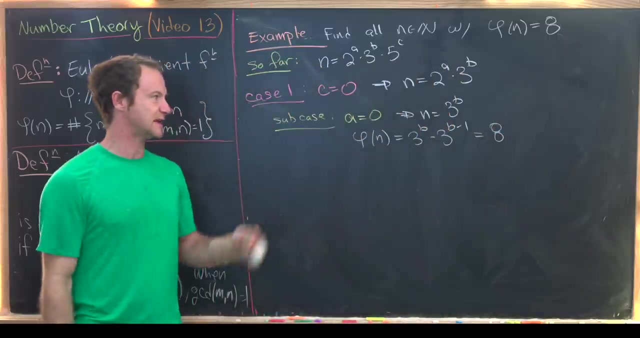 then that tells us that n is equal to 3 to the b, which tells us that phi of n is equal to 3 to the b minus 3 to the b minus 1.. And we want that to be equal to 8.. So 8 must be a different. 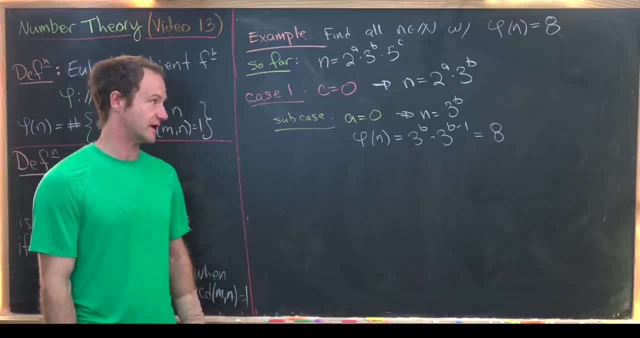 of 2, powers of 3. And those are consecutive powers of 3.. Now there are a couple of ways that you can figure out that that is impossible, But let's maybe just go ahead and factor out the 3 to the b. 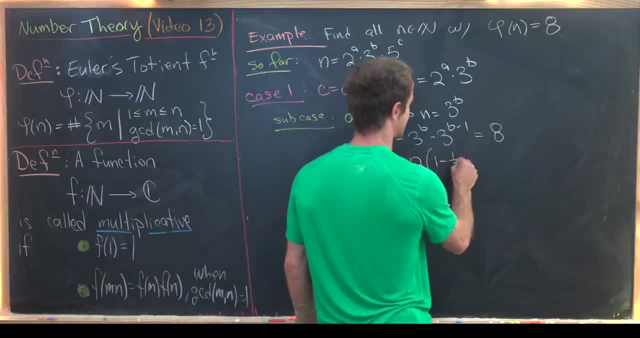 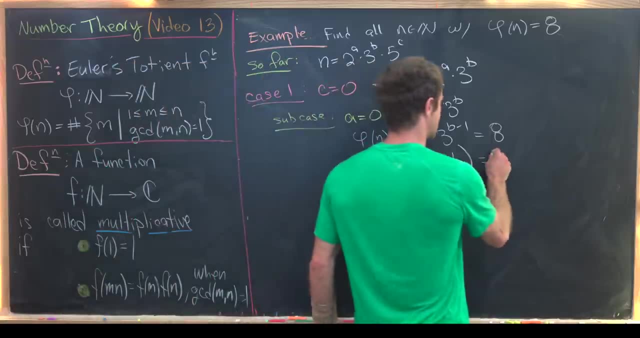 from this And notice that this is equal to n times 1 minus 1 third. So that's like also by our formula for phi of n. We need that to be equal to 8. But that tells us that 2 over 3. 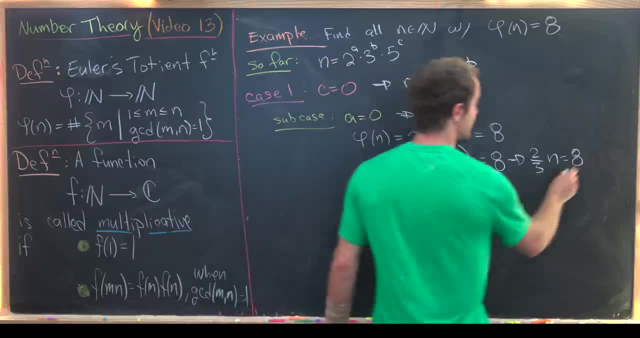 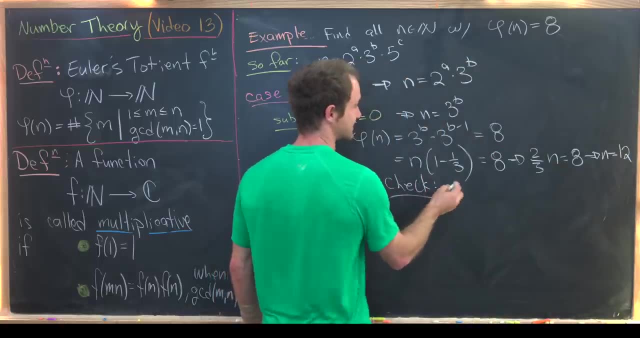 times n is equal to 8.. But notice that gives us that n is equal to 12.. But now, since all of this is all kind of funny business, we probably need to check. But phi of 12 is equal to 4,, which is: 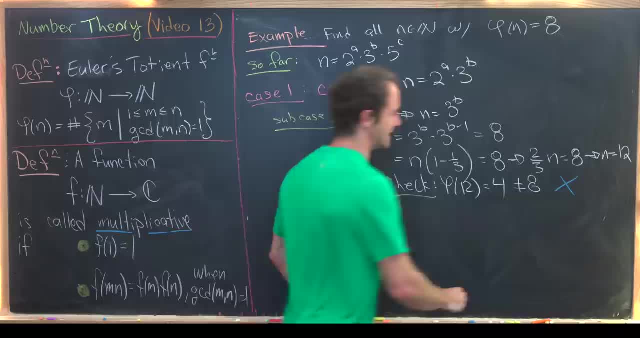 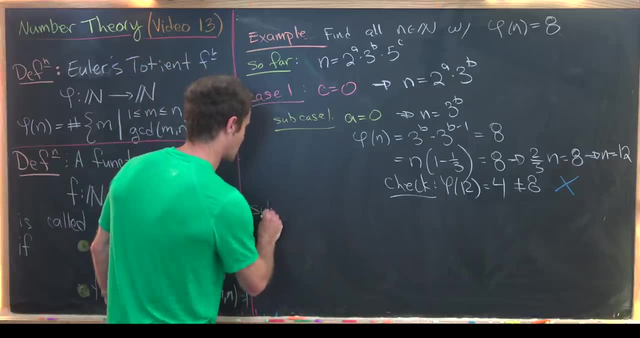 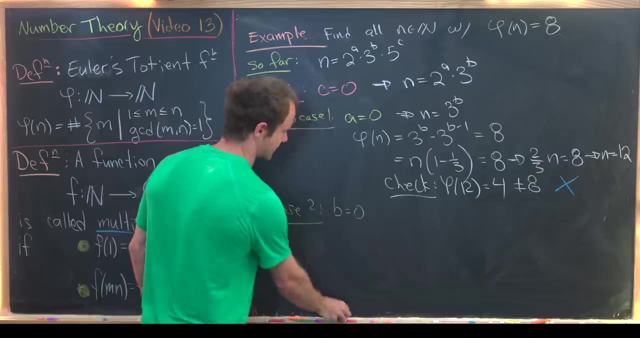 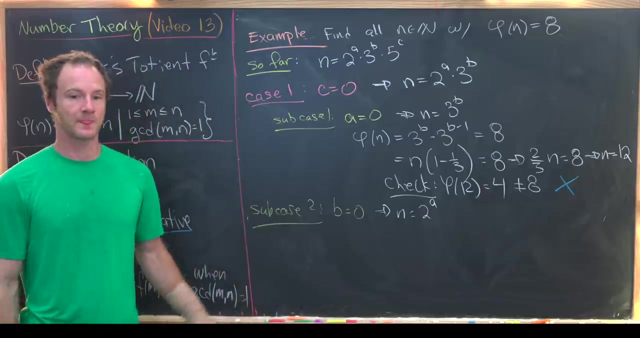 not equal to 8.. So that means we do not get a solution in that case. Okay. so now let's move on to our second subcase, So I'll call that subcase 2.. And that will be when b is equal to 0. So in other words, n is a power of 2. It's 2 to the a. Okay, so now we can do. 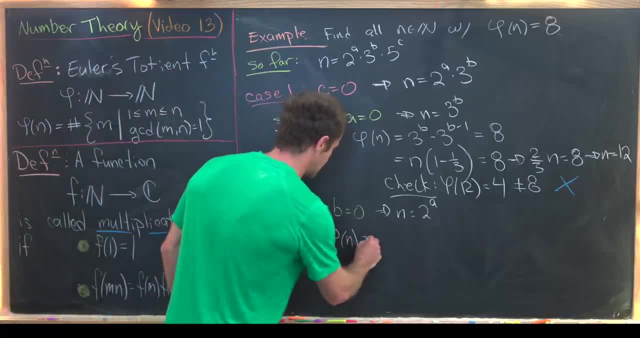 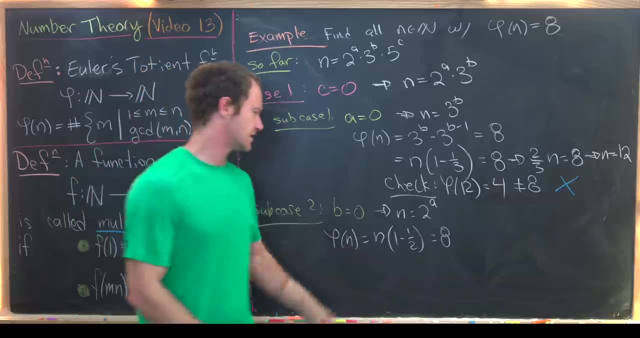 essentially the same thing that we did before. We know phi of n is equal to n times 1 minus half, but it's also equal to 8.. But notice that tells us that a half n is equal to 8.. Or in other words, 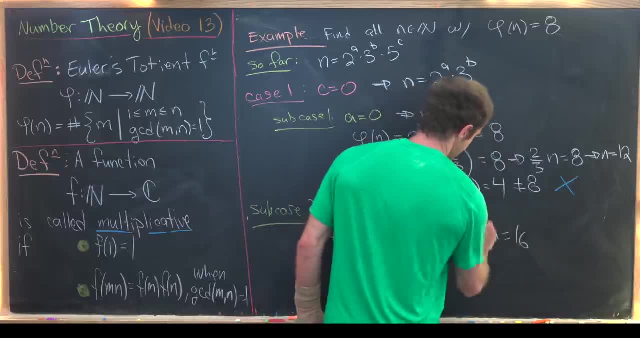 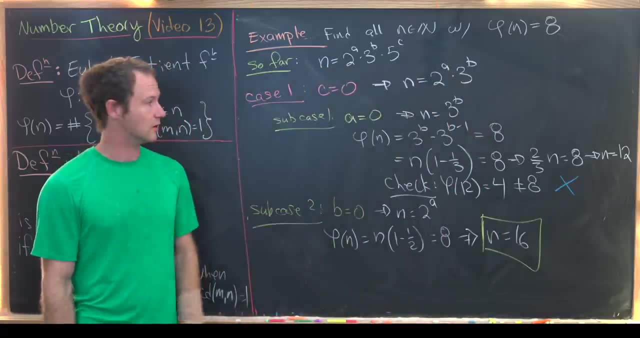 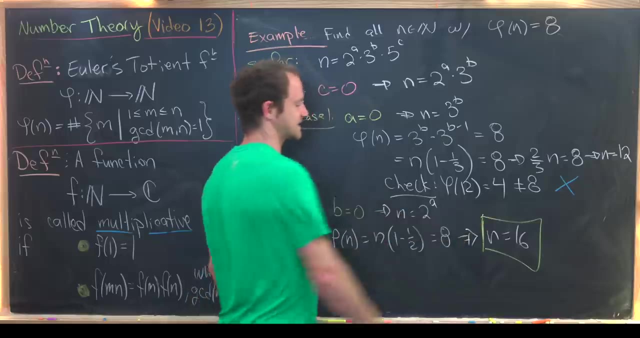 n is equal to 16.. But then Then you can check, using our formula for phi of n, that phi of 16 is good to go. Well, first of all, we see that our assumption really built into this was that n was a power of 2, but 16 is a power of. 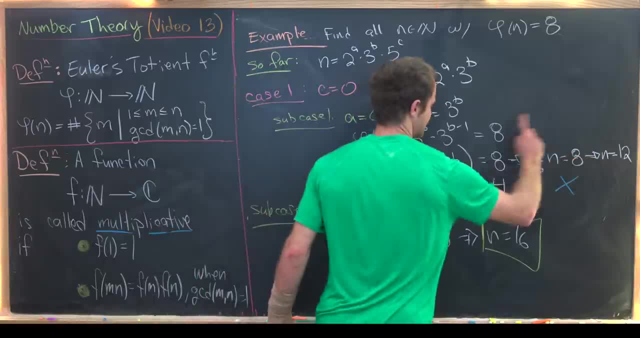 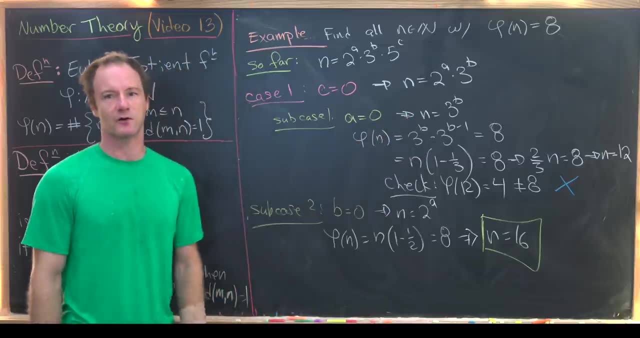 2,, which means we're good, Whereas over here this didn't work for a couple of reasons. but this says that n is 12, but our assumption was that n was a power of 3. And those are not conducive to each. 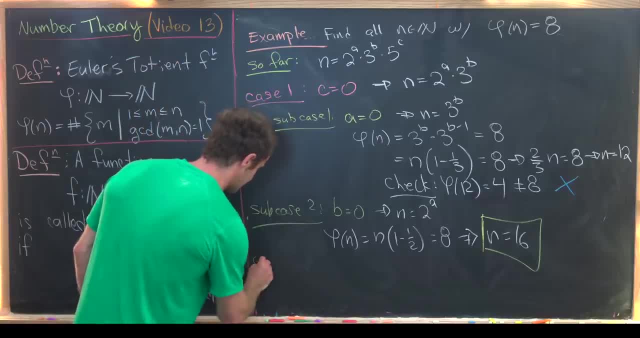 other. Okay, so now let's look at our next subcase. So we're going to look at our next subcase, So we're going to look at our third subcase, and that will be: neither of these are equal to 0.. 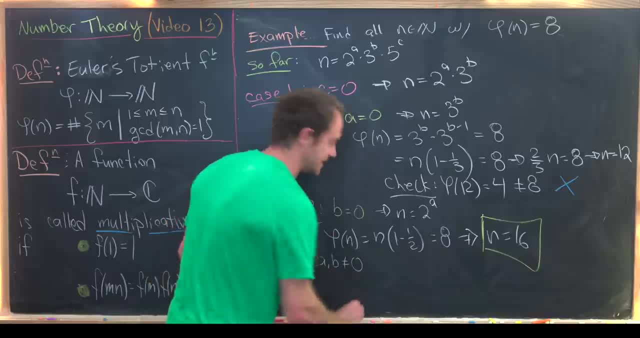 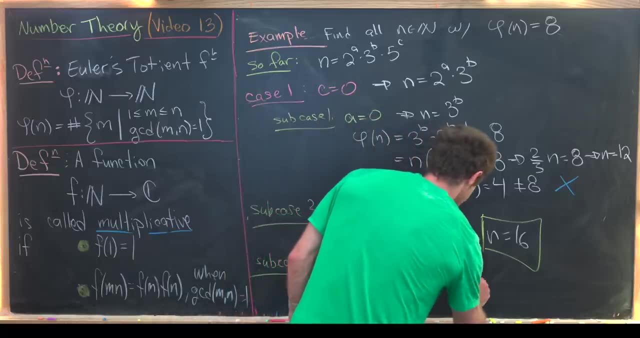 And so we've got a and b are non-zero. Okay, well, from there we've got that phi of n is equal to n times 1 minus half times 1 minus third. But let's see, that means that n over 3 is equal to 8.. 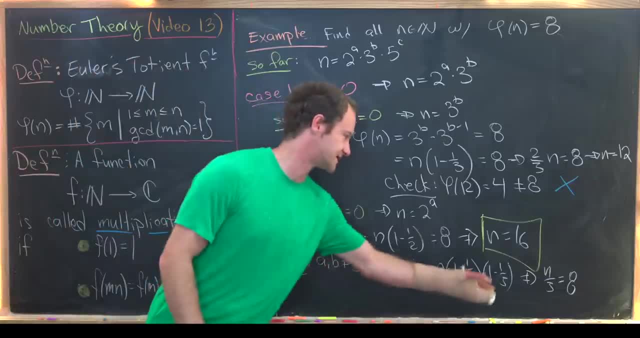 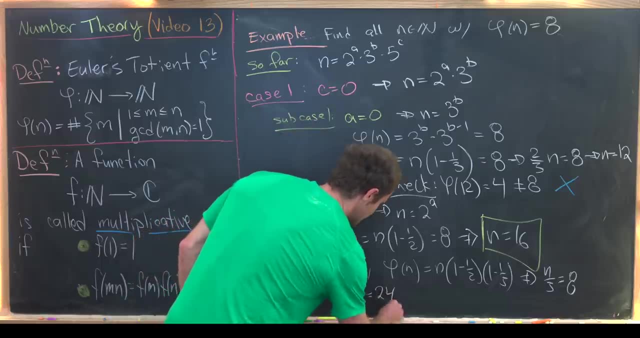 Well, you might say. well, why that? Well, that's just from standard multiplication of rational numbers there. But if n over 3 is equal to 8, that tells us that n is equal to 24.. But notice, 24 is: 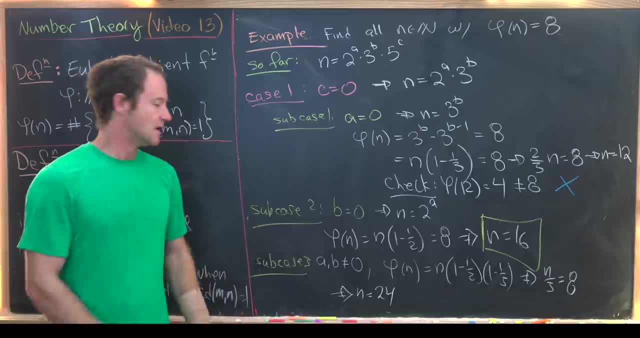 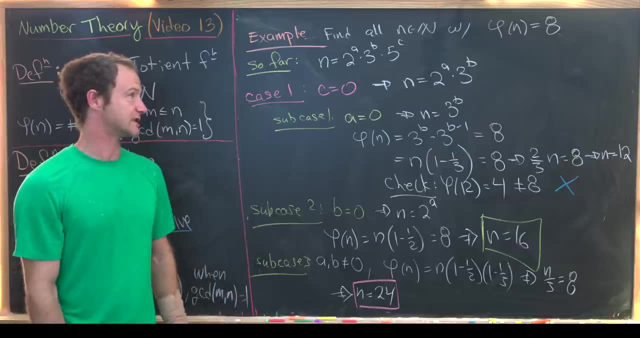 most definitely of the form, 2 to the a, 3 to the b, But you can also just run it through and see that phi of 24 is also equal to 8, which was our goal. Okay, so let's maybe summarize what we have. 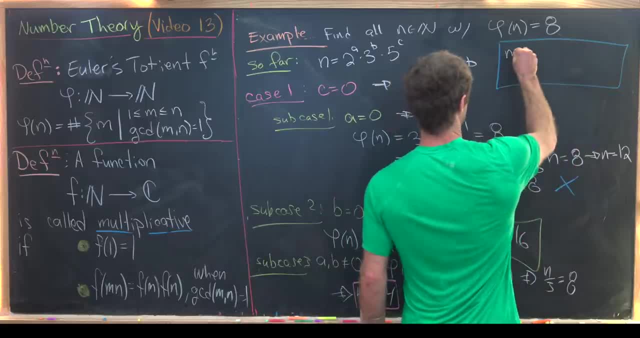 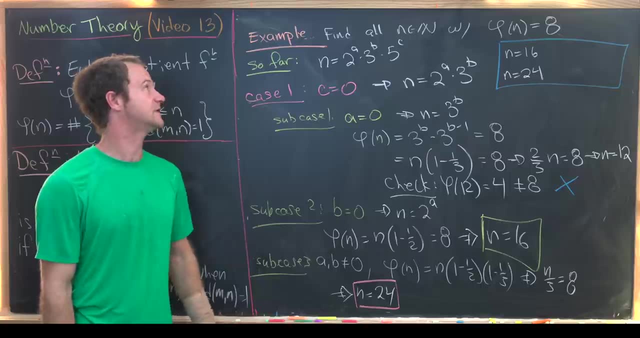 so far up here. So we see that n equals 16 works and n equals 24 also works, And I think that's maybe enough to do on this example. Maybe I'll leave as a warm-up to check the other cases. Okay, so I'm going to leave. 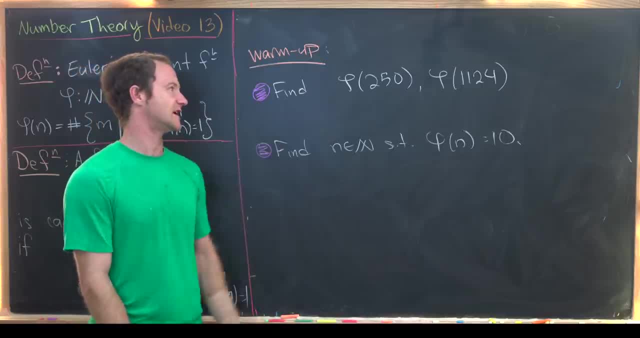 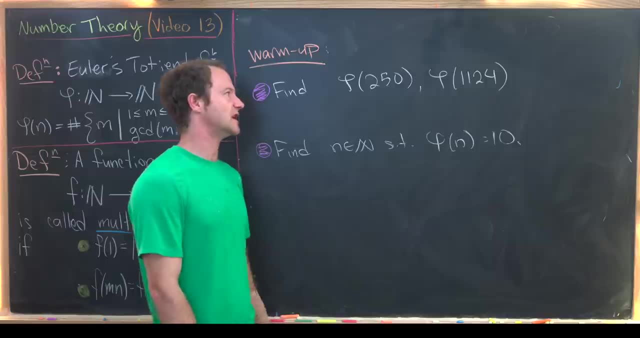 you guys with a couple of warm-up problems. So the first is to find phi evaluated at 250, using the formula that we developed in this video. The second one is to find phi of 1,124, again using the method that we constructed in this video. 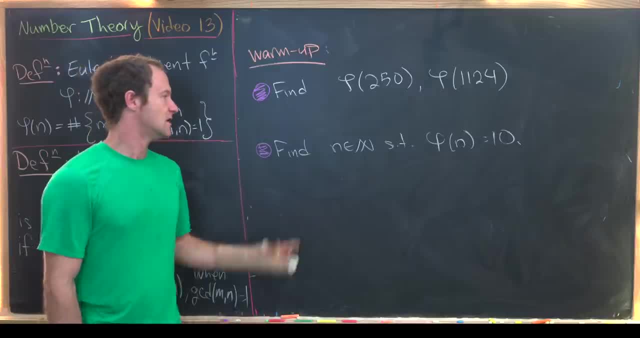 And the next, similar to the example, find all natural numbers, n, such that phi of n is equal to 10. And that's a good place to stop.